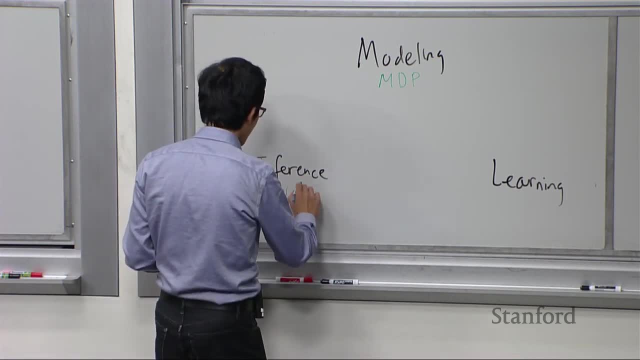 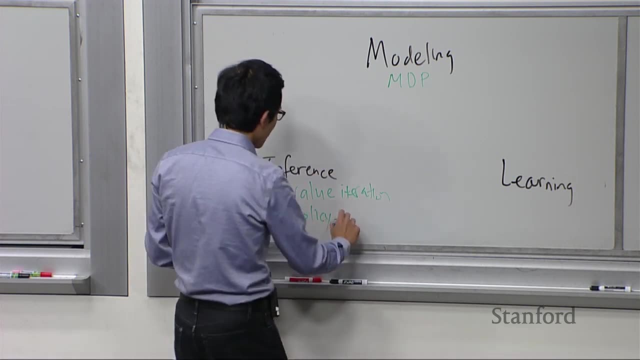 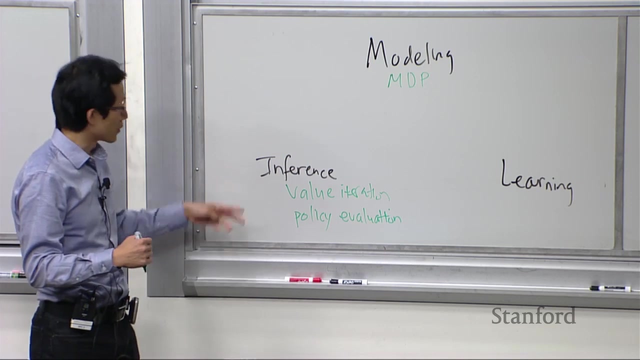 What about inference? So what do we have here? Last time we had value iteration- and which allows you to compute the optimal policy, and policy evaluation, which eval- allows you to estimate the value of a particular policy. So these are algorithms that operate on MDP right. 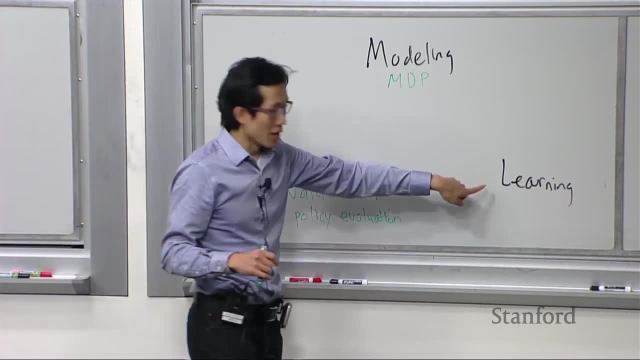 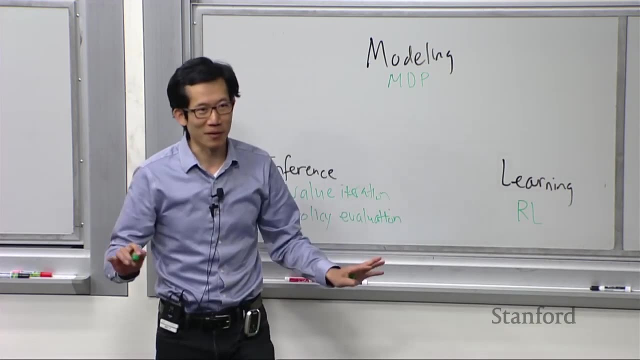 And we looked at these algorithms last time, So this lecture is going to be about learning. I'll just put R out for now. RL is not an algorithm, it's a kind of a- refers to the family of algorithms that fits in this week. 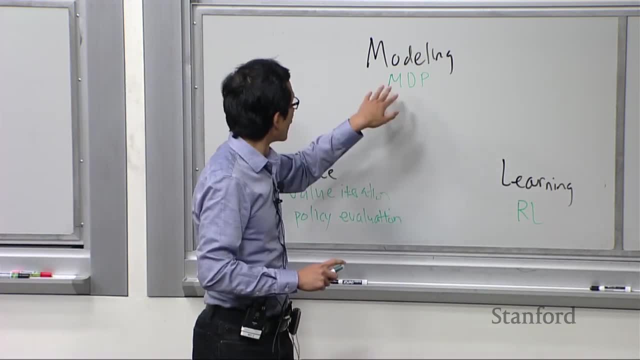 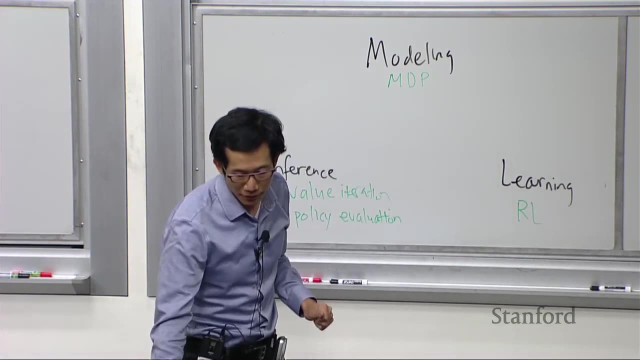 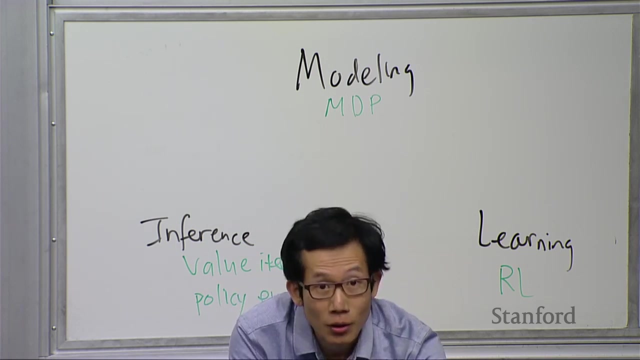 But that's the way you should think about it. RL allows you to either explicitly or implicitly estimate MDPs and then, once you have that, you can do all these inference algorithms to figure out what the optimal policy is. okay, So just to review. so what is an MDP? 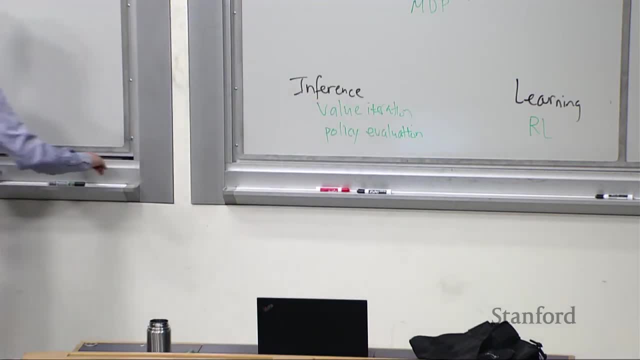 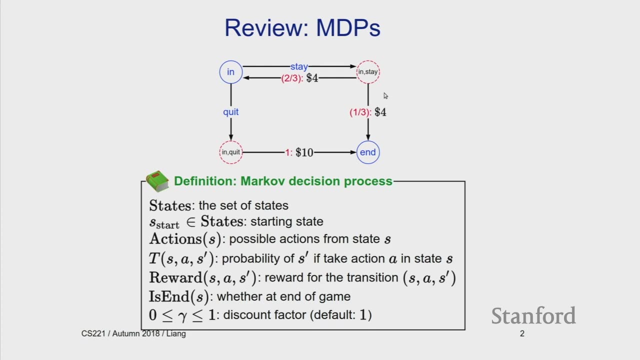 The clearest way remember to think about it is it's in terms of a graph, So you have a set of states. So in this dice game we have in and end, So we have a set of states. From every state you have a set of actions coming out. 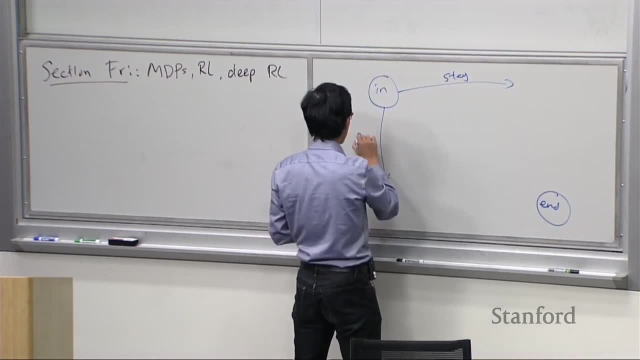 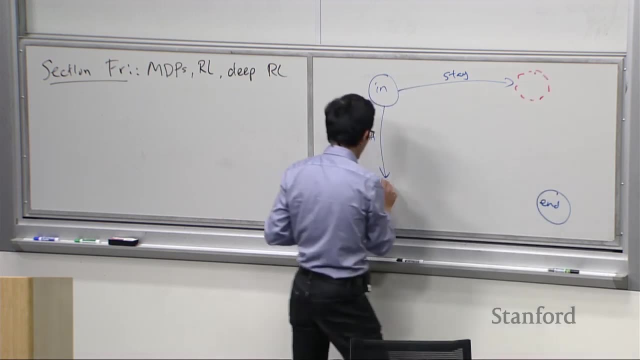 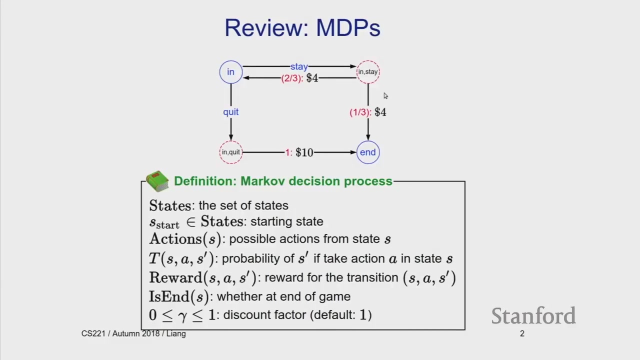 So in this case, stay and quit. The actions take you to chance nodes where the- you don't get to control what happens, but nature does and there's randomness. So out of these chance nodes are transitions. Each transition takes you into a state. 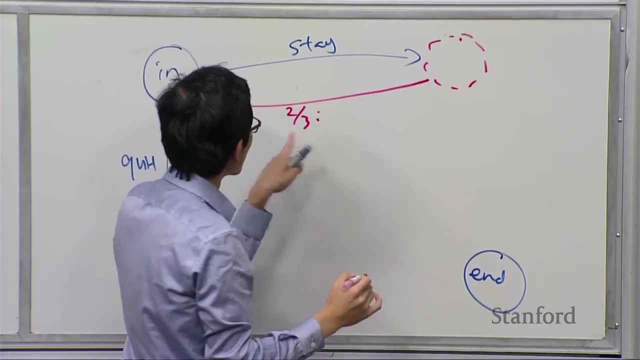 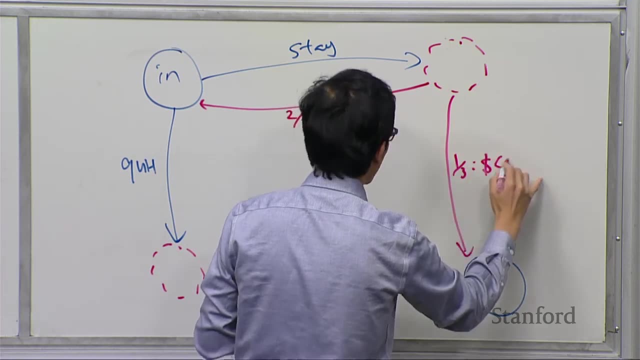 It has some probability associated with it, so two-thirds in this case. It also has some reward associated with it, which you pick up along the way, So naturally this has to be one-third four. And remember, last time this was probability one um ten okay. 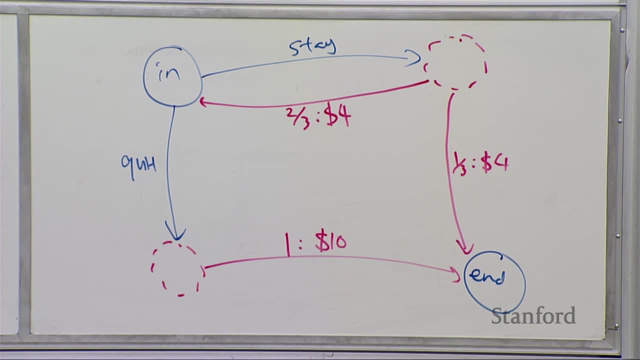 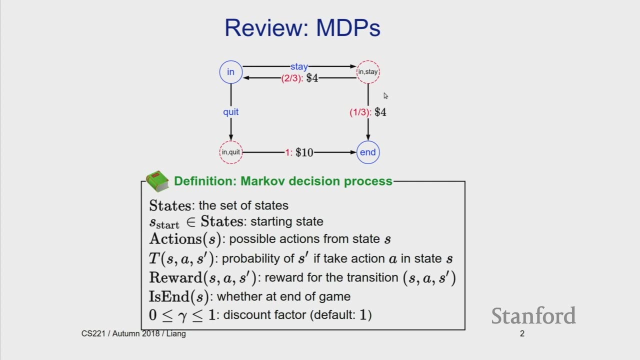 So, um, and then there is, you know, the discount factor, which gamma, which is the number between zero and one, tells you how much you value the future. For default, you can think about it as one. uh, for simplicity. 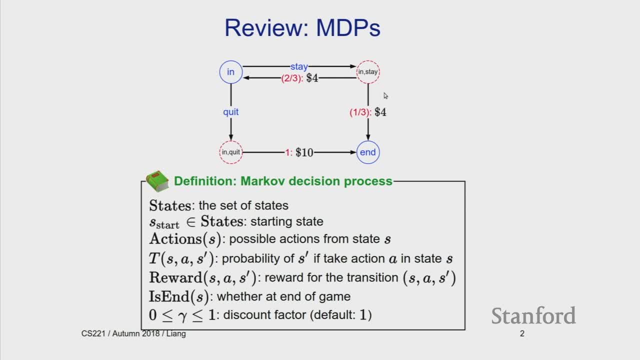 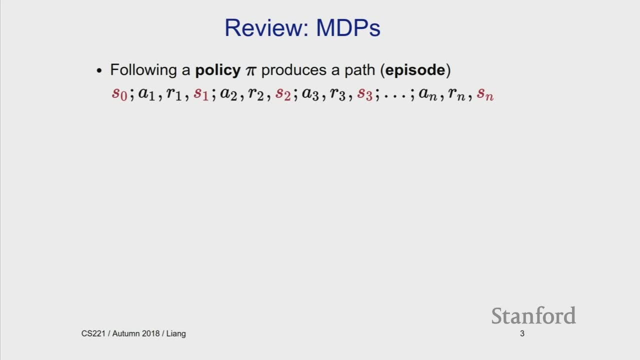 Okay, So this is a Markov decision process. Um, and what do you do with one of these things? We um have a notion of a policy and a policy. um, let's see, I'll write it over here. 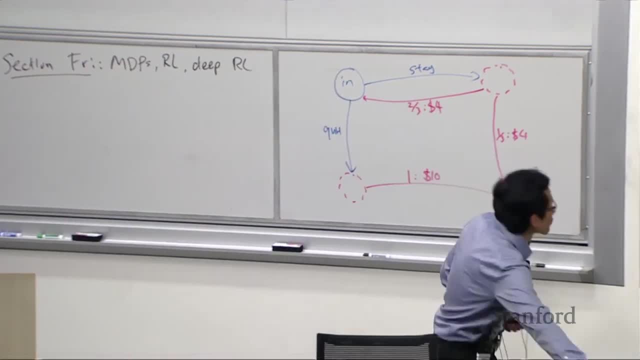 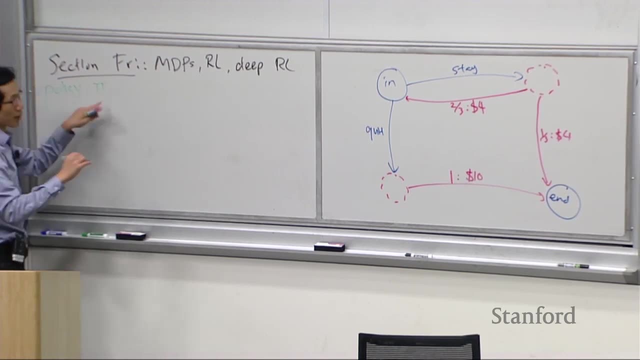 So a policy denoted pi uh- let me use green Um- so a policy pi? um is a mapping from states to action. It tells you a policy when you apply. it says: when I land here, where should I go? 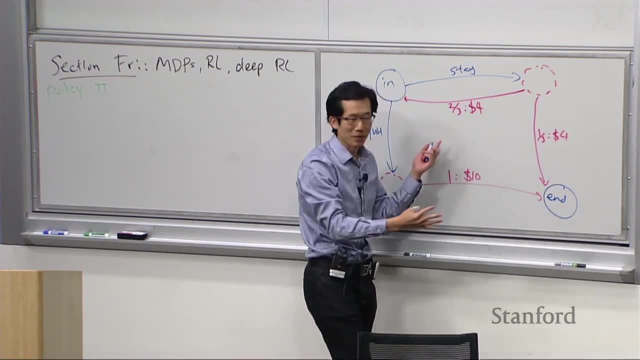 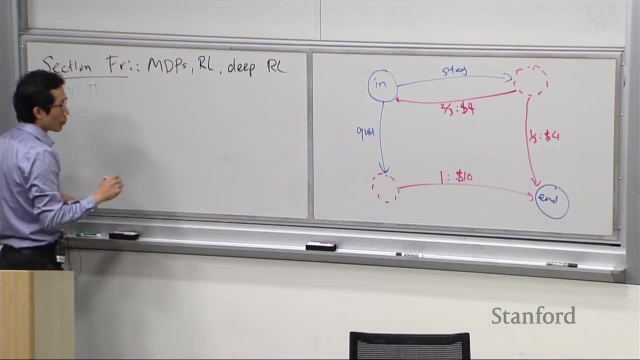 Should I do stay or quit If I land? well, I mean, this is kind of a simple MVP. Otherwise there'd usually be more states and for every state, blue circle will tell you where to go. Um, and when you run a policy, um, what happens? 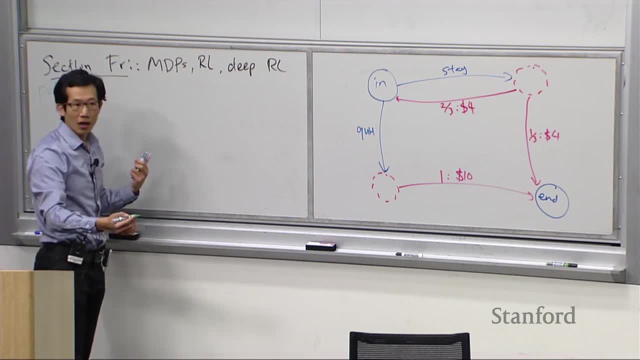 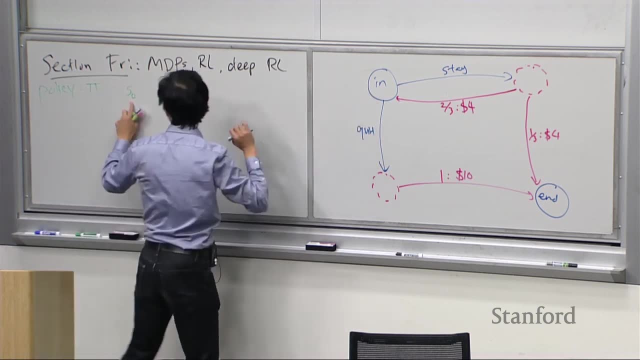 Uh, you get a path um, which I'm going to call an episode. So what do you do? You start in state S0, that's that would be in in this particular example. Um, you take an action A1, let's say, stay. 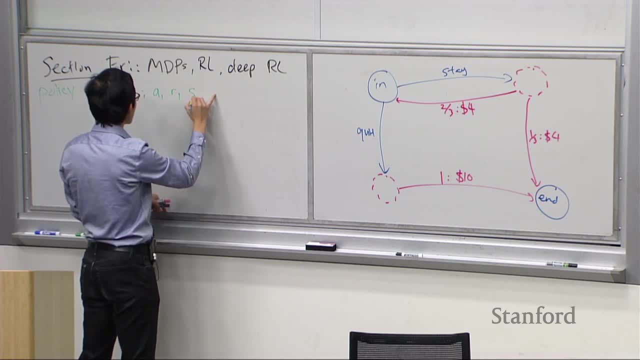 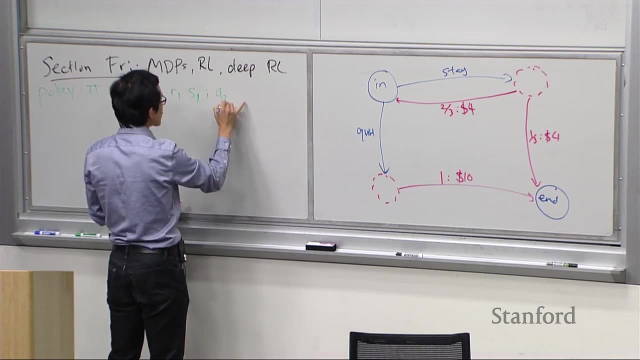 Um, you get some reward. in this case it will be four. You end up in a new state, um, oops, S1, and suppose you go back to in and uh, then you take another action. maybe it's stay. 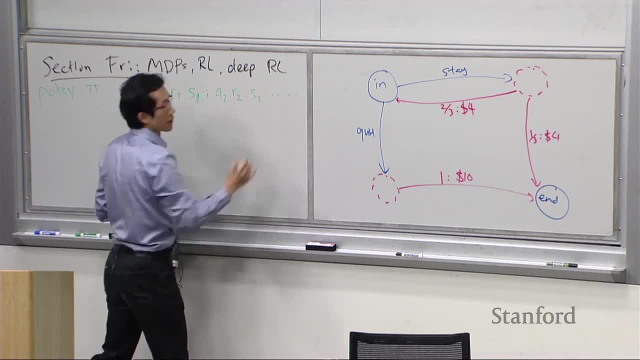 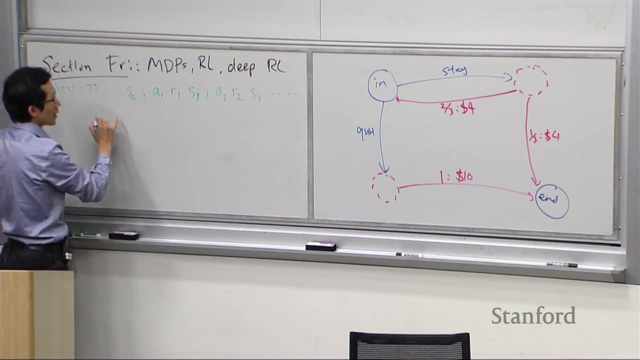 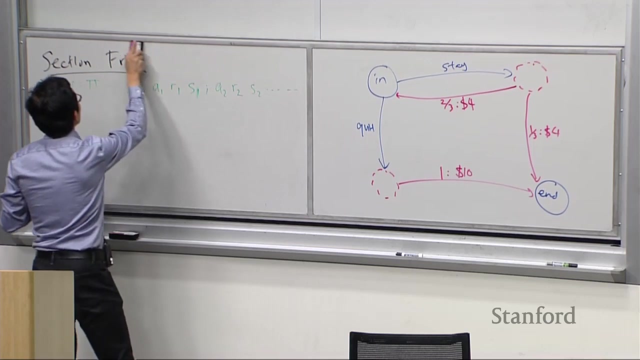 Reward is four, Reward is four again, and and so on. right, So this sequence is a path, or, in RL speak, it's, uh, an episode. um, let's see, So let me, let me erase this comment. 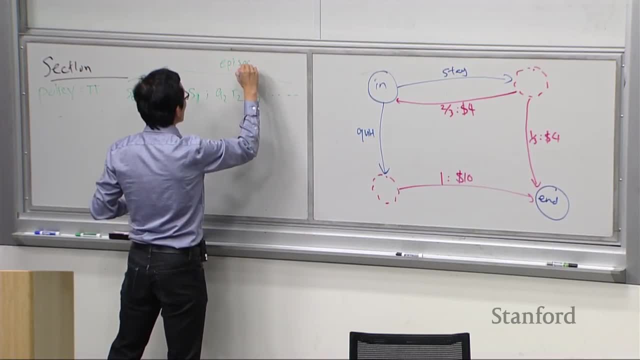 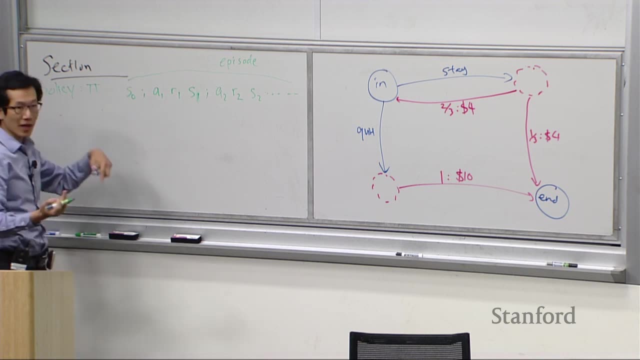 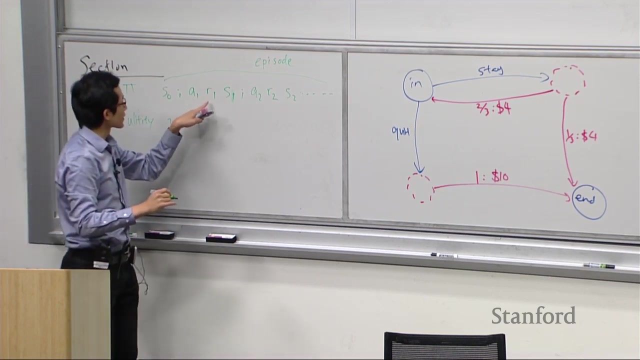 And so this is an episode. um, and until you hit the end state um And uh, what happens out of an episode. you can look at a utility. We're gonna denote u, which is the discounted sum of the rewards along the way, right? 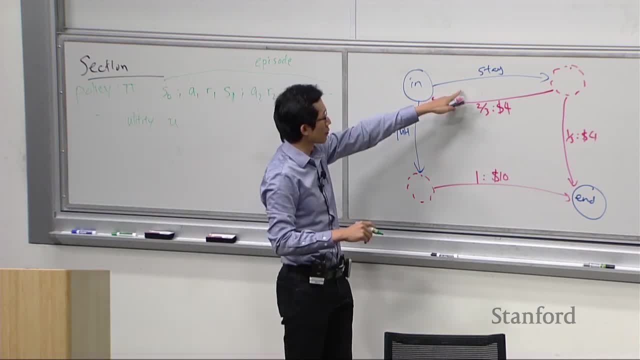 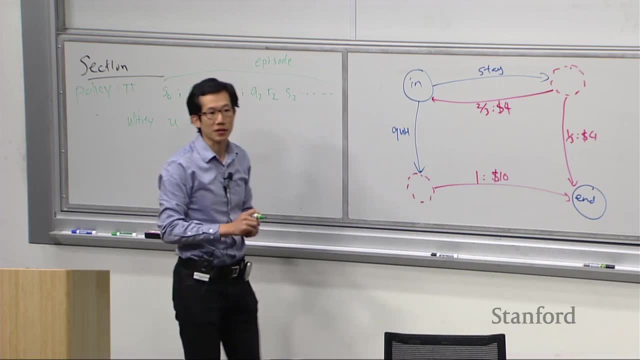 So if you, um, you know, stayed three times and then went there, you would have, uh, uh, utility of four plus four plus four plus four, So that would be 16.. Okay, So by last lecture we didn't really work with. 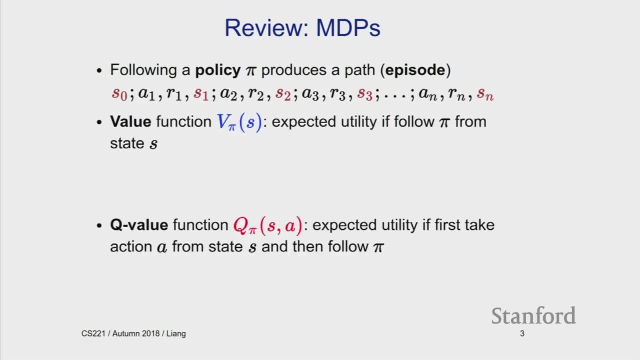 um the episodes in the utility, um, because we were able to define set of recurrences that uh, computed the expected utility. So, um, remember that we want to. you know, we don't know what's gonna happen. 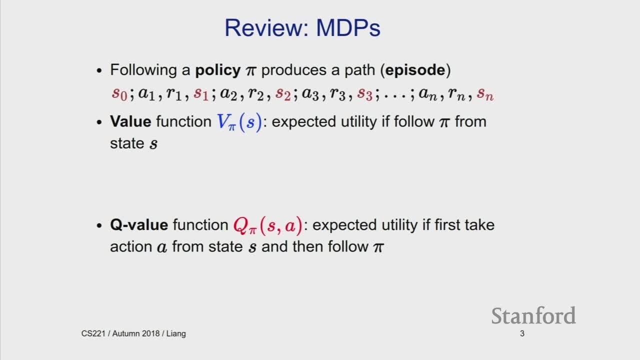 So, uh, there's a distribution, and in order to optimize something, we have to turn it to a number. That's what expectation does Um. so there's two uh concepts that we had from last time. One is the value function of a particular policy. 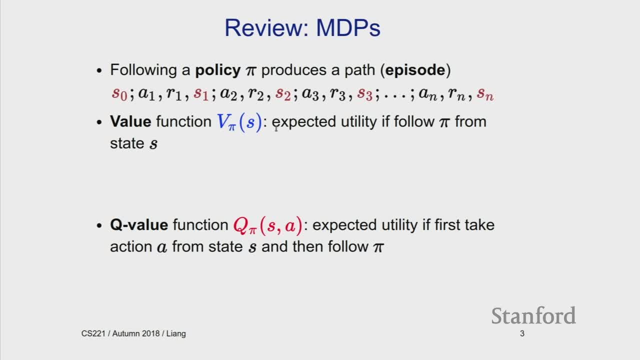 So v pi of s is the expected utility if you follow pi from s. What does that mean? That means if you take a particular s, let's take uh n, and I put you there and you run the policy, so stay and you traverse this graph. 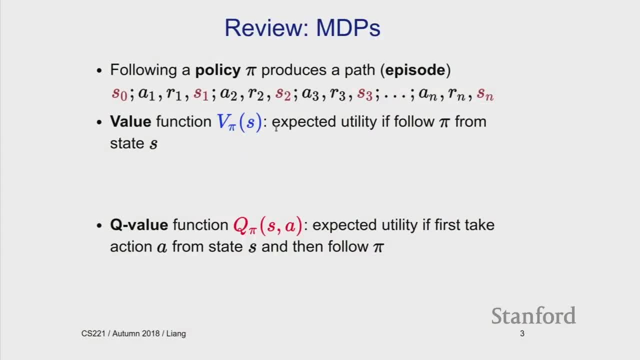 um, you will have different utilities coming out and the average of those is going to be v pi of s. Similarly, there's a q value um expected utility if you first take an action from state s and then follow pi. So what does that mean? 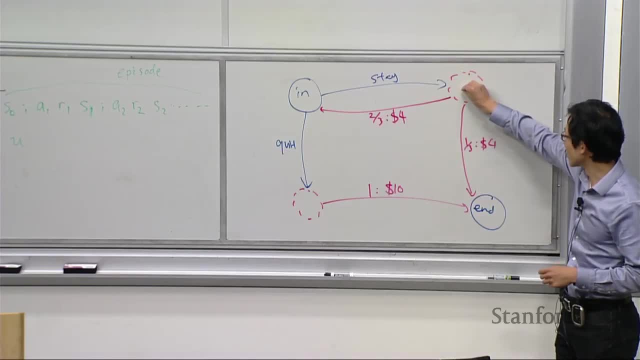 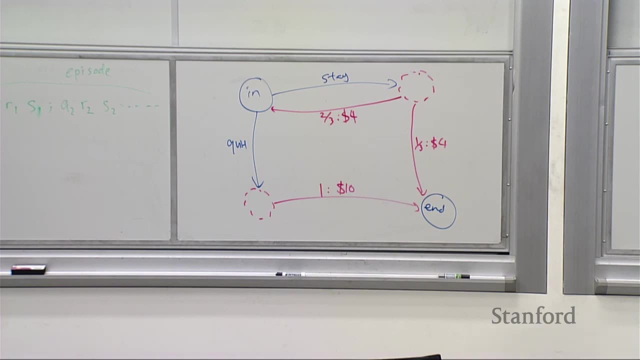 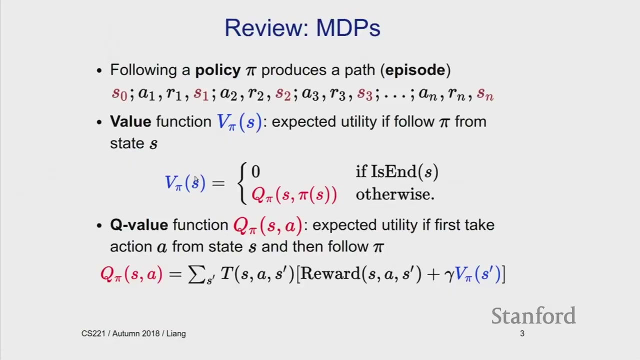 That means, if I put you on one of these, uh, red chance nodes and you basically play out the game um and average the resulting utilities that you get, what number do you get? Okay, Um, and we saw recurrences that related these two. 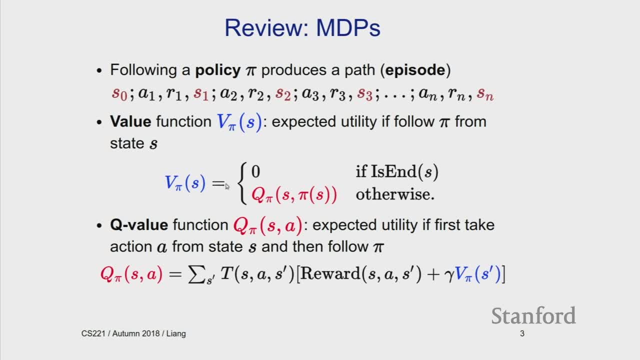 So v pi of s is um you recurrence. the name of the game is to kind of delegate to some kind of simpler problem. So you first uh look up what you're supposed to do in s. that's pi s. 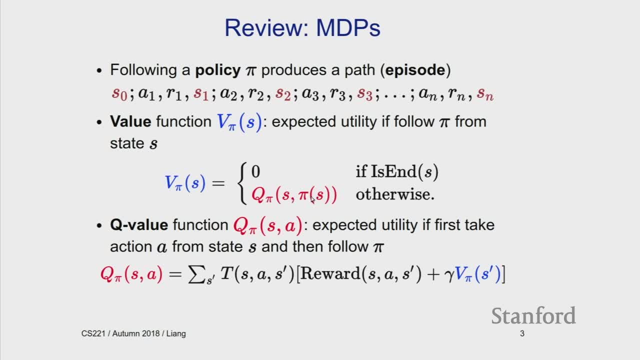 and that takes you to a chance node which is uh s comma pi Pi of sub s. and then you say, hey, how much um utility am I gonna get from that node And similarly from the, the chance nodes. you have to look at all the possible successors. 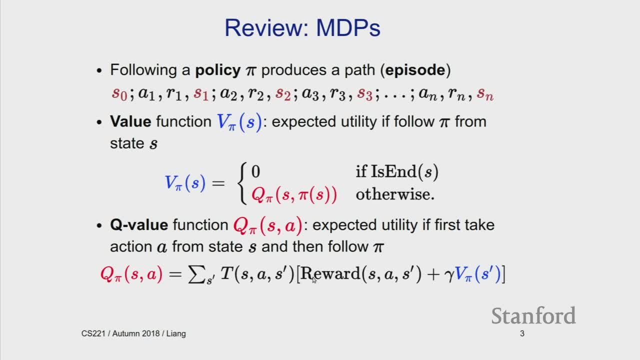 the probability of going into that successor, um, of the immediate reward that you get along the edge, plus the discounted um reward of the uh kind of the future when you end up in um s prime. Okay, So any questions? 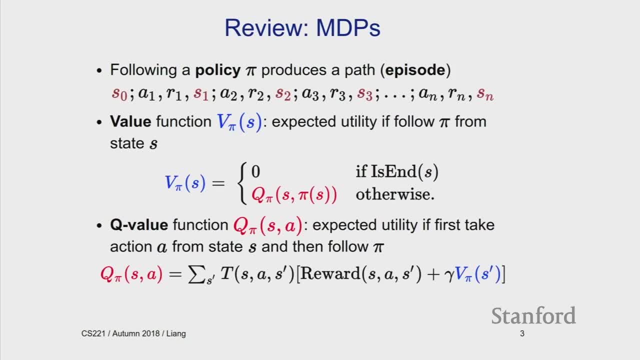 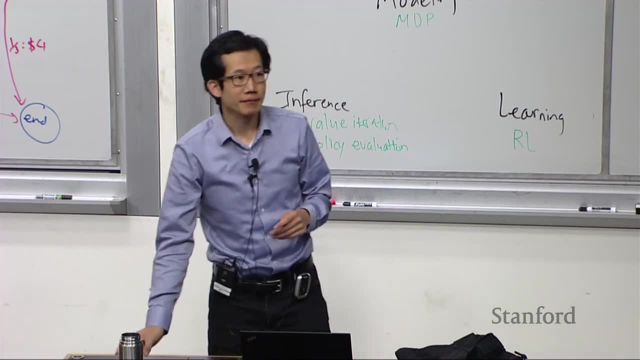 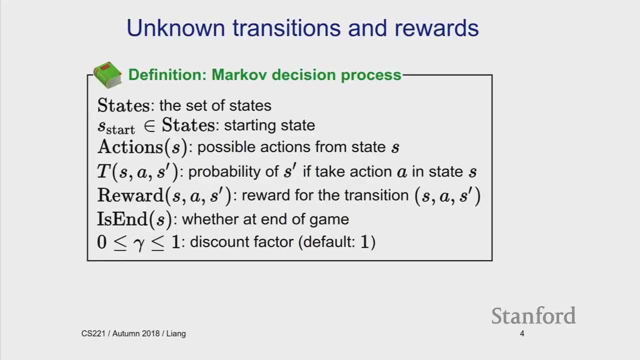 About this. This is a kind of review of uh Markov decision processes from um last time. Okay, So now we're about to do something different. Okay So, um, if you say goodbye to the transition and rewards, 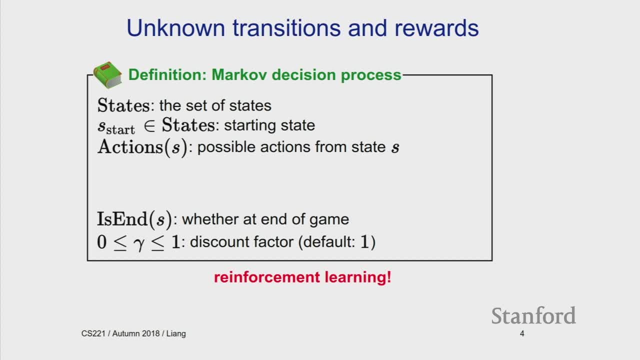 that's called reinforcement learning. So remember Markov: decision processes. I give you everything here and you just have to find the optimal policy. Okay, And now I'm gonna make life difficult by not even telling you um what rewards and what. 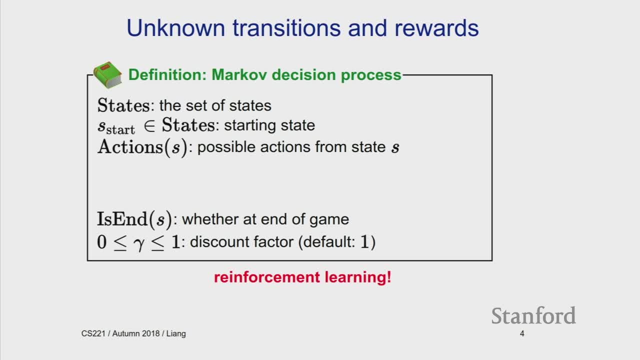 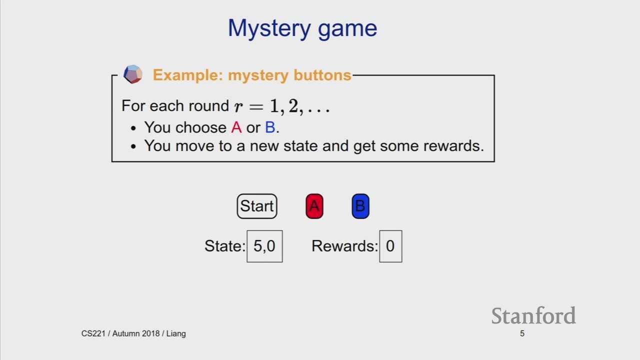 uh, transitions you have to get, Okay. So, just to give a kind of flavor of what that's like, um, let's play a game. So, um, I'm gonna need a volunteer. I'll, I'll give you the game. 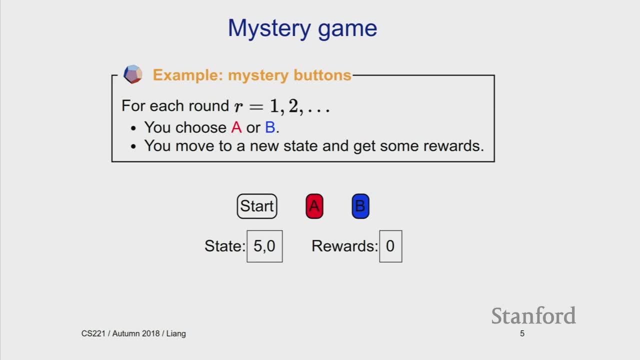 but this volunteer. you have to have a lot of uh grit and uh persistence, because this is not gonna be an easy game. You have to be one of those people that, even though you're losing a lot um, you're still gonna not give up. 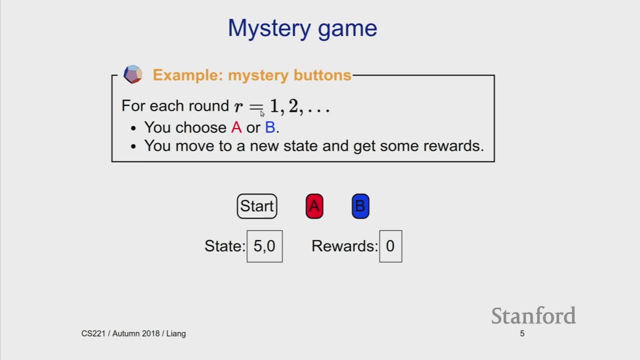 Okay, So here's how the game works. Um so, for each round, R equals uh, 1,, 2,, 3,, 4,, 5,, 6, and so on. You're just gonna choose A or B. 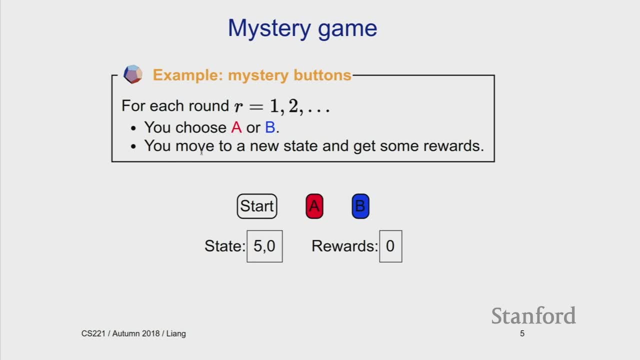 um, red pill or blue pill, I guess. Um, and you, you move to a new state, So the state is here and you get some rewards, which I'm gonna show here. Okay, And the state is 5 comma 0,. 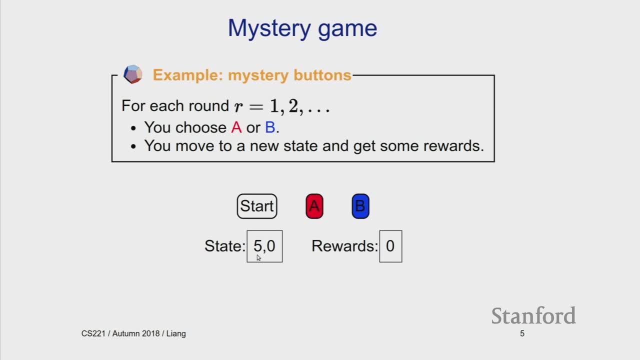 that's the initial state. Okay, So everything clear about the rules. the game, That's reinforcement learning, right? We don't know anything about how- okay, so, uh, any volunteers? Um, how about you in the front? Okay? 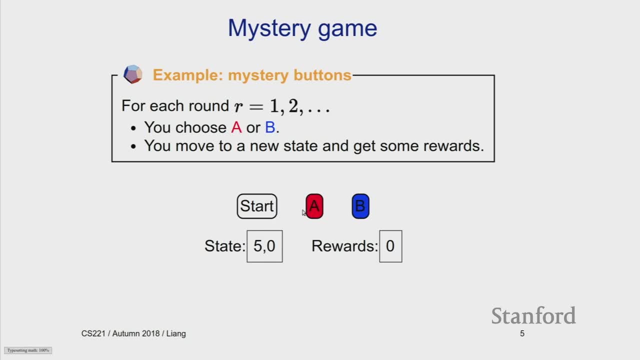 Uh, A A. Okay, Let me, let me click start. A A, A, B, B A. It's an MDP, so, uh, in that case that helps. B, B, B B. 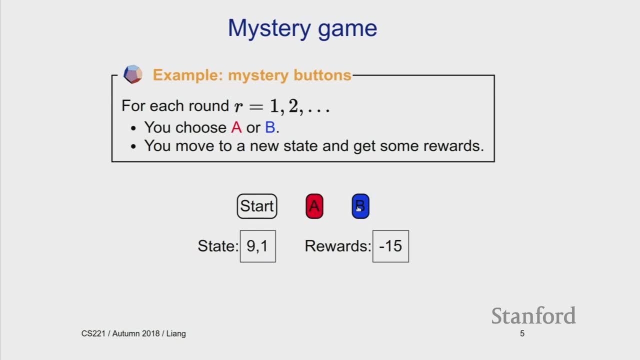 Just infinitely click B, There's an A. I guess I feel like I'm losing points every time. I warned you. Okay, A A, A, B, No, no, no. A, A, A, B, No, no, no. 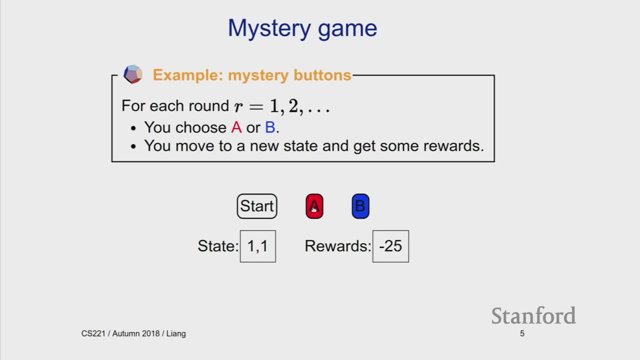 A, A, A, No, no, no. Okay, I'm glad this worked, because last time it took a lot longer, But you know so. so what did you have to do? I mean, you don't know what to try. 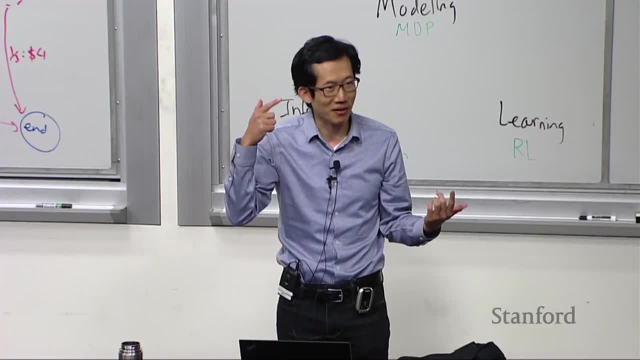 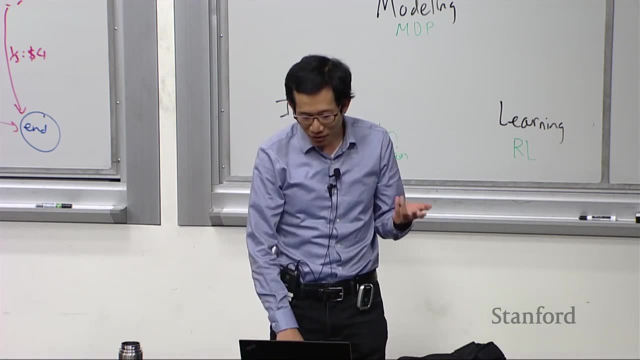 so you try A and B and then hopefully you're building MDP in your, your head, right, Yeah, right, Okay, Just smile and nod And you have to figure out how the game works, right? So maybe you notice that, hey. 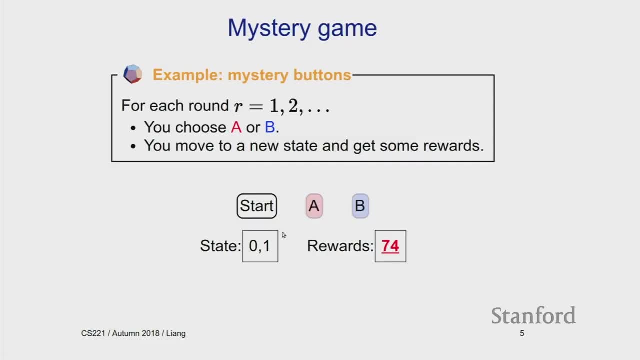 A is, you know, decrementing and B is going up, but then there's this other bit that gets flipped. So, um, can you figure this out? And in the process, you're also trying to maximize reward, which, uh, apparently I guess. 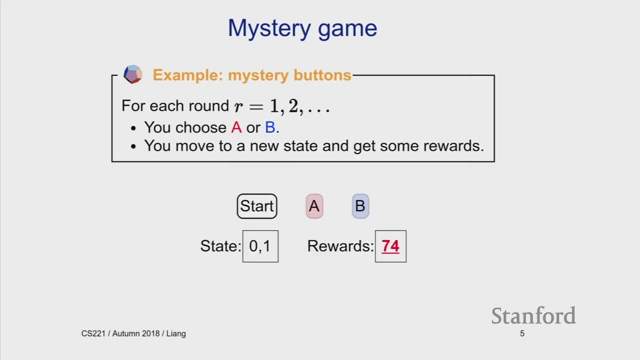 wasn't- doesn't come until the very end because, um, it's a cruel game. Okay, So how do we get an algorithm to kind of do this And how do we think about, uh, pros, um, doing this? 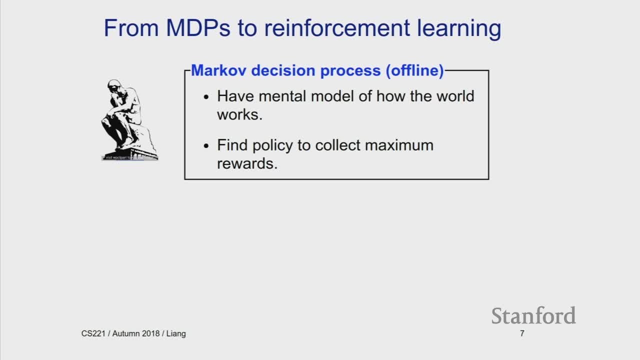 So just to kind of make the contrast between MDPs and reinforcement learning sharper. So, Markov, decision process is an offline thing, right? So you already have a mental model of how the work- world works. That's the MDP, That's all the rewards and the transitions and the states and the actions. 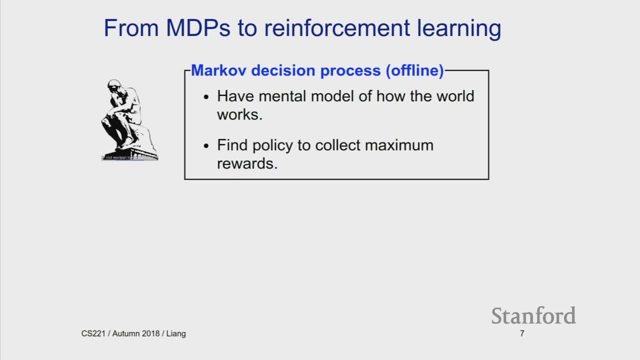 And you have to find a policy to collect maximum rewards. You have it all in your head so you just kind of think really hard about you know what is the best thing is like. oh, if I do this action, then I'll go here and you know. 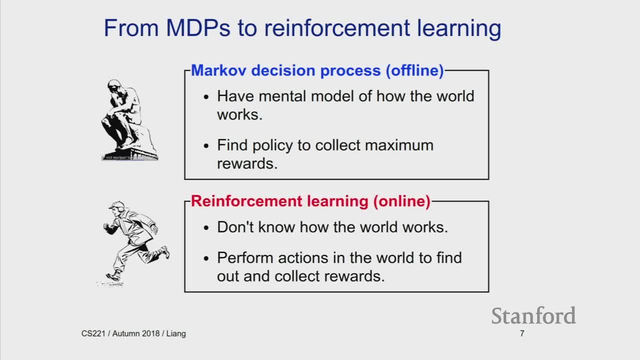 look at the probabilities, take the max or whatever. So reinforcement learning is very different. You don't know how the world works, so you can't just sit there and think, because thinking isn't gonna help you figure out how the world works. Um, so you have to just go out and perform actions in the world, right? 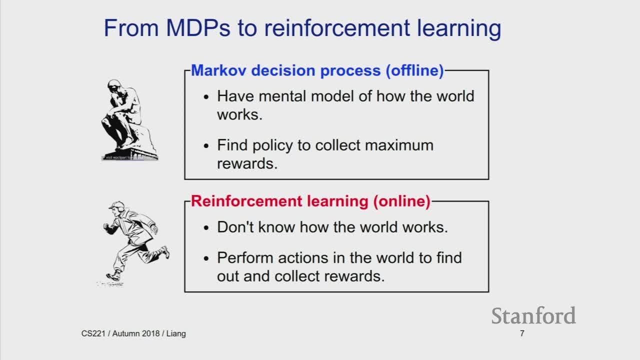 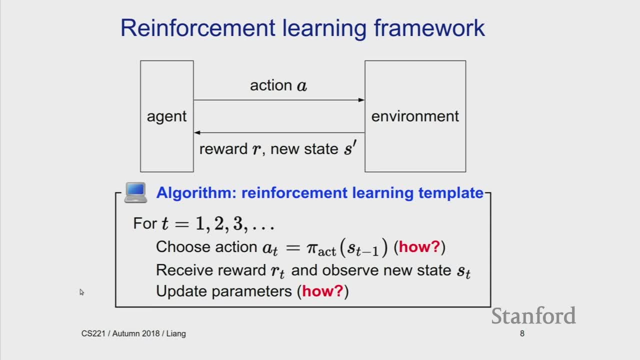 And in doing so you hopefully you'll learn something, but also you're um, you'll get some rewards. Okay, So so to maybe formalize the um, the paradigm of RL, So you can think about it as an agent. 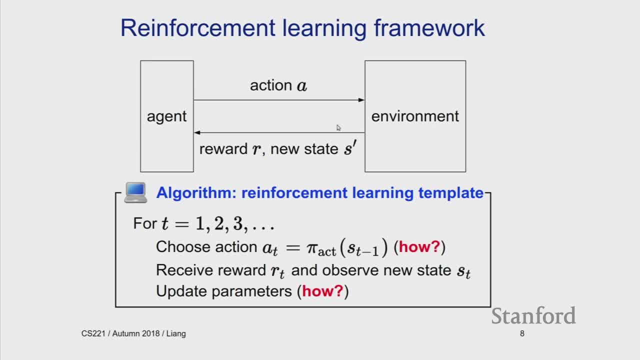 that's uh, that's you um and uh, you have the environment, which is everything else. that's not agent. Uh, the agent takes actions. So the agent sends action to the environment and the environment just sends you back rewards and a new state. 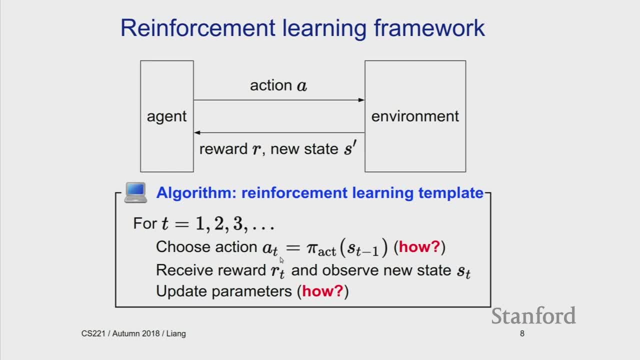 And you keep on doing this. Um, so what you have to do is figure out how. first of all, how am I gonna act If I'm in a particular state, S t minus 1, what action should I choose? Okay, So that's one um, one question. 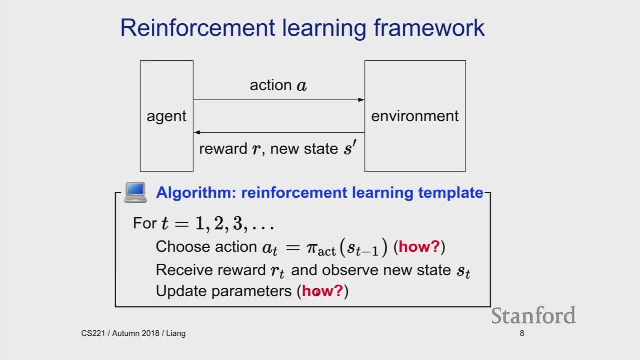 And then you're gonna get this reward and observe a new state. How, what? what should I do to uh, update my mental model of the world? Okay, So these are the main two questions. I'm gonna talk first about how to update the parameters. 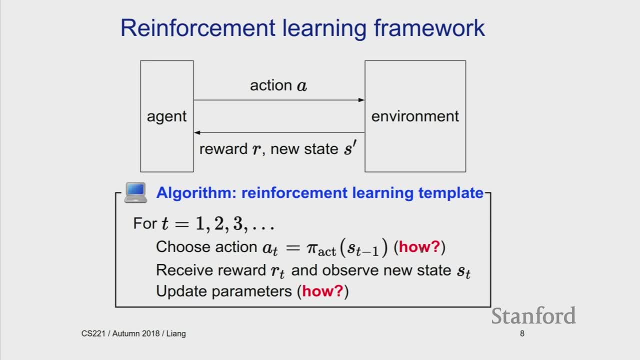 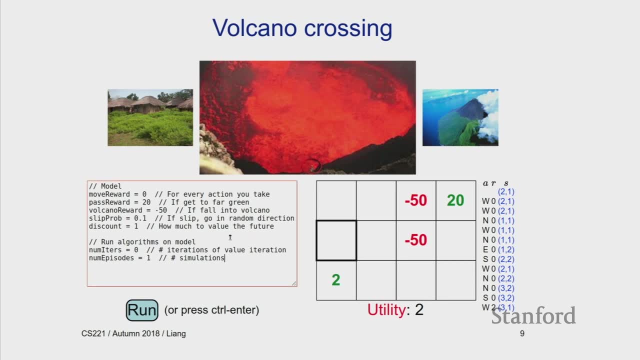 And then later in the lecture I'm gonna come back to how do you actually go and, you know, explore, Okay. So, um, I'm not gonna say much here, but, you know, in the context of volcano crossing, 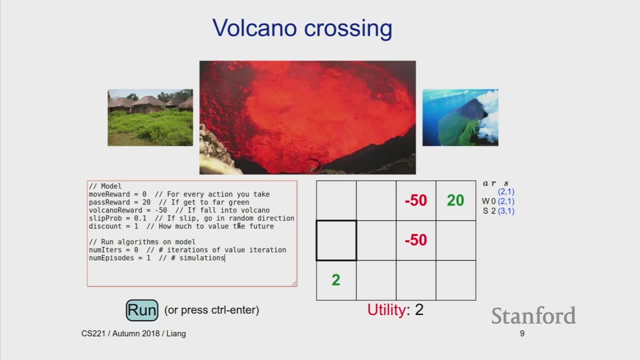 um, just to kind of think through things, every time you play the game right, you're gonna get some utility, So you take a- so this is the episode over here. so A-R-S, You're gonna-. sometimes, you, you know. 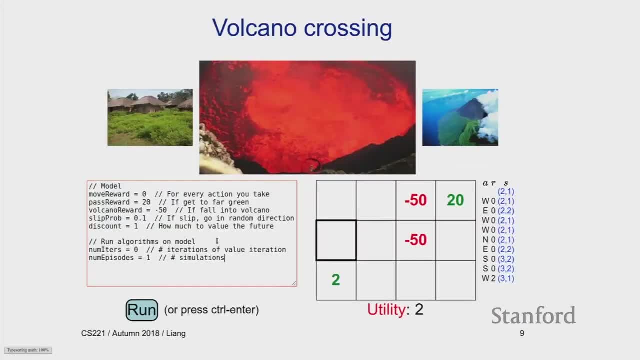 fall into a pit. sometimes you go to a hut, Um, and based on these experiences, um, if I didn't- hadn't told you what any of the actions do and what's the slip probability or anything, how would you kind of go about? 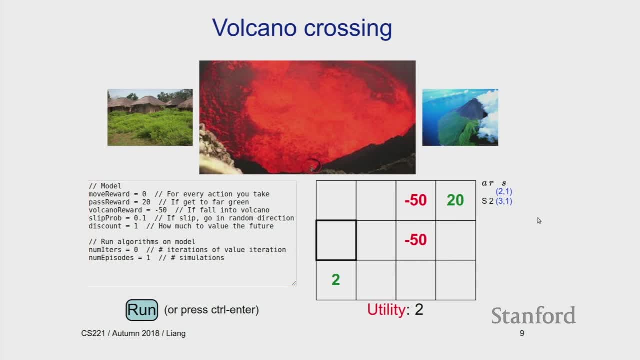 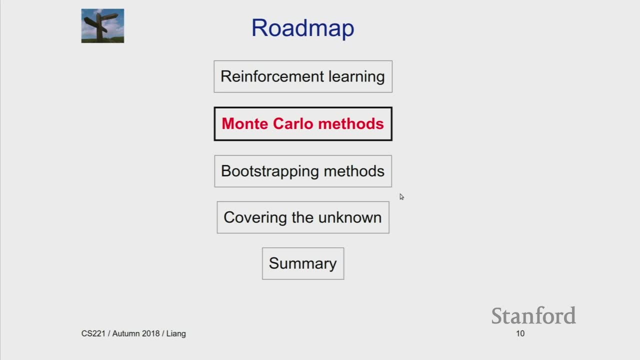 um, just kind of solving this problem. That's the-. that's the question. Okay, So there's a bunch of algorithms. I think there's gonna be one, two, three, four, at least four algorithms that we're gonna talk about, with different characteristics. 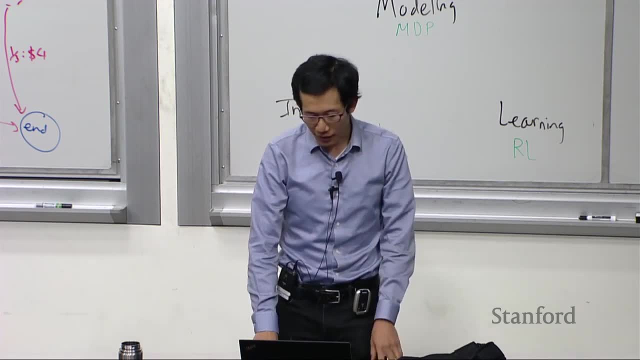 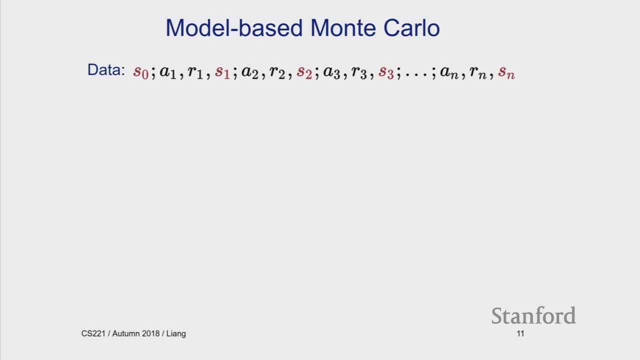 but they're all gonna kind of build onto each other in some way. So first class of algorithm is Monte Carlo methods, right, Um so, um, okay. So when you're- ever you're doing RL or any sort of learning? 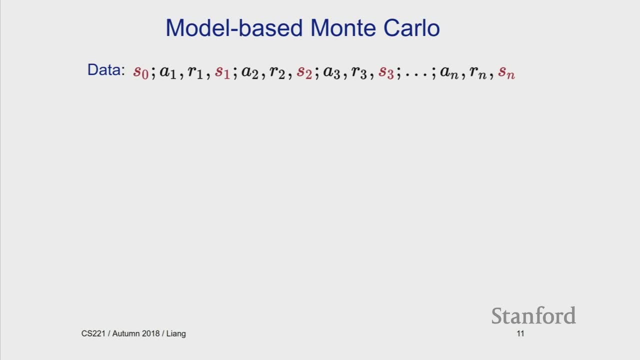 uh, the first thing you get is: you just have data, Let's- let's suppose that you run even a random policies. you're just gonna- because in the beginning you don't know any better. So you're just gonna try random actions and uh, but in the process, 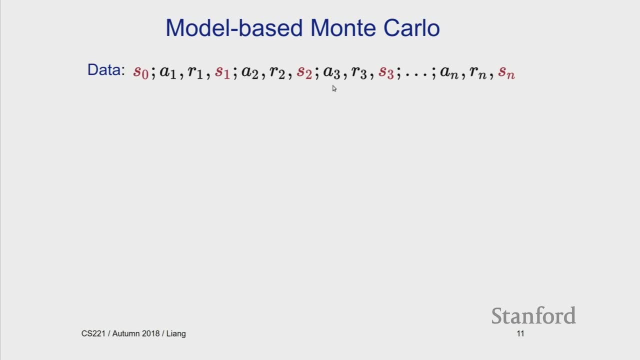 you're gonna see, hey, I tried this action and it led to this reward and and so on. So in a concrete example, just to make uh things a little more crisp, it's gonna look something like in um. 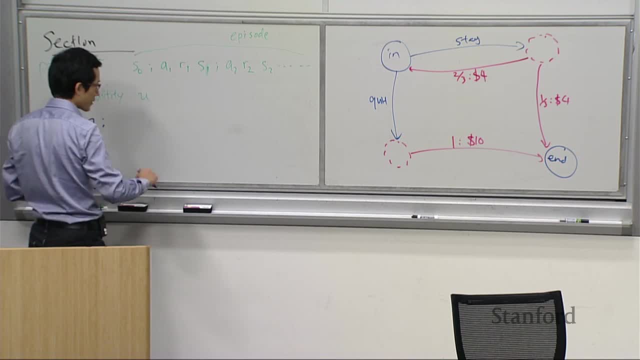 and then you take- uh, you know you did um, let's see, let me try to color coordinate this a little bit- Um, so you're in, in, you do um, stay and you get a reward of four, and then you're back in. 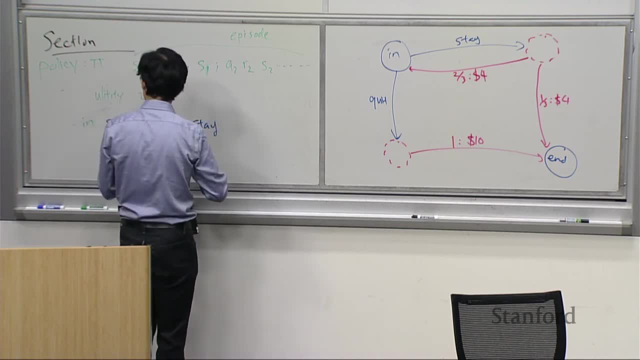 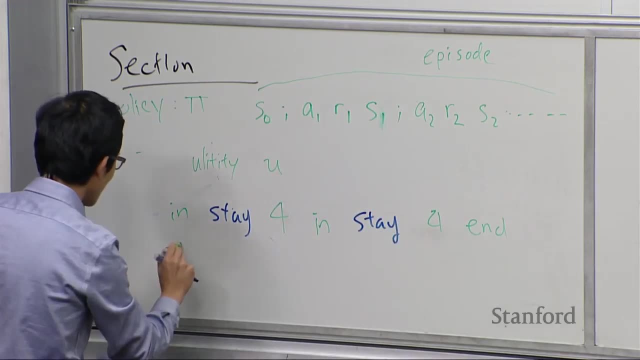 in, you do a stay and then you get four and then maybe you're done, you're out, Okay. So this is uh, an example episode, um, just to make things concrete. So this is S0, A1,, R1,. 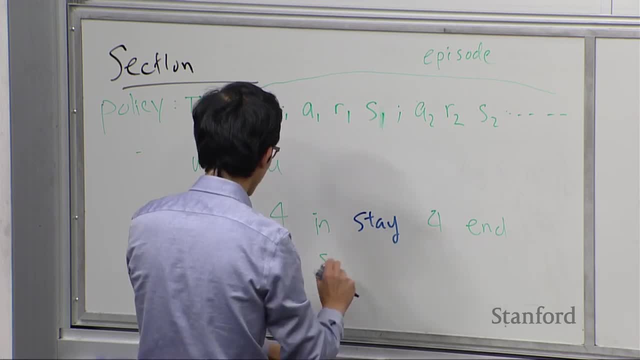 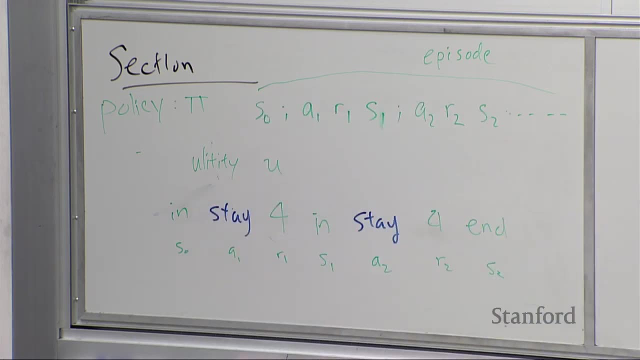 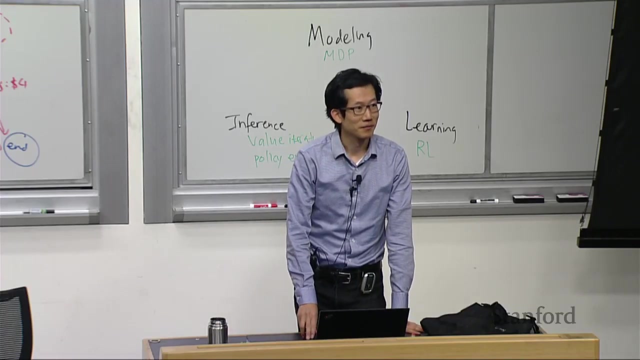 S2, S1, I'm incrementing too quickly um A2, R2, S2, okay, Okay, So what should you do here? All right, So um any ideas, Model-based Monte Carlo. So, if you have the MDP. 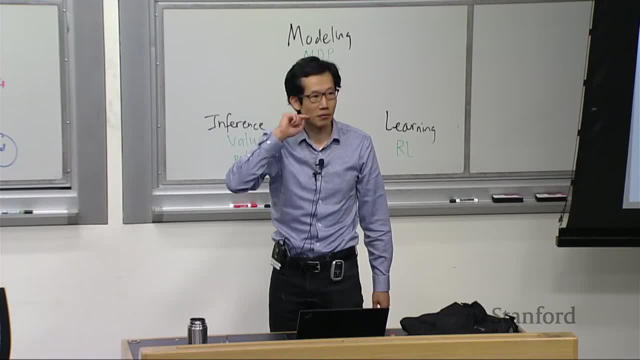 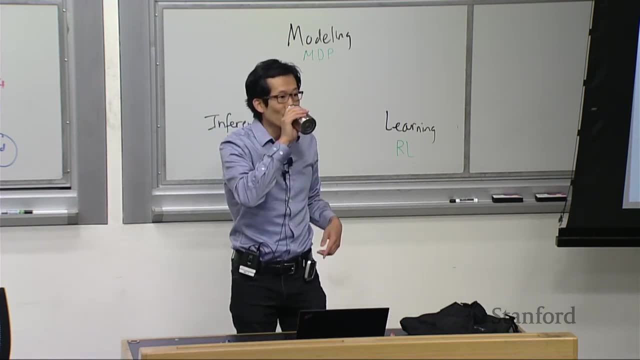 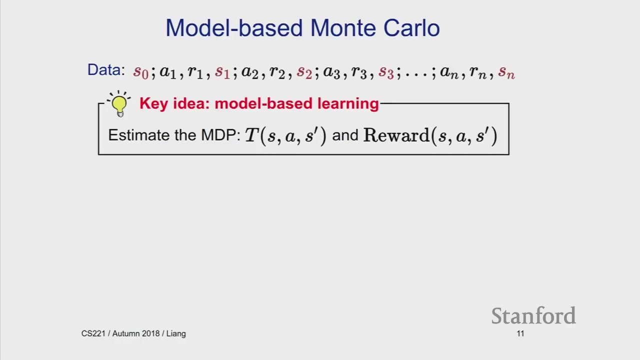 you would be done, But we don't have the MDP, we have data. So what can we do? Yeah, So from that data? Yeah, Let's try to build an MDP from that data. Okay, So, um, as the idea. 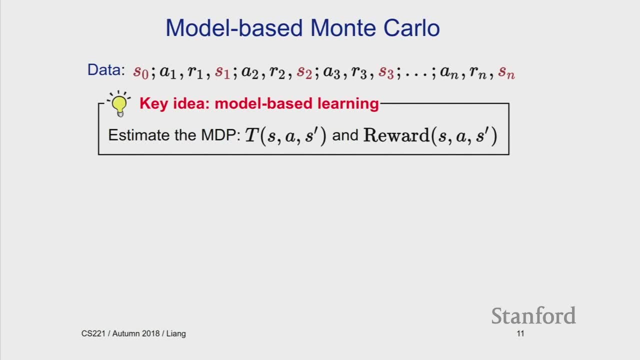 is, uh, estimate the MDP. Um, so intuitively, we just need to figure out what the transitions and rewards are, and then we're done, right. Um, so how do you do the transitions? Um, so the transition says: 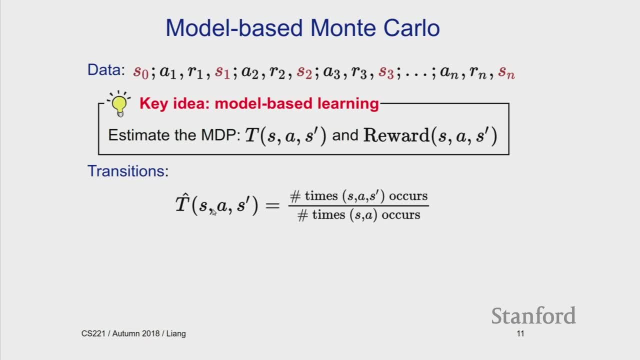 if I'm in state S and I take action A, what will happen? I don't know what will happen, but let's see in the data what happened So I can look at the number of times I went into a particular S prime. 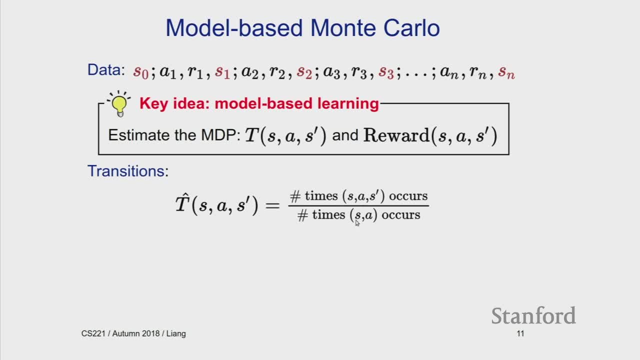 um, and then divide it over the number of times I attempted any of this action from that state at all and just take the ratio okay. And for the rewards, um, this is actually fairly, you know, easy when I- because when I observe a reward, 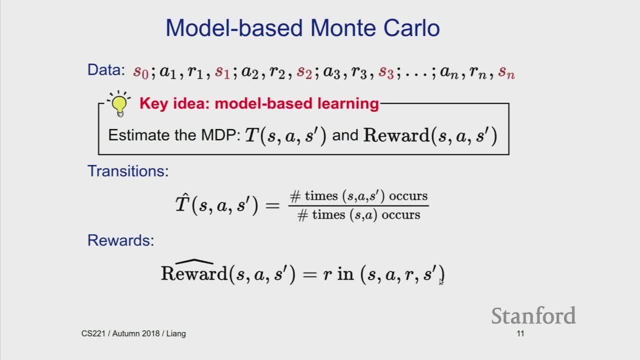 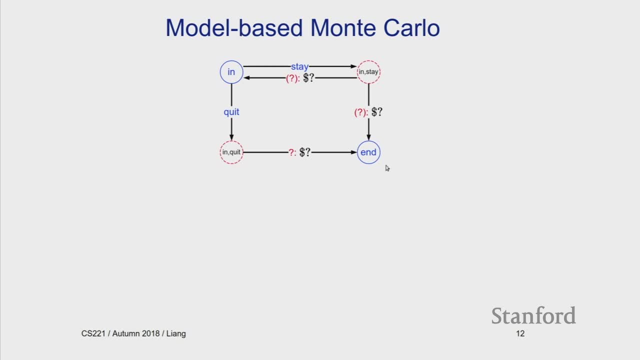 um, from S A and S prime. I just write it down and say: that's the reward, okay, Okay. So, on the concrete example, what does this look like? So remember, now here's the MDP graph. I don't know what the- the uh. 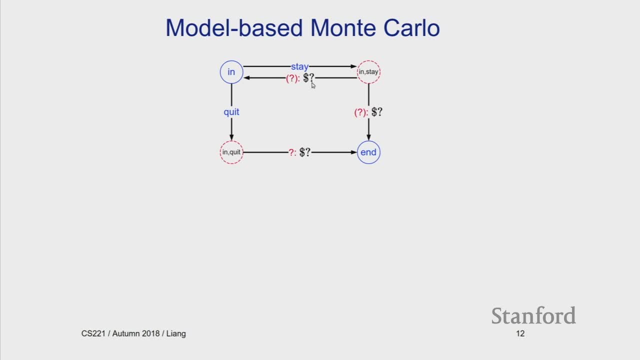 transition, dis- distribution is okay, The distribution or the rewards are Um. so let's suppose I get this trajectory. What should I do? So I get, stay, stay, stay, stay and then I'm out. okay, So first I- I can write down the rewards of four here. 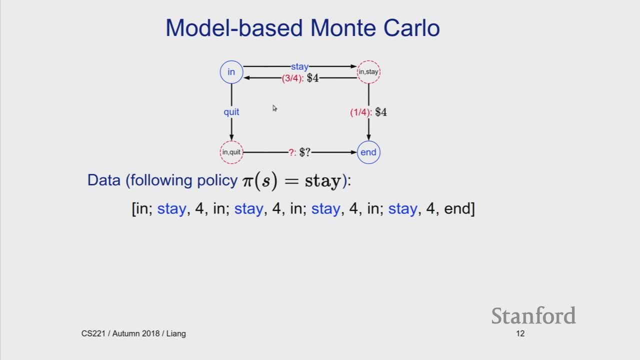 and then I can um estimate the probability of, uh, you know, transitioning. So, three out of four times I went back to N, one out of four times I went to N. so I'm gonna estimate this as three. this is three-fourths, one-fourths, okay. 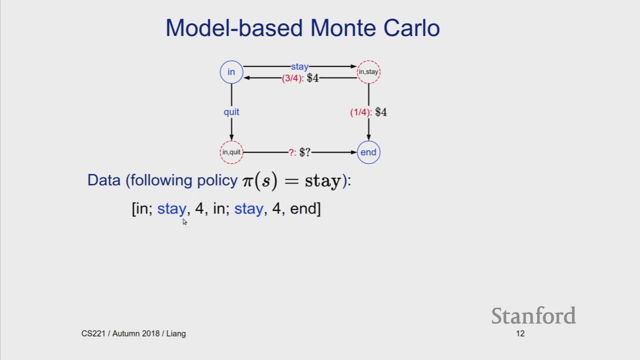 But then, uh suppose I get a new uh uh data point, So I have stay, stay, end. So what do I do? I can add to these counts, um, so everything is kind of cumulative. So two more times- oh sorry. 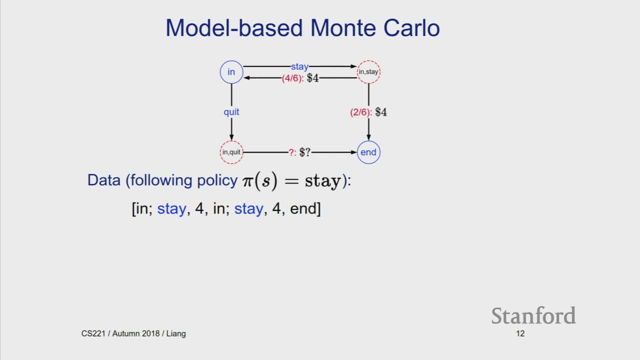 one more time I went into N and another time I went to N, so this becomes four out of six, three out of six, And suppose I see another time when I just go into N. so I'm just gonna increment, uh, this counter, and now it's three out of seven and four out of seven. 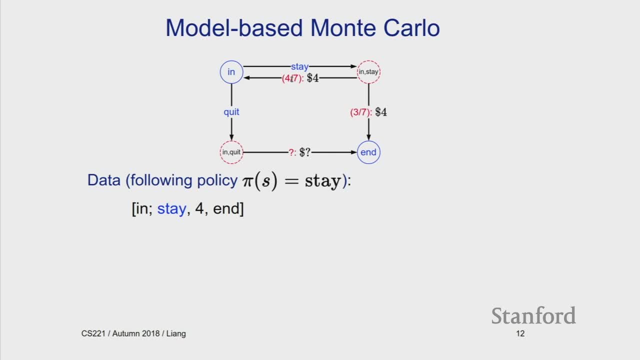 Okay, So pretty, um, pretty simple, Okay. So, for reasons I'm not gonna get into, um, this process actually, you know, converges to the- if you do this kind of, uh, you know, a million times, 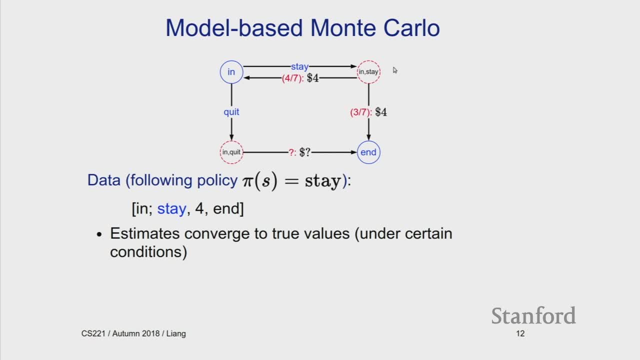 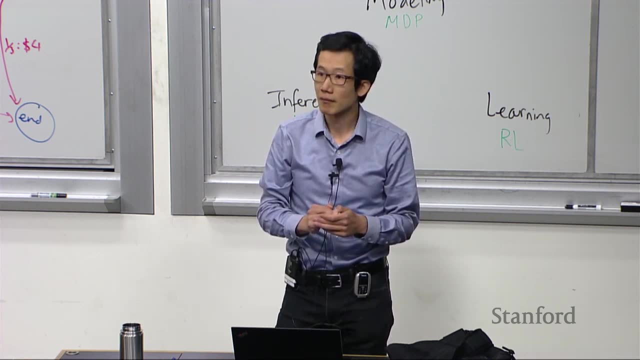 you'll get pretty, um, accurate, Um, yeah, question: Are we saying here that we don't know the transition of probabilities and the reward, but do we know the number of states and the actions we can take? Yeah, So the question is: you don't know the rewards or the transitions, um, but yeah. 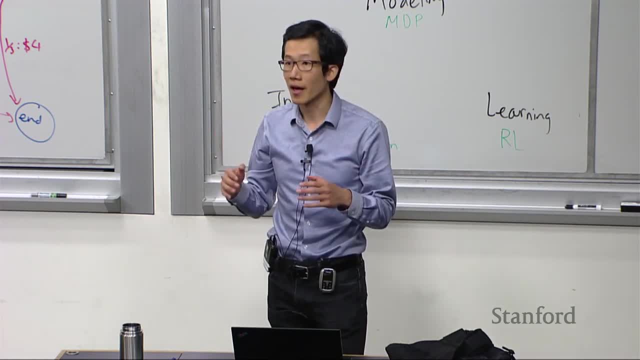 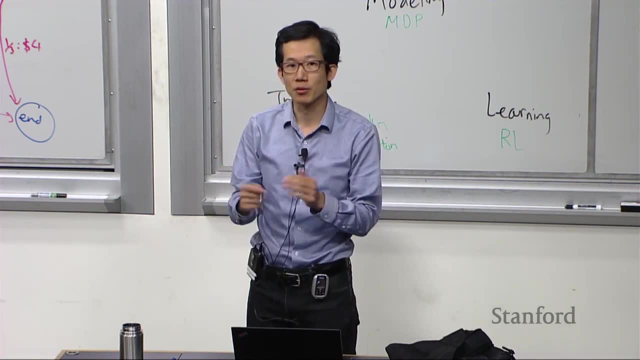 so you do know the set of uh states and the actions Set of states. I guess you don't have to know them all in advance, but you will just observe them as they come. The actions you need to know because you are an agent and you need to play the game. 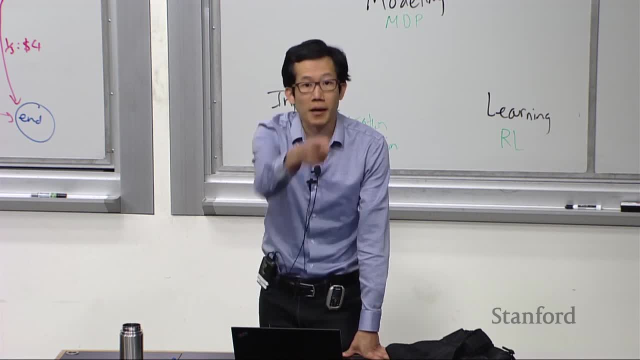 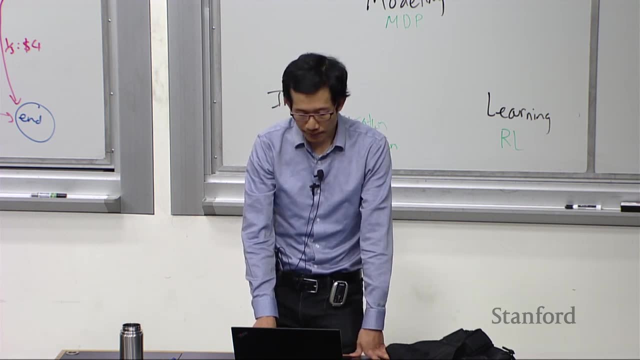 Yeah, Good question, Okay. So yeah, Does this work with variable costs, like there's a probability- or variable rewards? rather, There's a certain probability you get some rewards, certain probability you get a different reward. Yeah, So the question is: 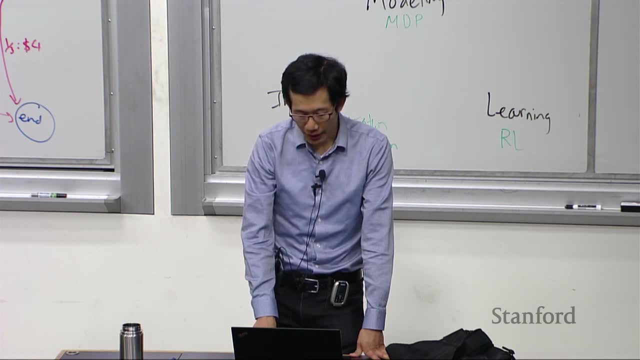 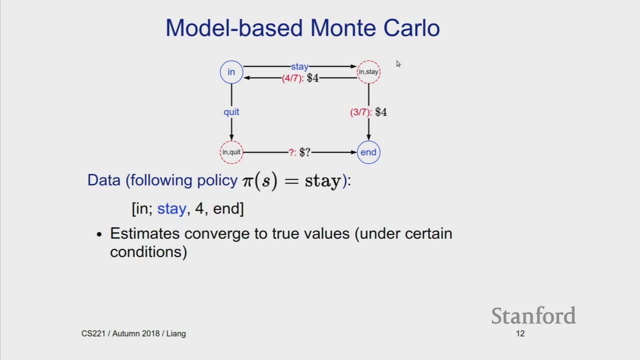 does this work with variable, uh rewards, Um, and if the reward is not a function of um, the S-A-S prime, um, you would just take the average of the rewards that you see. Yeah, Okay, So so what do you do with this? 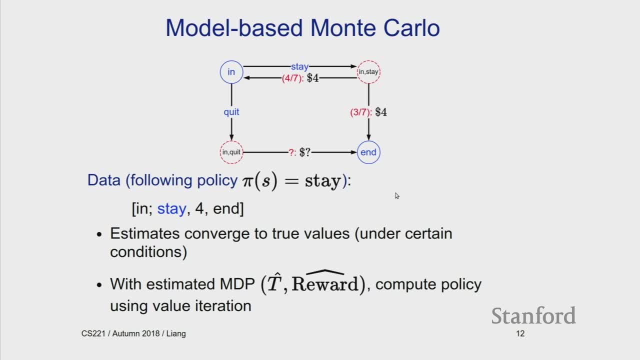 So, after you estimate the MDP, so you- all you need is the transitions and rewards. um then, now we have MDP, It might- it might not be the exact right MDP, because this is estimated from data, so it's not gonna match it exactly. 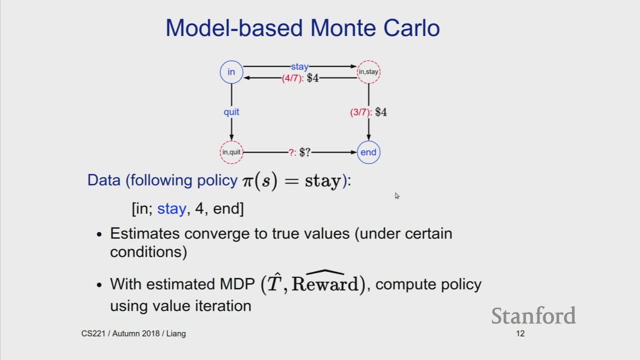 Um, but nonetheless we already have these tools from last time. You can do value iteration to compute um the optimal policy on it, and then you, just you know you're done, you run it, Um. in practice you are probably kind of interleave the learning and the. 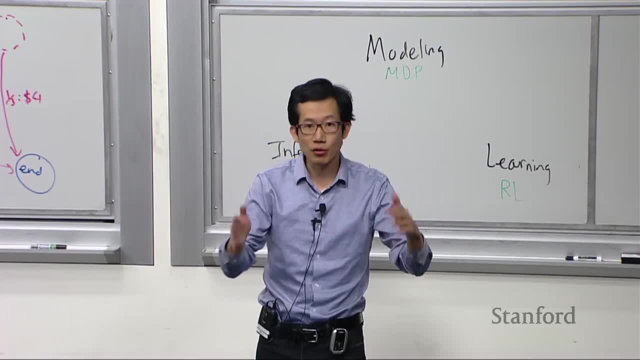 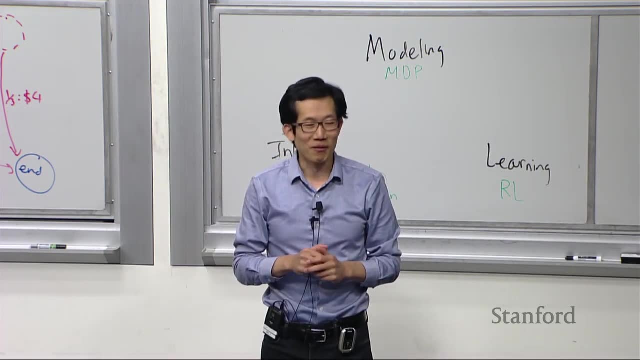 the optimization. but, um, for simplicity, we can think about it as a two-stage, where you gather a bunch of data, you estimate the MDP and then you are off. Okay, There's one problem here. Does anyone know what the problem might be? 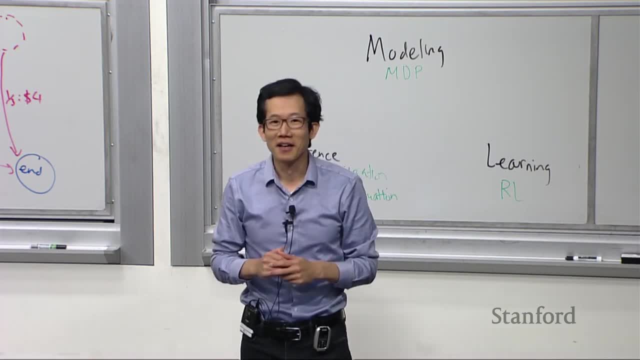 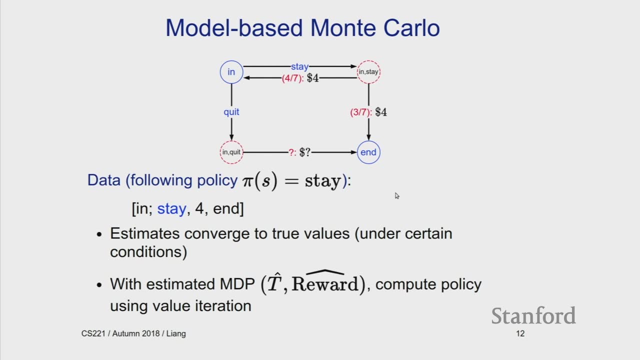 You can actually see it by looking on the slide. Yeah Well, with your base policy of always staying on leverage for the quick branch of the world, Yeah Yeah, You didn't explore this at all, So you actually don't know how much reward is here. 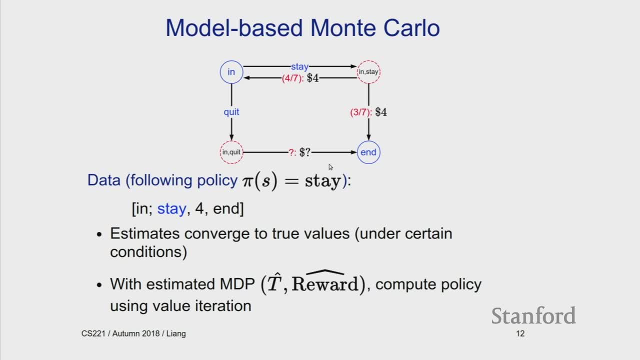 Maybe it's like: uh, you know 100, right? So so this is this- this problem, this kind of actually a pretty big problem that, unless you have a policy that, um, actually goes and covers all the the states, you just won't know, right. 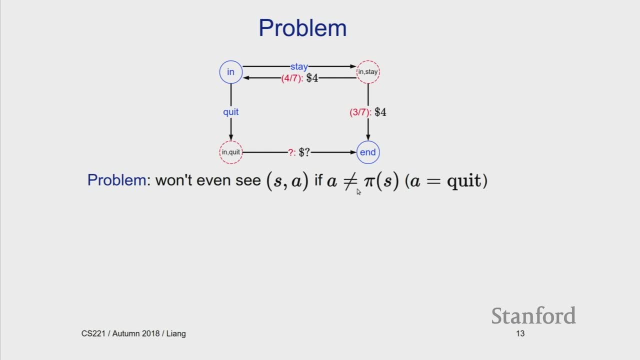 And this is kind of natural, because there could always be, you know, a lot of reward hiding under kind of one state. but unless you see it, you, you don't, you just don't know. Um, okay, So this is a kind of key idea. 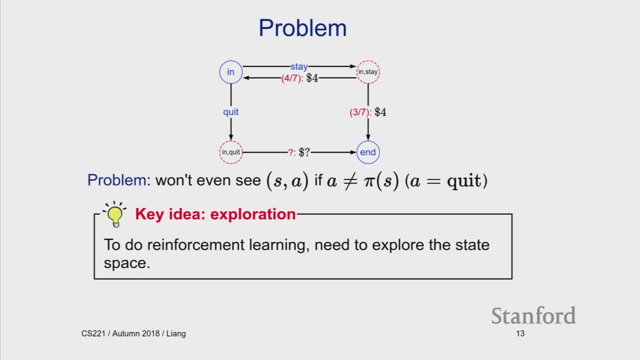 a key challenge I would say in reinforcement learning is exploration. So you need to be able to explore um the state space. This is different from normal machine learning where data just comes in passively and you learn a, you know, a nice function and then you're, you're done. 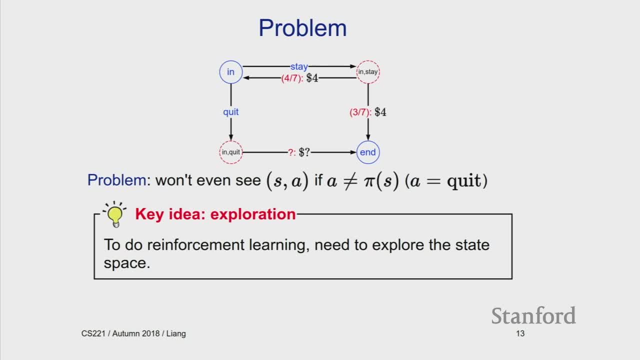 Here you actually have to figure out how to get the data, And that's that's kind of one of the the key challenges of RL. So we're gonna uh go back to this, uh, this problem, and I'm not really gonna. 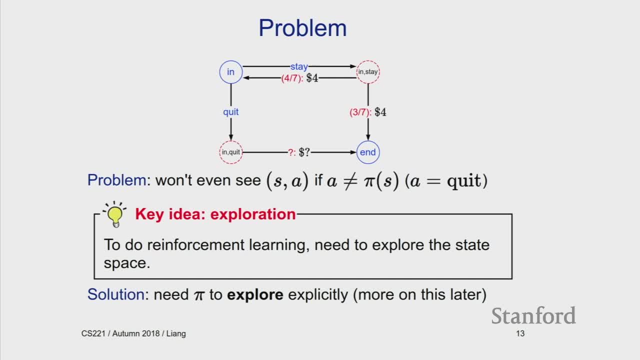 uh, try to solve it now. Um, for now you can just think about pi as a random policy, because a random policy eventually will just, you know, hit everything, for you know finite uh uh, small uh state spaces. 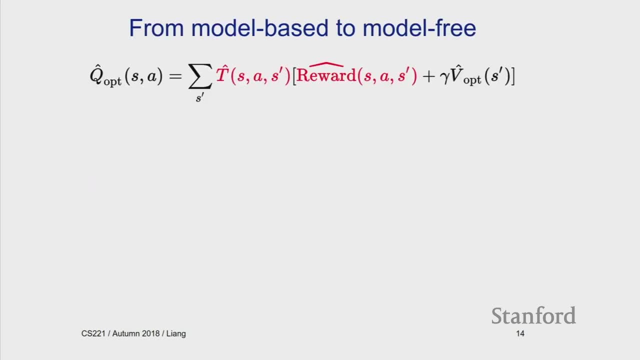 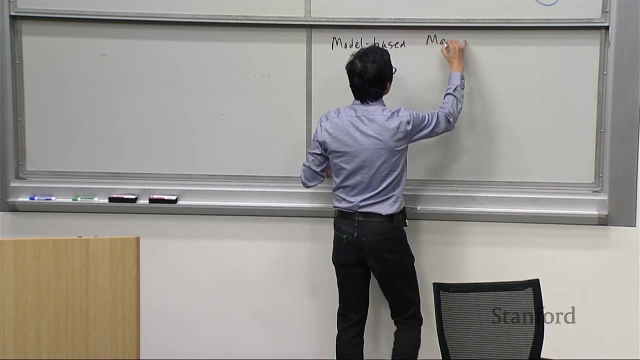 Okay, So, um, okay. So that's basically the end of the first algorithm. Let me just write this over here. So, algorithms: we have model-based um, Monte Carlo Um, and the model base is referring to the fact that we're estimating a model. 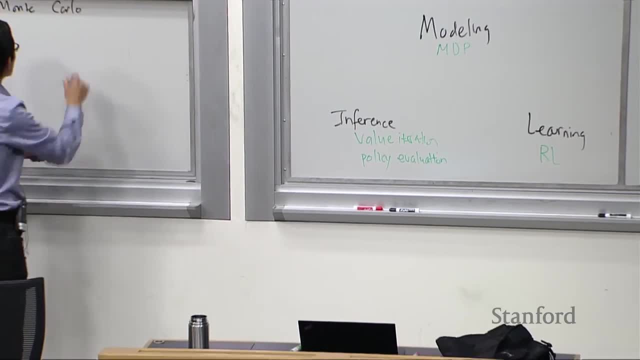 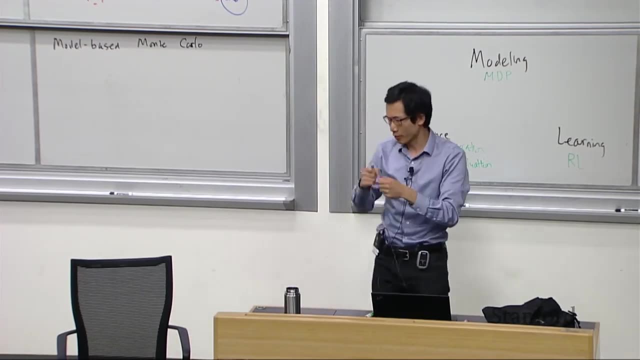 the, in particular the MDP, The Monte Carlo part is just referring to the fact that we're using samples uh to estimate um a model, or you're basically applying the policy multiple times and then estimating um the model based on averages. 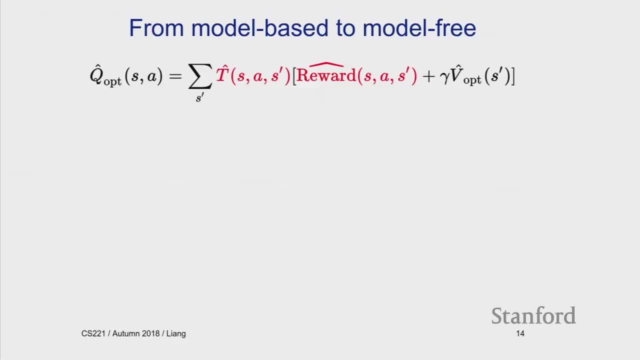 Okay, So. so now I'm going to present, uh, a different algorithm, and it's called uh, model-free Monte Carlo, And you might, from the name, guess what we might want to do is: maybe we don't have to estimate this model. 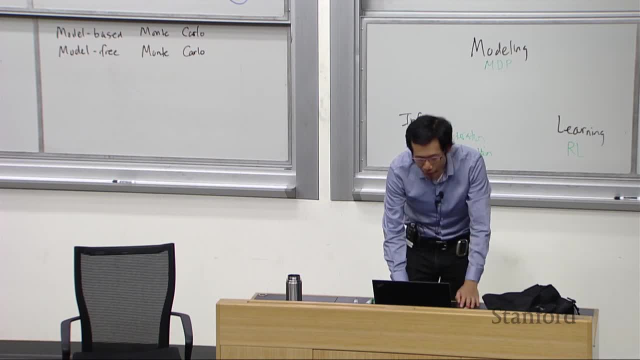 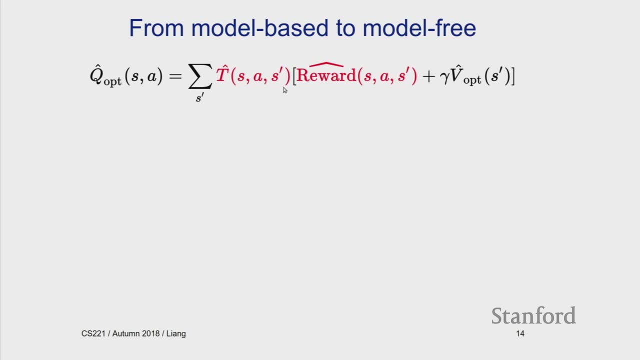 Okay, And why? why is that? Well, what do we do with this model? Um, what we did was we, you know, uh, presumably use value iteration to, um, you know, compute the optimal policy And the. remember this, uh. 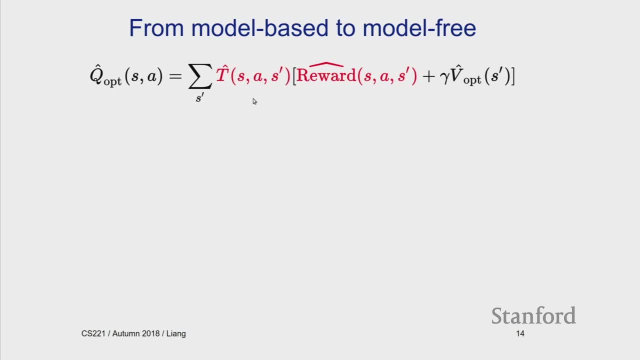 recurrence um. for computing Q-Opt Um, it's in terms of t and reward, but at the end of the day, all you need is Q-Opt. If I told you um, Q-Opt SA, which is um, 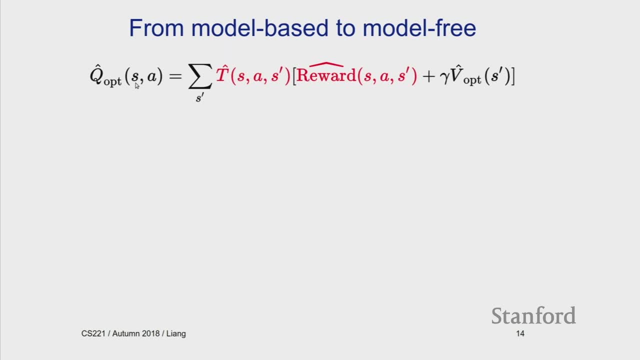 what is Q-Opt SA? It's the um, the maximum possible utility I could get. if I am in chance node SA and I followed optimal policy. So clearly. if I knew that then I would just produce optimal policy and I would be done. 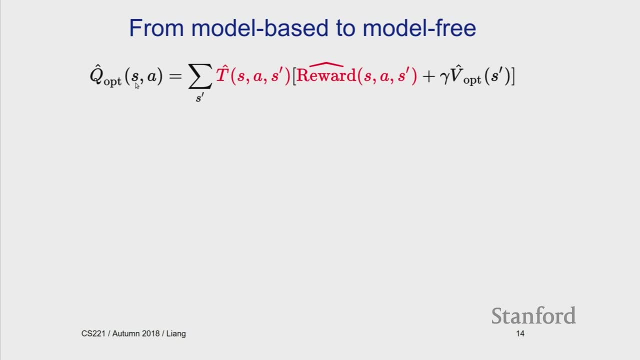 I don't even need to know, understand the, the rewards and transitions. Okay, So with that, uh, insight is model-free learning, which is that we're just gonna try to estimate Q-Opt. um, you know directly. 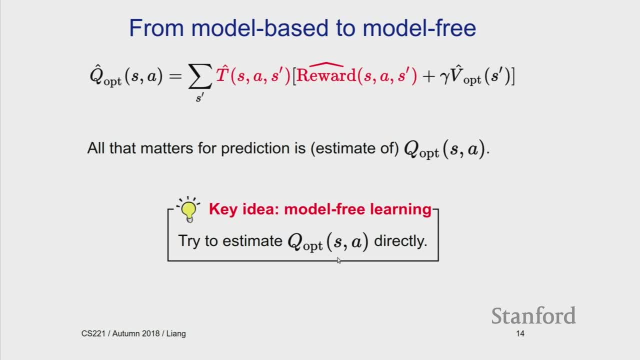 Um, sometimes it can be a little bit confusing what is meant by model-free. So, Q-Opt itself, you can think about it as a as a model, but in the context of MDPs and reinforcement learning, generally people when they say model-free refers to the fact that there's 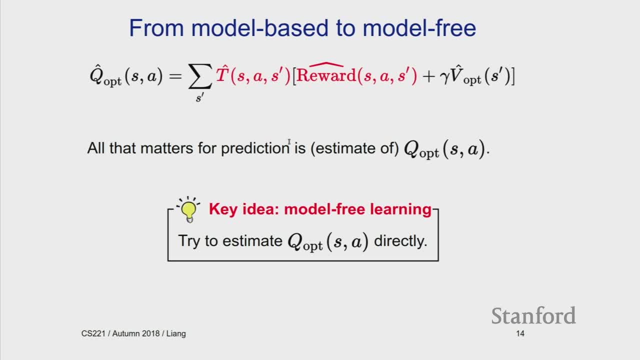 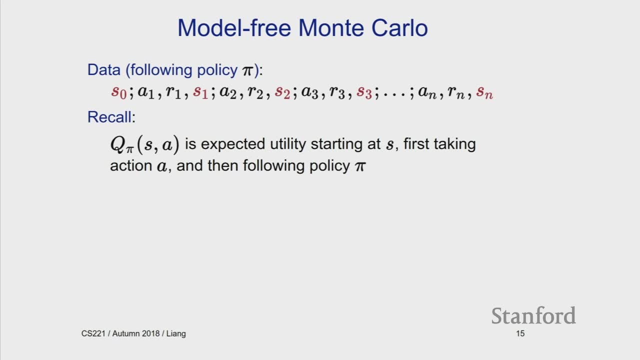 no MDP model, not that there is no um model in general. Okay, So, um, so we're not gonna get to Q-Opt, uh, yet. Um, that'll come later in the lecture. So let's warm up a little bit. 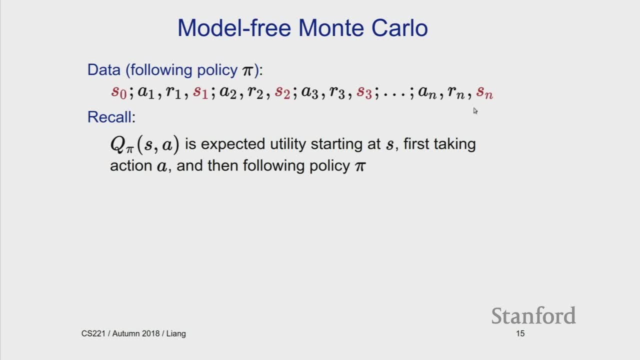 Um. so here's our data staring at us. Um, remember, let's. let's look at a related quantity. So Q-Pi. remember what Q-Pi is? Q-Pi of SA is the expected utility if we start at S. 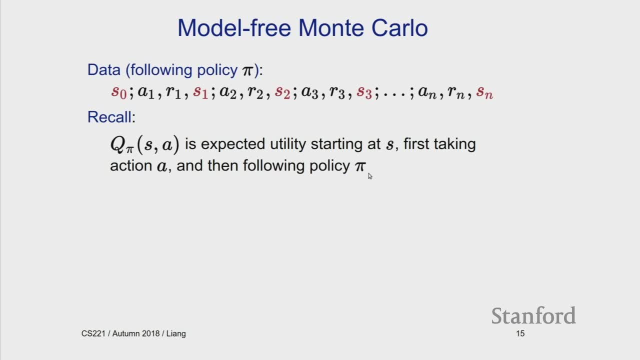 and you first take action A and then follow policy Pi right, So in um, in. I guess another way to write this is um. if you are at a particular uh time, step t, you can define u t as the. 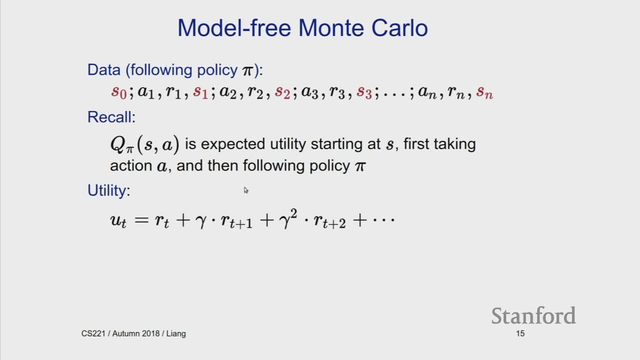 the discounted sum of the rewards from that point on, which is, you know the reward immediately that you would get plus discounted. uh, in the nine- next time, step, plus, you know a square discounted, and then, uh, two time steps in the future, and so on. 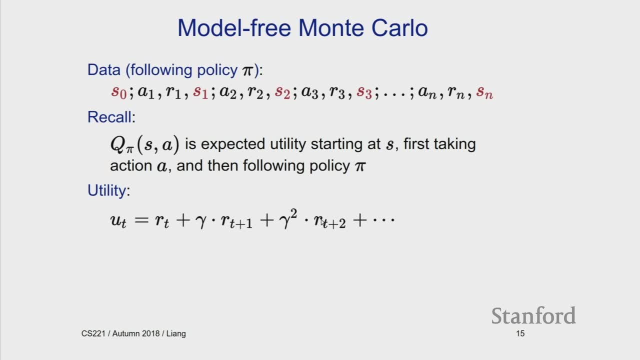 And, um, what you can do is you can try to estimate Q-Pi from this utility, right? So this is the utility, uh, that you get at a particular time step. So suppose you do the following: So suppose you average the utilities that you get only on the time steps. 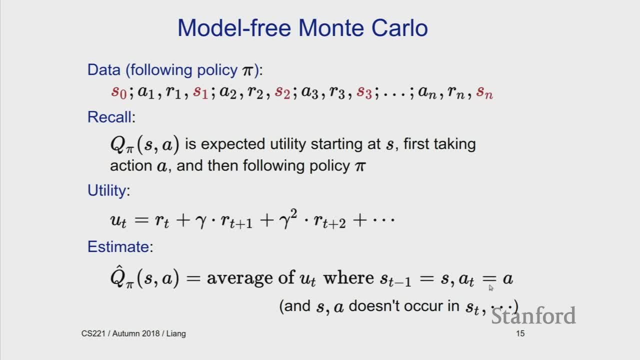 where I was in a particular state S and I took an action, A. okay, So you have a- let's suppose you have a bunch of episodes, right? So, um, here a picture: Victorially, um uh. 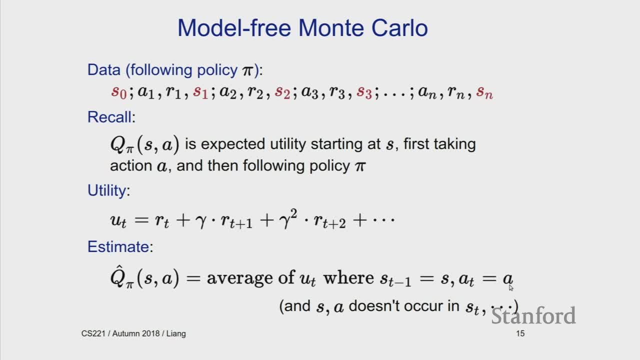 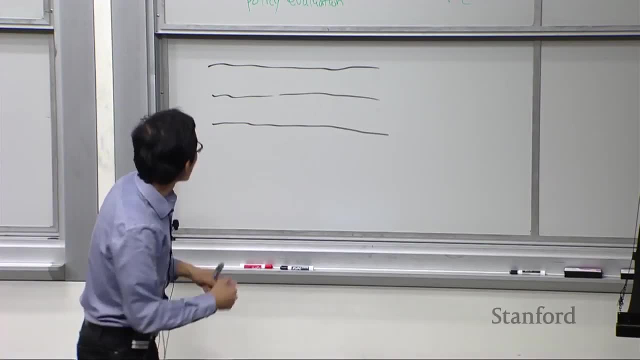 let's see, Here's another way to think about it. So I get a bunch of episodes. I'm gonna do some abstract um drawing here, Um. so every time you have you know, S A shows up here. maybe it shows up here. 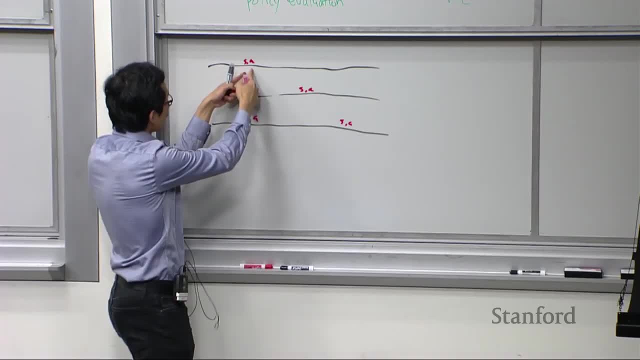 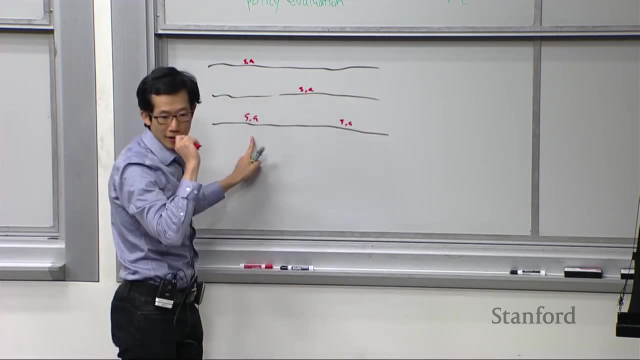 maybe it shows up here. maybe it shows up here. you're gonna look at: how much reward did I get from that point on. How much reward did I get from here on? How much reward do I get from here on And um average them. 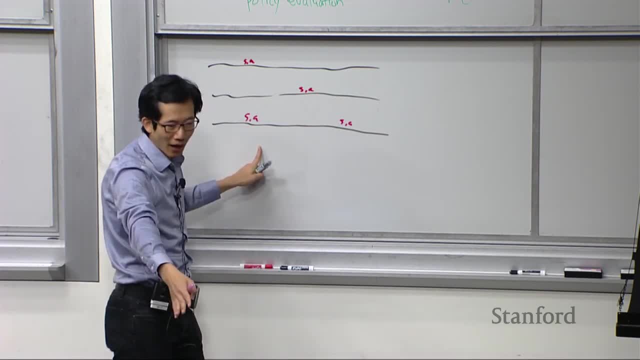 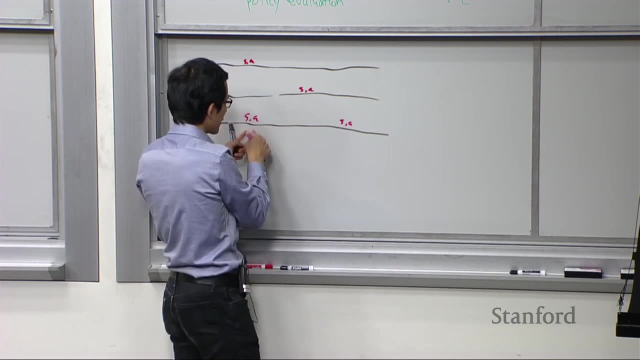 Okay, Right, So- and there's a kind of a technicality, which is that if S A appears here and it also appears uh after it, then I'm not gonna count that, because I'm kind of- if I do both. 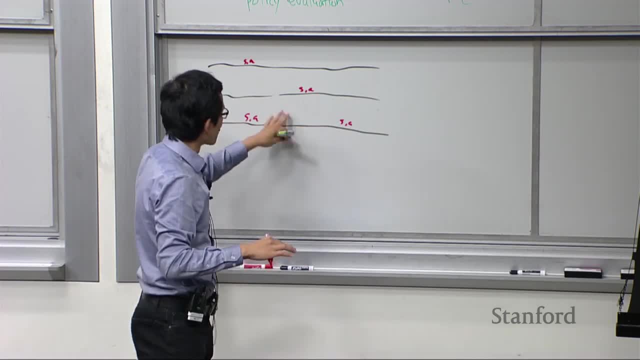 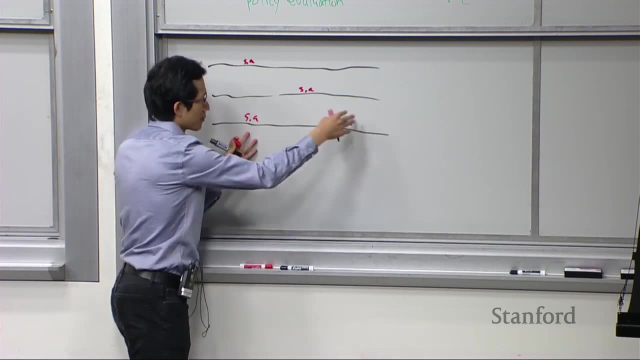 I'm kind of double counting. Um, in fact it works both ways, but just conceptually it's easier to think about just taking the uh, an S A if uh the same- you don't kind of go back to the same. 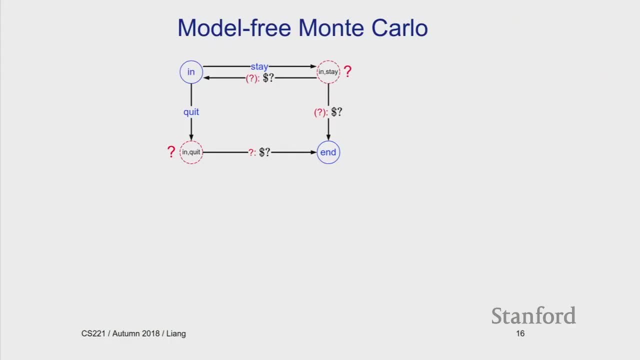 you know, uh position Okay, So let's do that on a concrete example. So q pi, let's just write it. q pi S. A is a thing where we're trying to estimate, And this is a- a value associated with every chance. node S A. 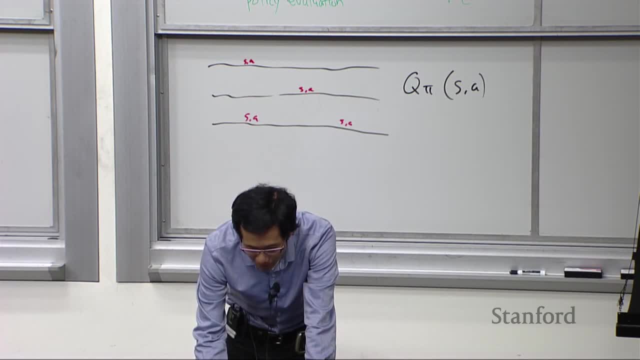 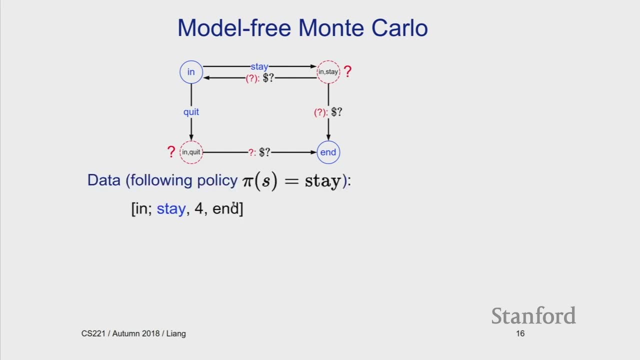 So in particular, I've drawn it here: I need a value here and a- a value here. Okay, So suppose I get some data, I stay and then I get- go to the end. Um, so what's my utility here? 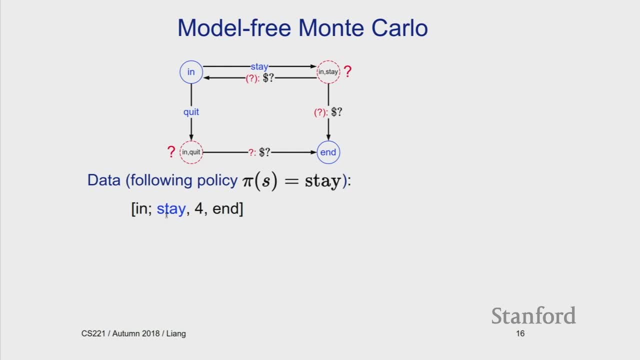 It's not a trick question: Four, Four, Yes, Um sum of four is four. Okay, So now I can say, okay, it's four. That's my best guess so far, I mean, I haven't seen anything else. Maybe it's four. 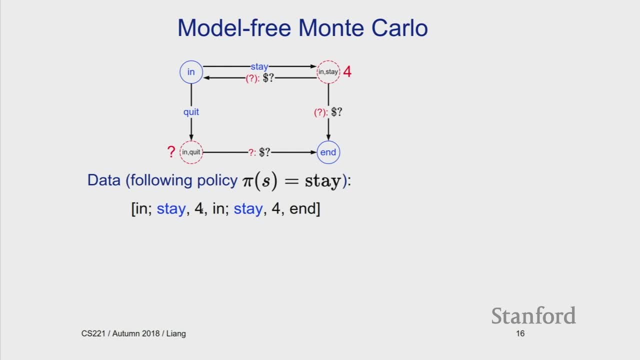 Um, so what happens if I play the game again and I get four, four, So what's the utility here? Eight, So then I update this to the average of four and eight. I do it again, I get 16, then I average, uh, in the 16.. Okay. 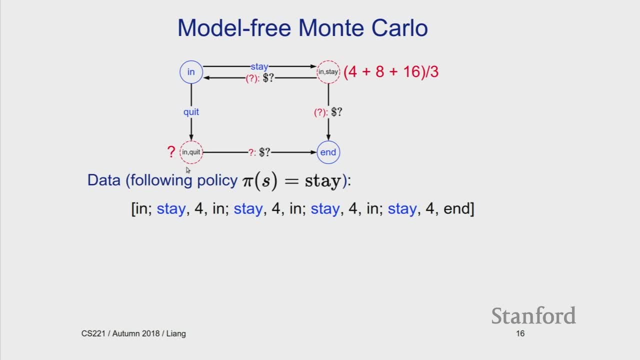 And um and again. you know I'm using state, so I don't learn anything about this In practice. you would actually go explore this and figure out how much utility is sitting there. So in particular notice: I'm not updating the rewards nor the transitions, because I'm model-free. 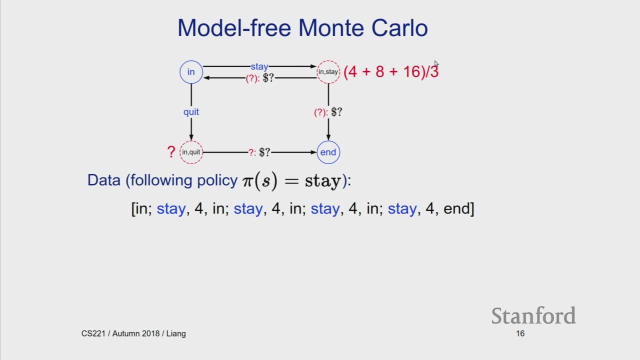 I just care about the Q values that I get, which are the values that sit at the nodes, not on the edges. Okay, So one caveat, uh is that we are estimating Q-pi, not Q-opt. We'll revisit this um later. 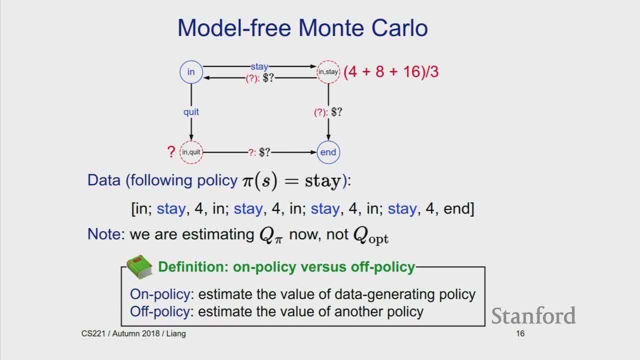 Um, and another uh thing to kind of note is the difference between what is called on-policy and off-policy. Okay, So in reinforcement learning you're always following some policy to get around the world, right? Um and uh, that's generally called the exploration policy or the control policy. 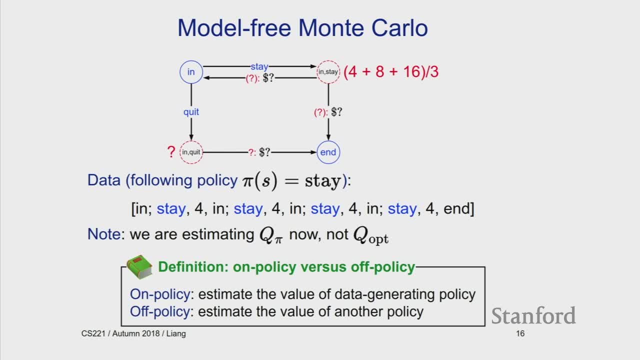 Um, and then there's usually some other thing that you're trying to estimate, usually the- the value of a particular policy, and that policy could be the same or it could be different. So on-policy means that, um, we're estimating the value of the policy that we're following. 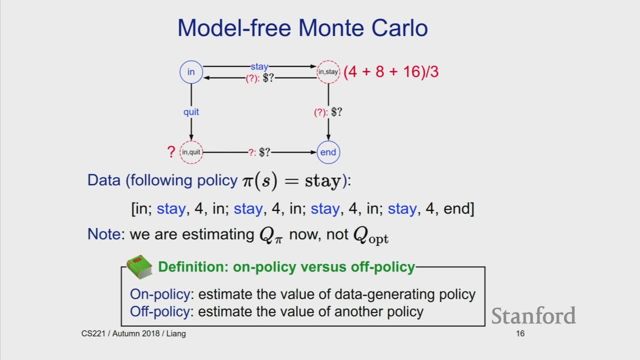 the gen- data-generating policy. Off-policy means that we're not okay, So um. so, in particular, is uh model-free Monte Carlo, um on-policy or off-policy? It's on-policy because I'm estimating q-pi, not q-opt, okay. 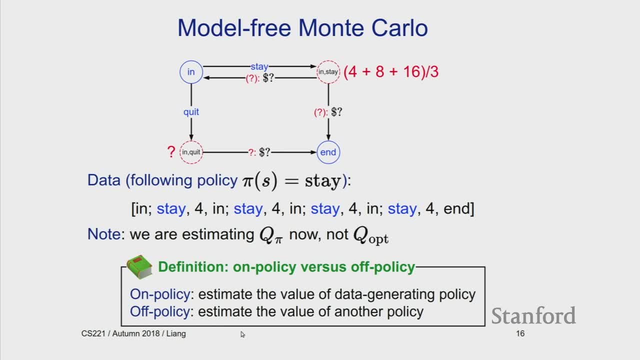 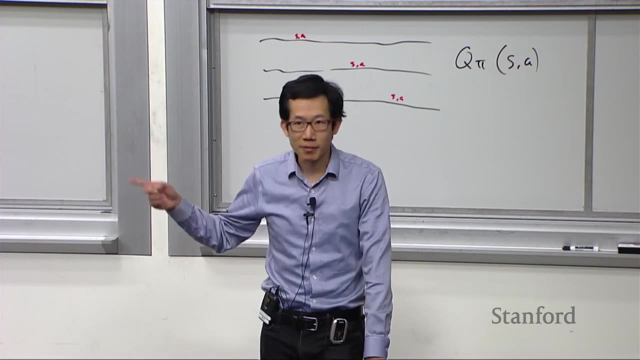 That's on-policy, Um, and off-policy. uh, what about model-based Monte Carlo? I mean, it's a little bit of a slightly weird question, but in model-based Monte Carlo, we're following some policy, maybe even random policy. 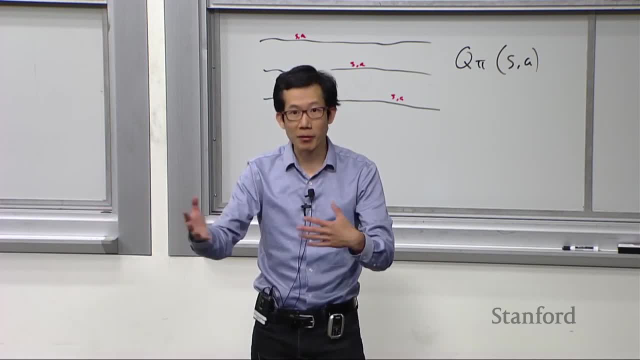 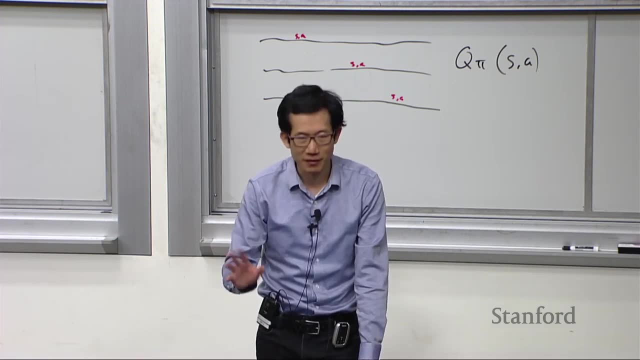 but we're estimating the transitions and rewards and from that we can compute the- the optimal policy. So you can- you can think about it as a um off-policy, but you know, that's maybe not, uh, completely standard. 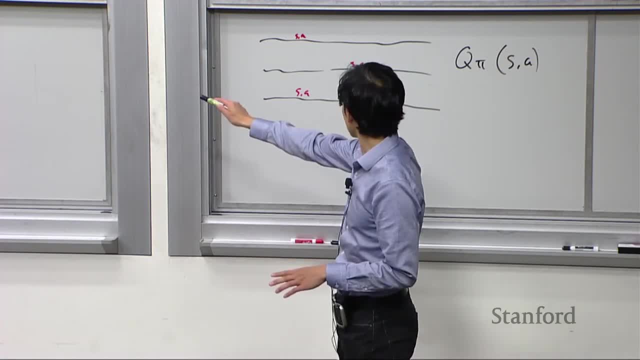 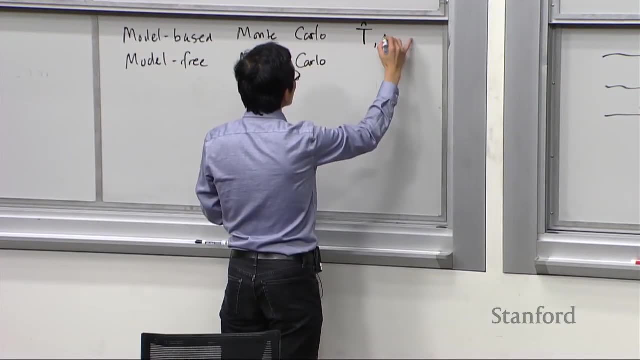 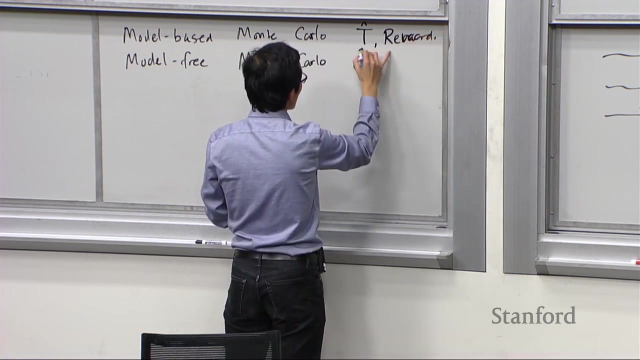 Okay, So any questions about what model-free Monte Carlo is doing? So let me just actually write. So what is model-based Monte Carlo is doing? It's trying to estimate the uh, the transition and rewards, and model-free Monte Carlo is trying to estimate uh. 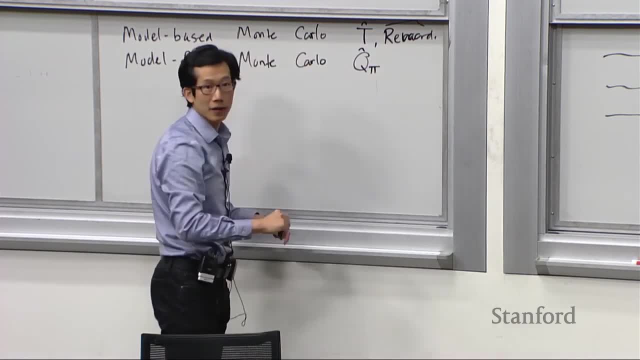 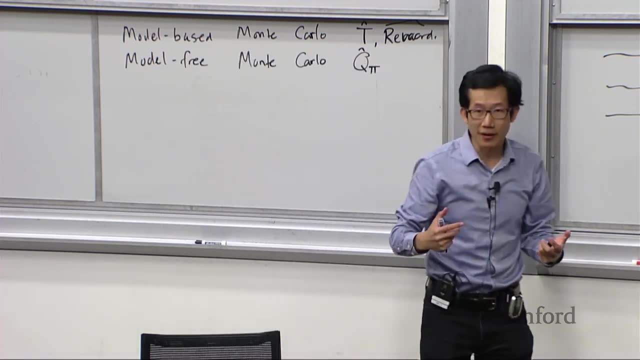 the um, q-pi, um, okay, And just as a note, I put hats on uh, any letter that is supposed to be a quantity that's estimated from data and that's what you know I guess statisticians do um. 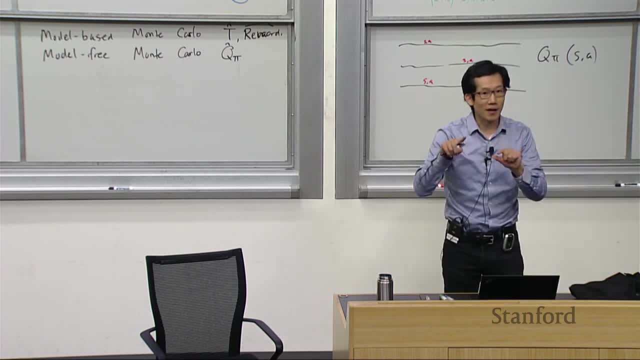 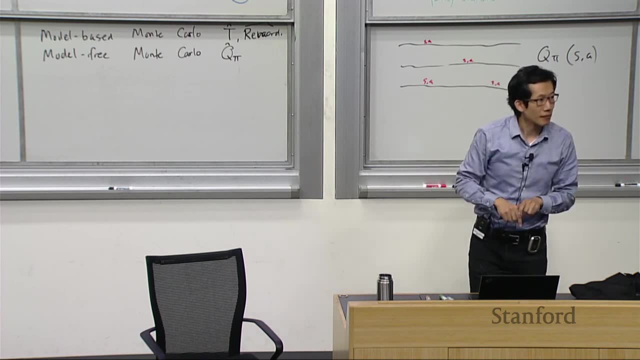 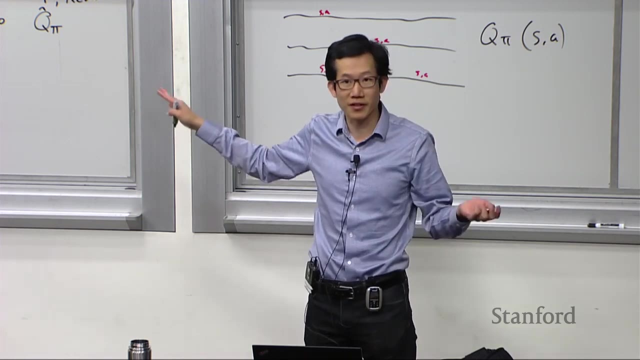 to differentiate them between whenever I write q-pi. that's the true uh value of that. you know policy, which you know. I don't have, Okay, Any questions about model-free Monte Carlo? Both of these algorithms are pretty simple, right. 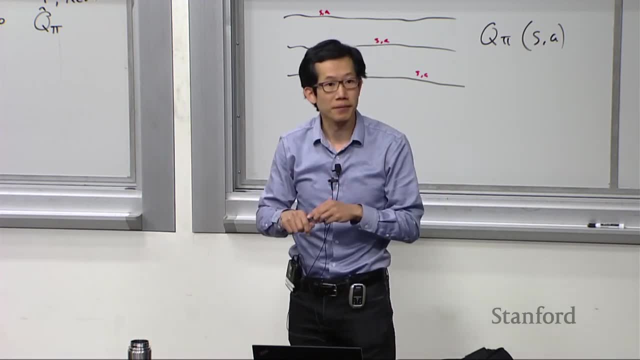 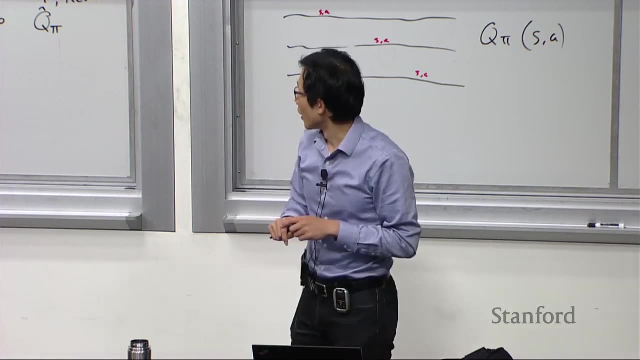 You just you know, you look at the data and you take averages. Yeah, So model-free is not trying to optimize the policy at all. You're not making changes to your policy, Uh. so question is: is model-free, uh, making changes to a policy or is it fixed policy? 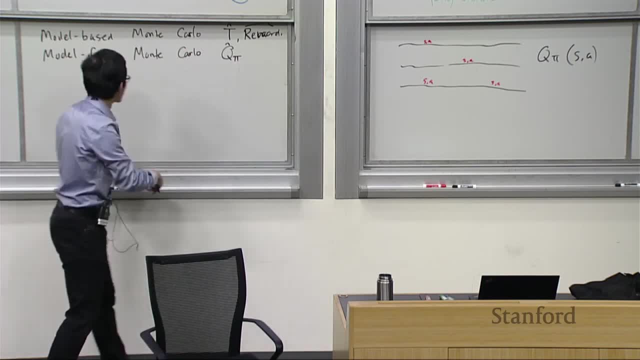 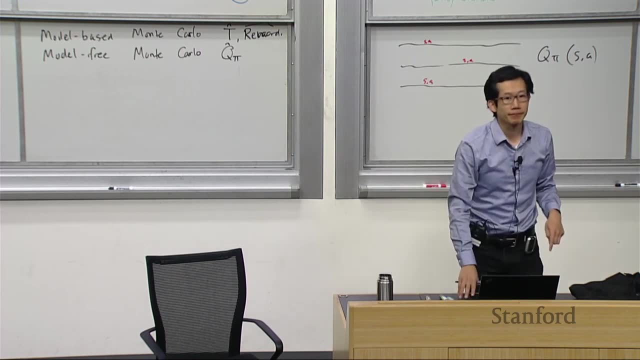 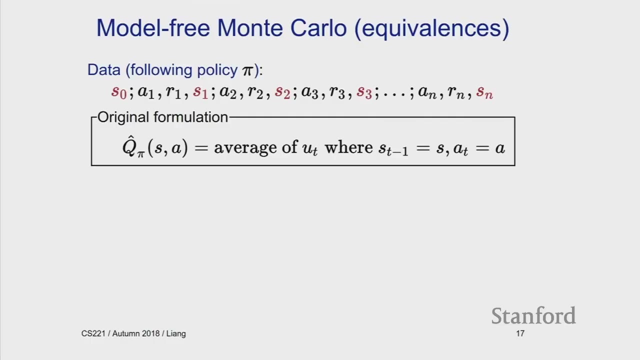 So so this version I've given you is only for a fixed policy, The general idea of model-free, as we'll see later. uh, you can also optimize a policy, Okay, So so now, what we're gonna do is we're gonna. 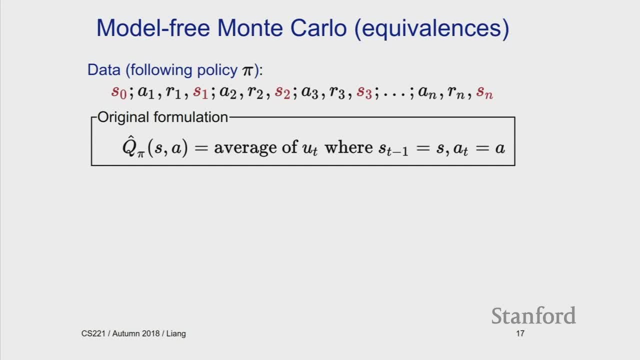 uh, do theme and variations on um model-free Monte Carlo? Actually we're. it's gonna be the same algorithm, but I just want to interpret it in kind of slightly different ways. That'll help us um generalize it in the future. Yeah. 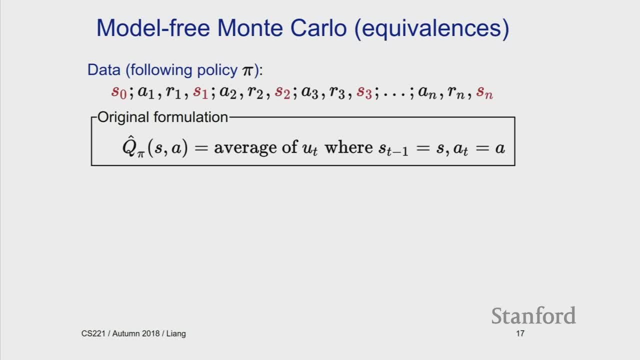 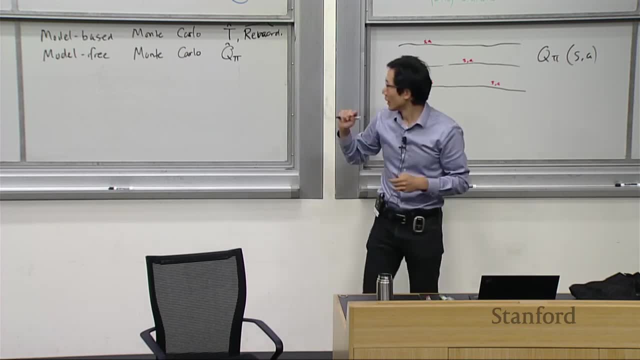 Are there certain problems where model-free is better than model-based? Are there certain problems where model-free is better than model-based? So this is actually a really interesting question, right? So, um, you can show that if your model is correct. 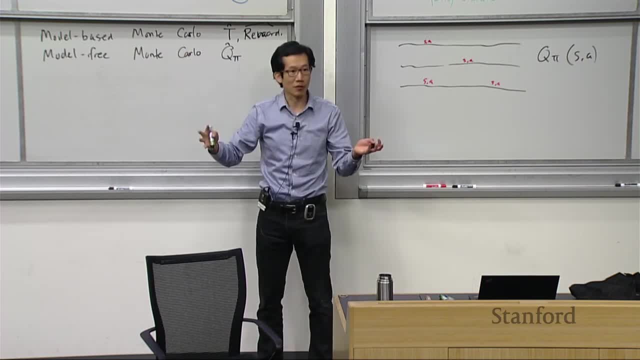 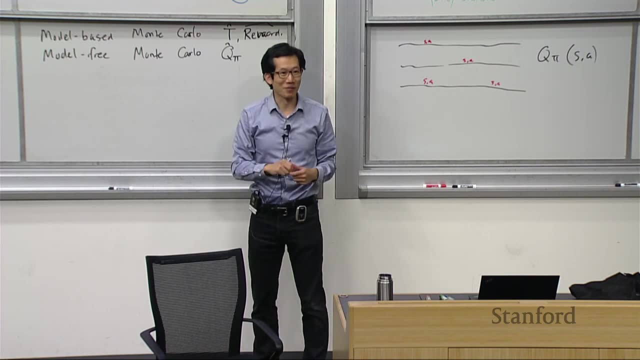 if your model of the world is correct. model-based is kind of the way to go because it will be more sample efficient, meaning that you need fewer ex- uh data points. But it's really hard to get the model correct in the real world. 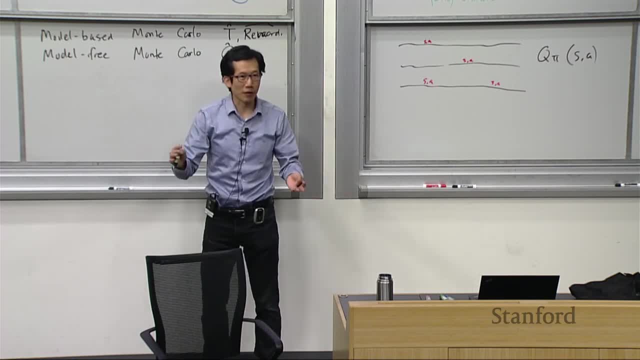 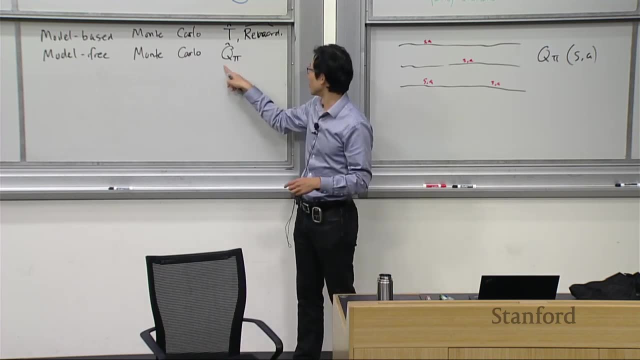 So recently, uh, especially with, you know, deep reinforcement learning- people have gotten a lot of mileage by just going model-free, because then, um, jumping ahead a little bit, you can model this as a kind of a deep neural network. 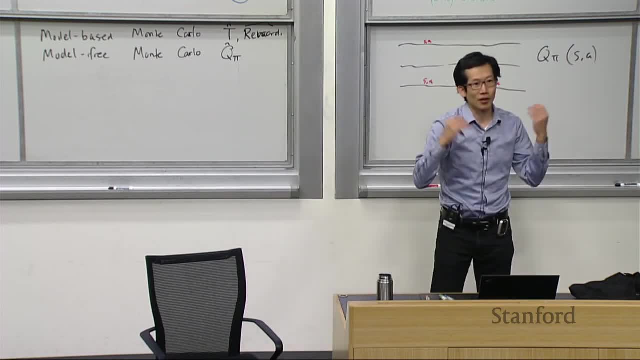 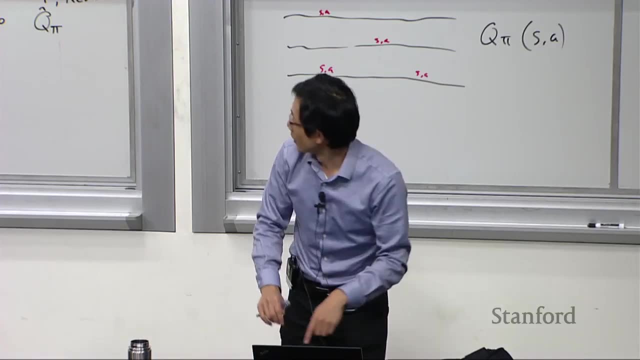 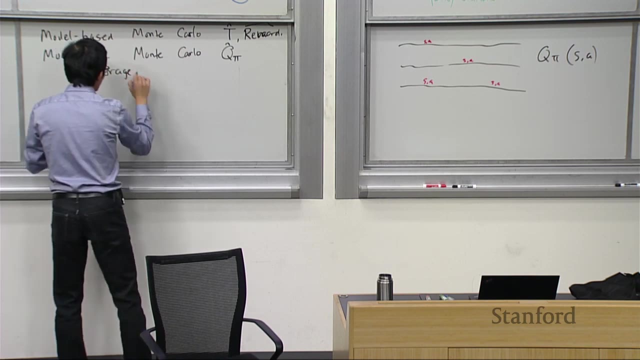 and that gives you an extraordinary flexibility and power without having to solve the hard problem of, you know, constructing the MDP Okay So so there's kind of three ways you can think about this. So the first- we already talked about it- is. 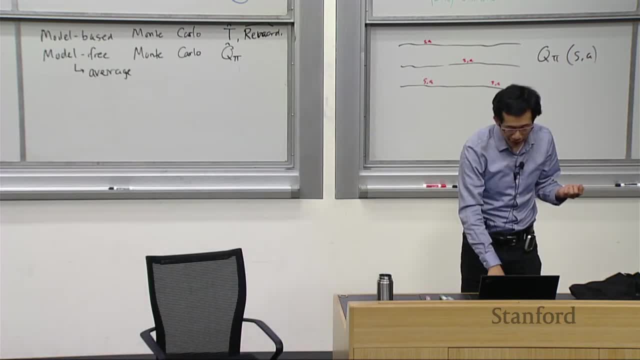 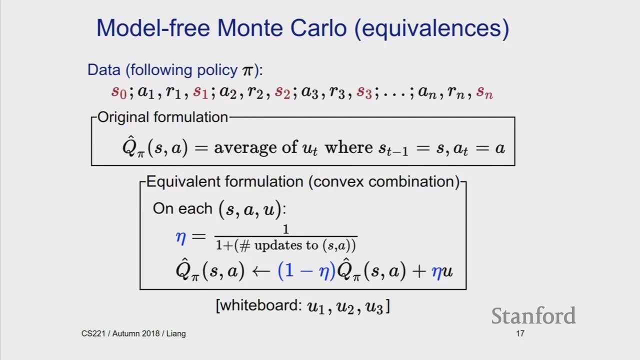 you know this average idea, So we're just looking at the utilities that you see whenever you counter an S and an A and you just average them. Okay, So here is an equivalent formulation: Um, and the way it works is that for every? 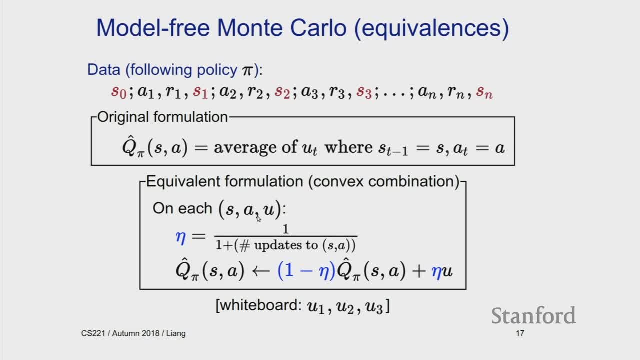 um, SAU that you see. so every time you see a particular SAU, SAU, SAU and so on, I'm going to perform the following update: Um, so I'm gonna take my existing value and I'm going to do a. 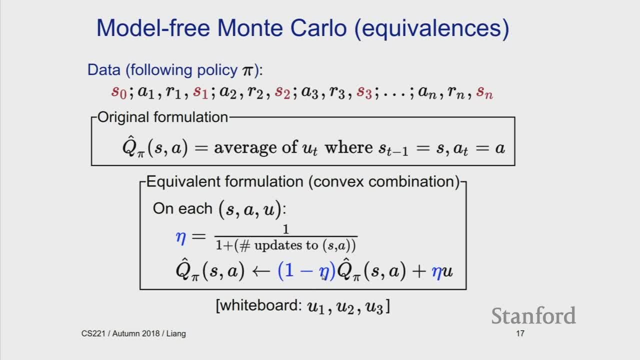 what we call a convex combination. So you know, 1 minus eta and eta sum to 1.. So it's, you know, kind of balancing between two things, Balancing between the old value that I had and the the new utility that I saw. 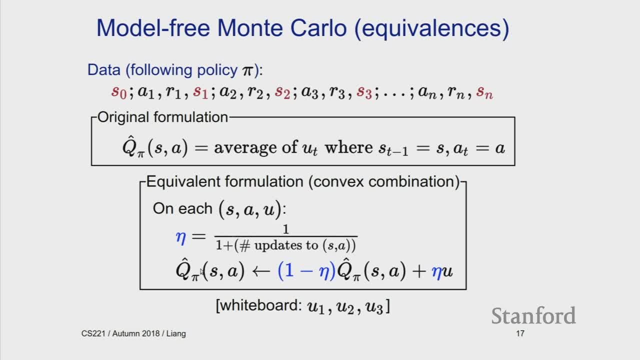 Okay, And the eta is set to be 1 over 1, plus the number of updates. Okay. So let me do a concrete example. I think it will make this very clear what's what's going on. So suppose my data looks like this: 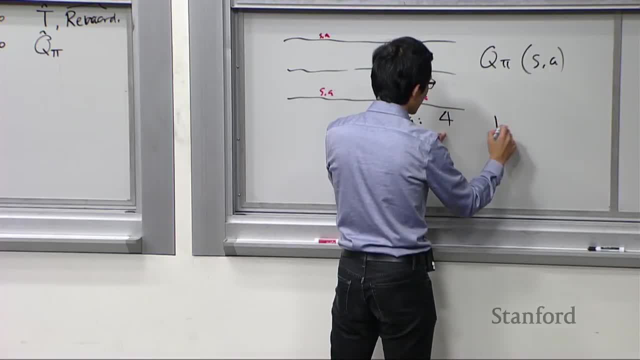 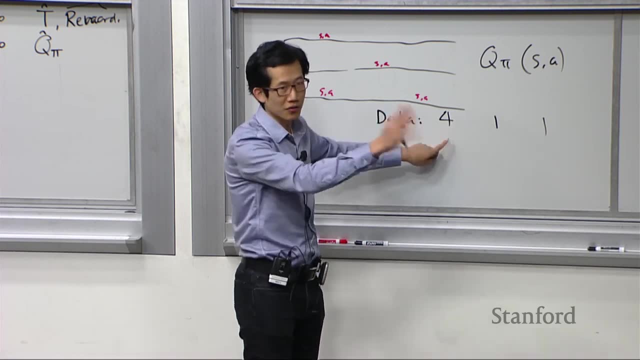 So I had got uh 4, um, and then a 1 and a 1.. Um, so these are the utilities, right? That that's a U. here I'm ignoring the S and the A, I'm just gonna assume that they're some something. 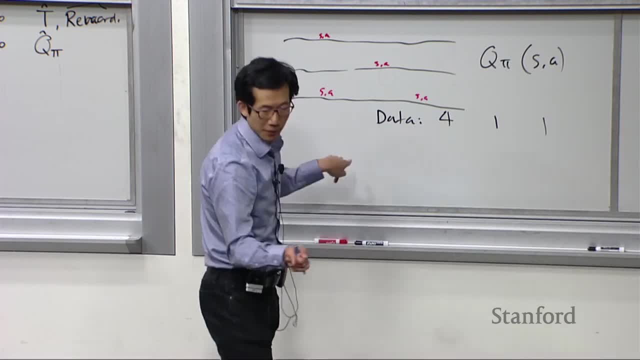 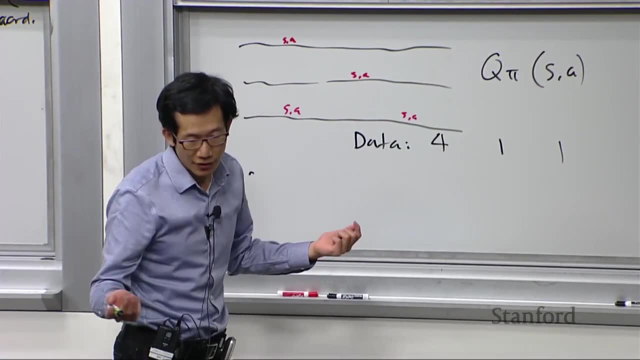 Okay, So first, uh, let's assume that Q, pi is 0.. Okay So the first time I do um. uh, let's see number of updates. I haven't done anything, So it's 1, um 1 minus 0.. 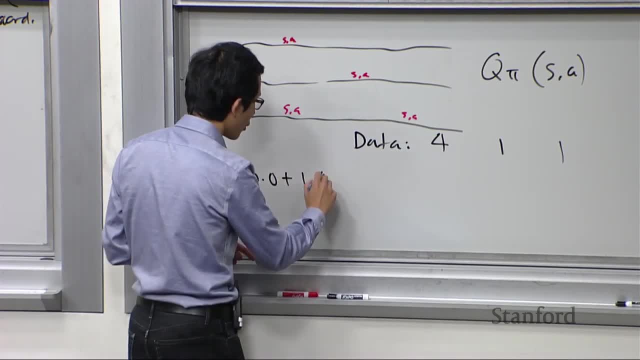 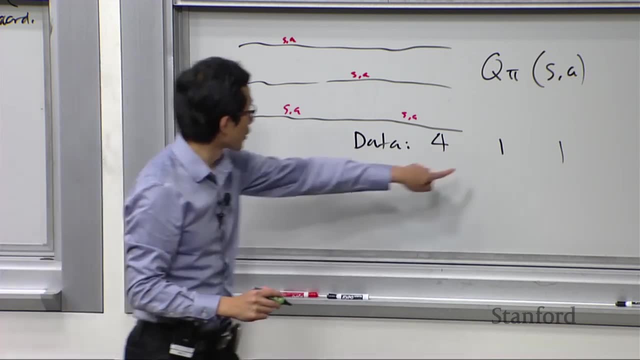 So 0 times 0 plus 1 times 4,, which is the first U that comes in. Um, okay, So this is 4.. Okay, So then what about the next data point that comes in? So I'm gonna take um. 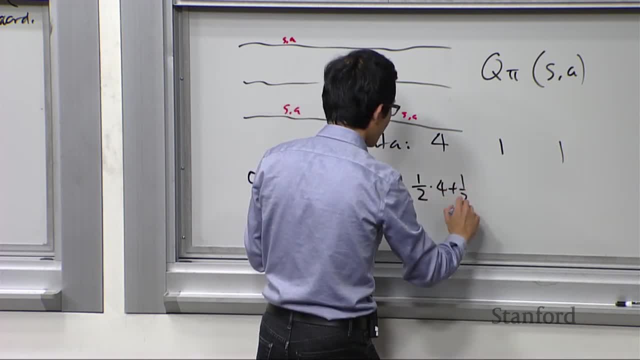 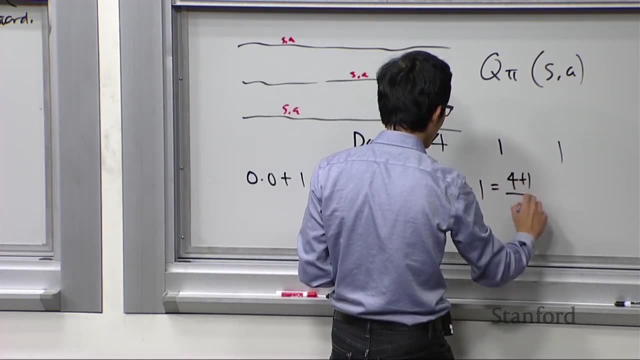 1 half now times 4 plus 1 half times 1, which is a new value that comes in, And that is: I'm gonna write it as 4 plus 1 over 2.. Okay, So now. okay, just to keep track of things. 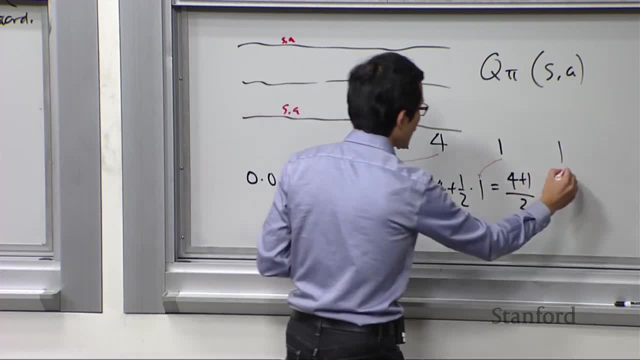 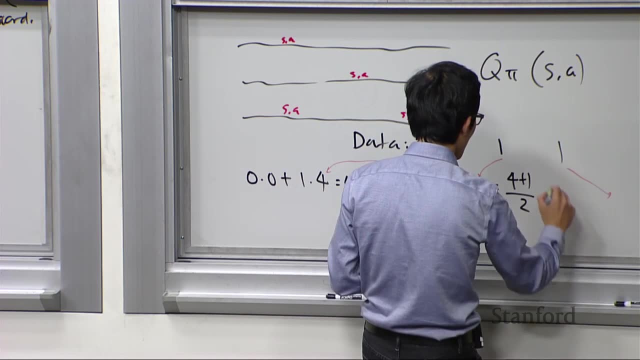 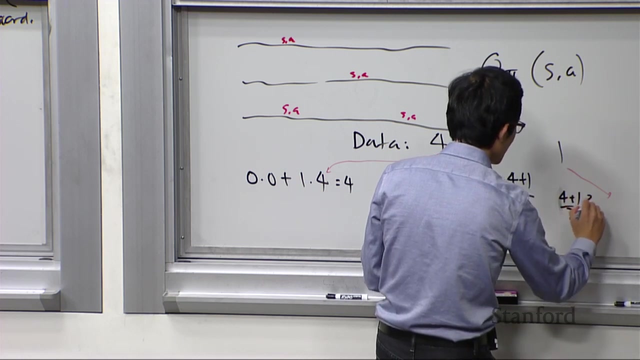 this results in this, this results in this. and then now, um, I'm running out of space, but hopefully I can, So now, on the third one, I do: um, uh, two-thirds, So I have 4 plus 1, over 2 times two-thirds plus. 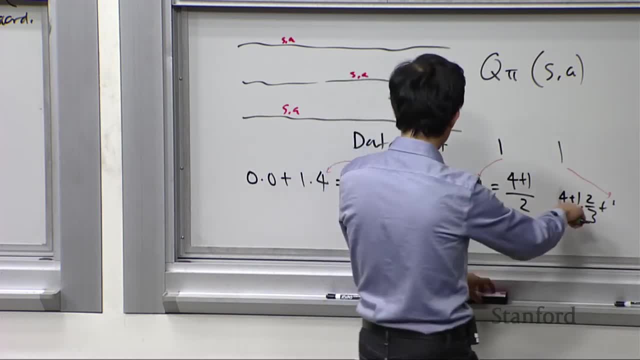 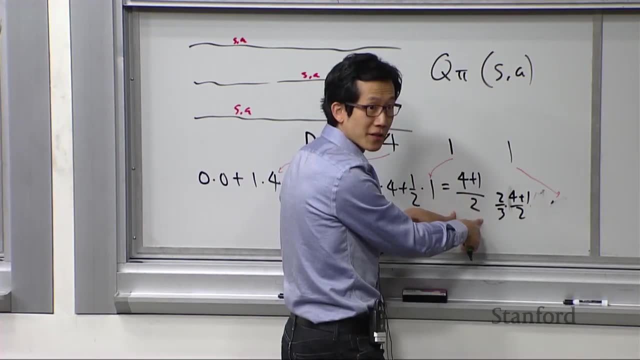 um, actually I I guess I should do two-thirds to be consistent. Two-thirds times 4 plus 1 over 2, which is a previous value, that's sitting in Q pi, plus a one-third times 1, which is a new value. 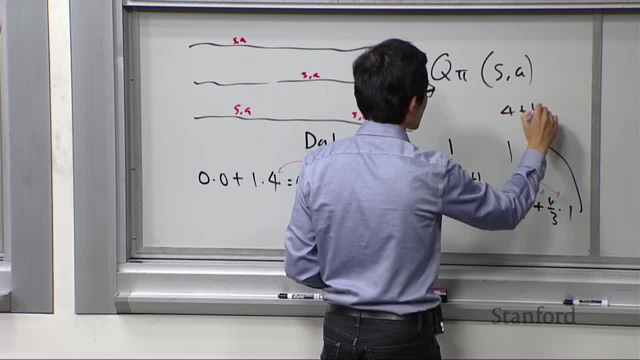 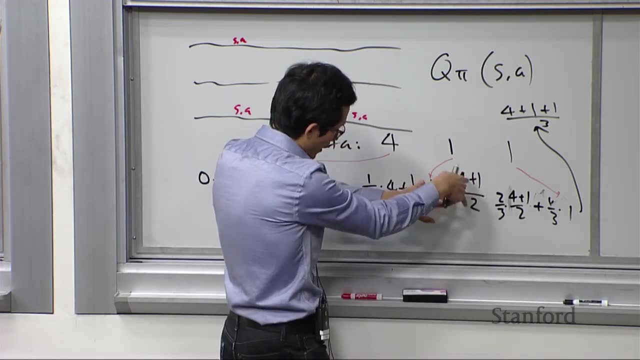 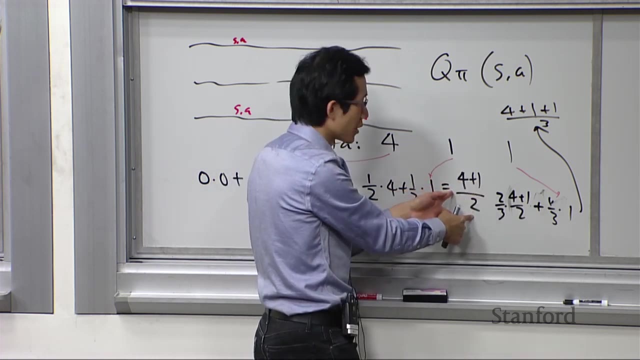 And that gives me um 4 plus 1 plus 1 over 3, right, So you can see what's going on here. is that you know each uh, each time I have this, you know, sum over all the two-thirds I've seen, over the number of times it occurs. 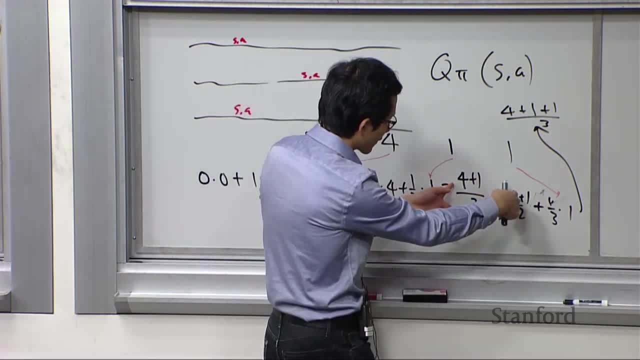 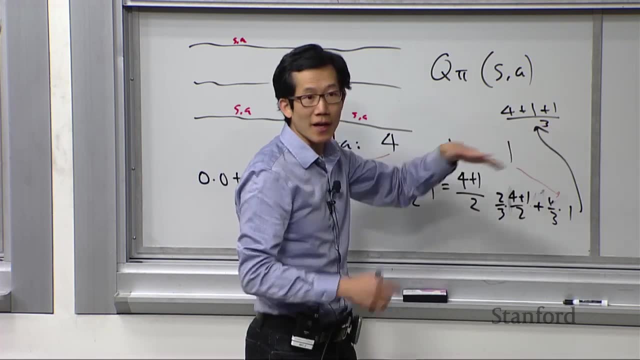 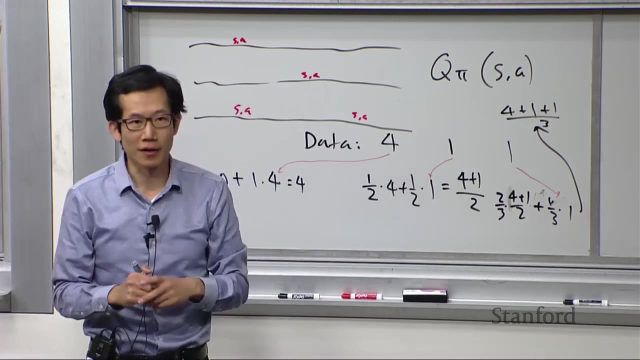 And this uh, eta is set so that next time I kind of cancel out the old account and I add the new count to the denominator and it kind of all works out so that at every time step what actually is in Q, pi is just the plain average over all the numbers. 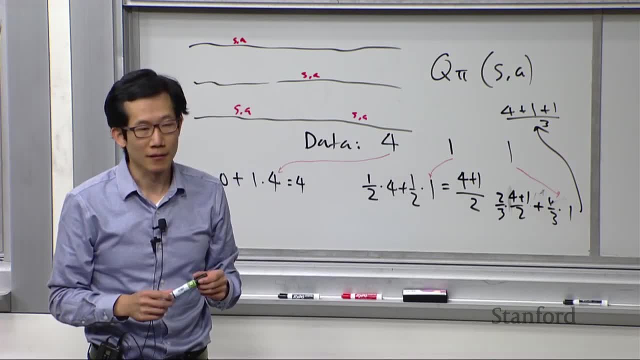 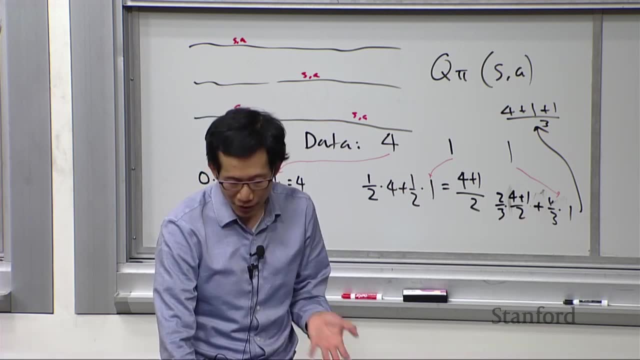 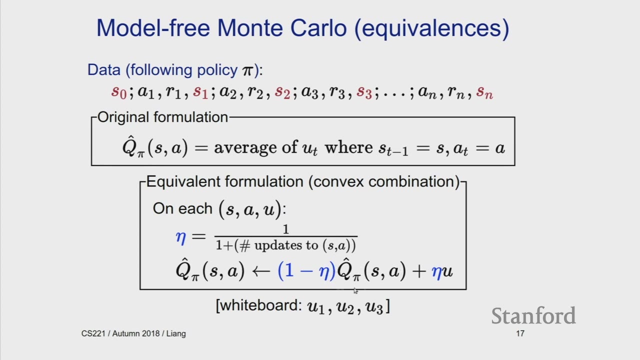 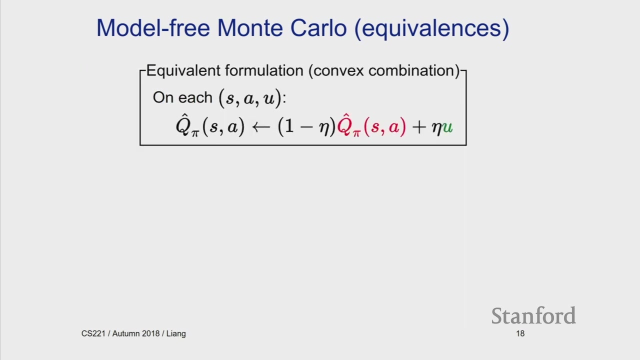 I've seen before. all right, This is just kind of algebraic trick to um get this original formulation, which is a notion of average, into this formulation, which is a notion of um, kind of, you're trying to um take a little bit of the old thing and add a little bit of a new thing. okay, 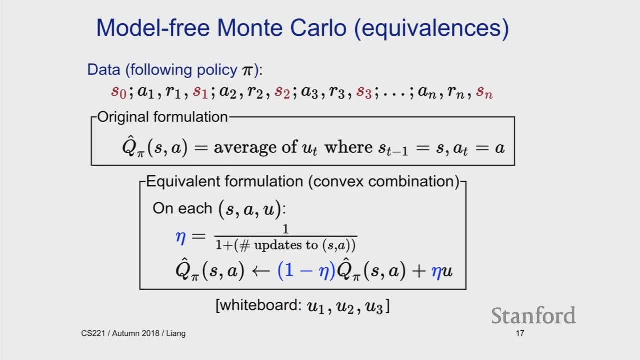 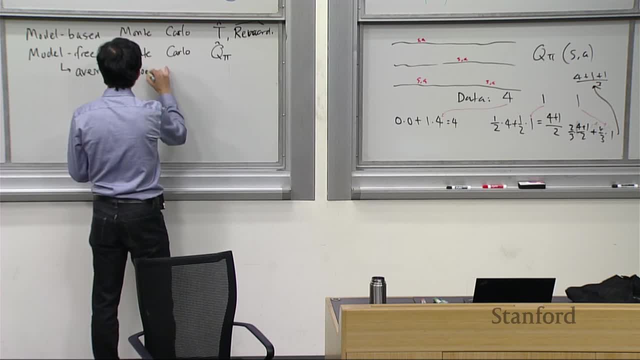 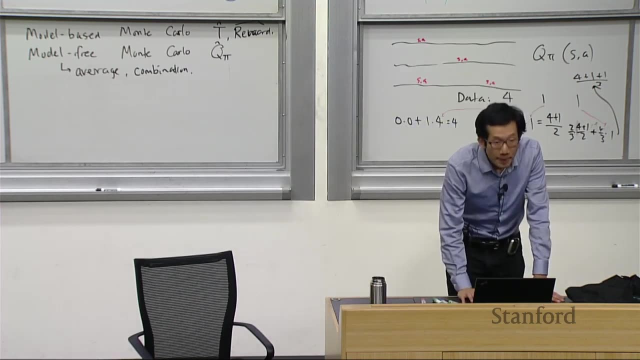 So, um, I guess I'm gonna call this, uh, I guess um combination, I guess. So that's the second interpretation. There's a third interpretation here, which, um, you can think about it as, uh, in terms of stochastic gradient, descent. 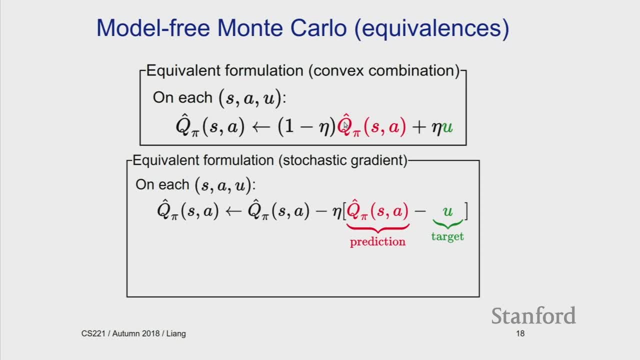 So this is actually a kind of a s- a simple algebraic manipulation. So if you look at this expression, what is this? So you have 1 times Q, pi, Um. so I'm going to pull it out and put it down here. 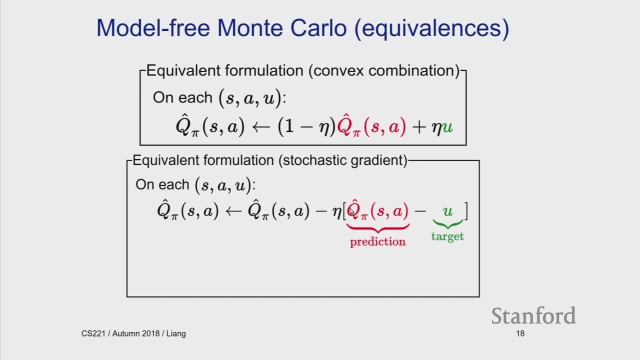 And then I'm gonna have minus eta times q, pi, that's this thing. And then I also have a eta a u, Um, so I'm gonna put kind of minus a u here and this is uh inside this friend. 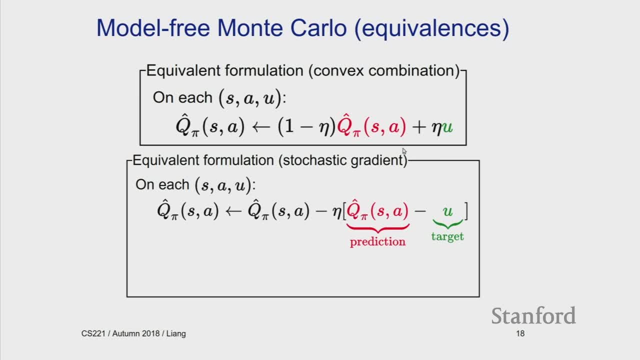 So, um, if you just, you know, do the, the algebra, you can see that these two, you know, are equivalent. Um, so what's the point of this Right? So, um, where have you kind of seen this, uh, before? 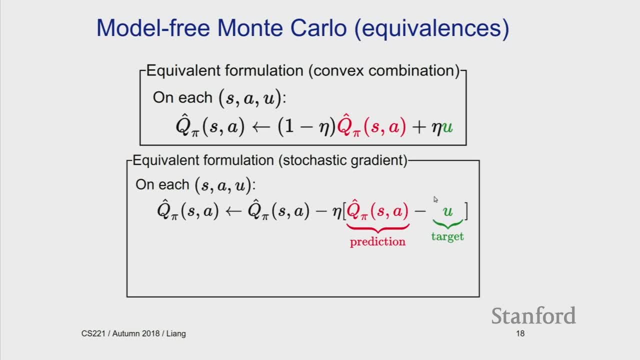 Something like: maybe not not this exact expression, but something like that. Any ideas? Yeah, when you looked at a stochastic gradient descent in the context of, uh, the square loss for linear regression, right. So remember, um, we had these updates that all looked like kind of prediction minus target. 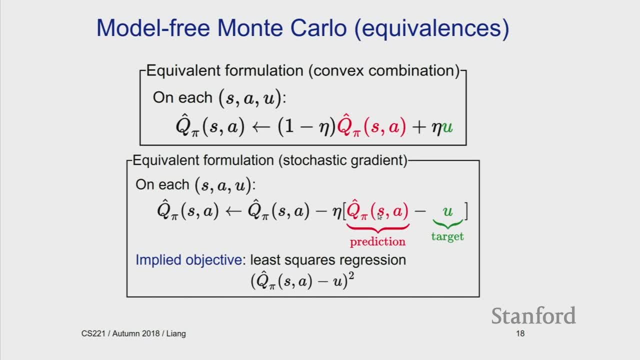 which was, you know, the residual and that was used to kind of update. So one way to interpret this is: um, this is kind of implicitly trying to do stochastic gradient descent on the objective, which is a squared uh. 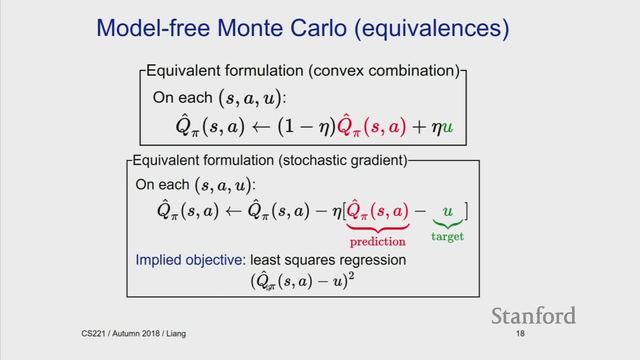 loss on uh, the, the q pi value that you, you you're trying to um set And um u, which is the new piece of data that you got. So think about in regression: this is the y, This is uh. 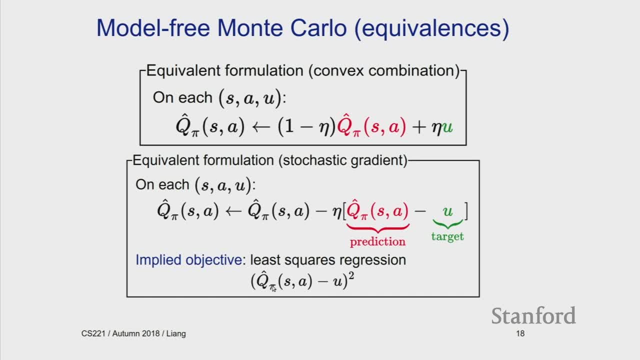 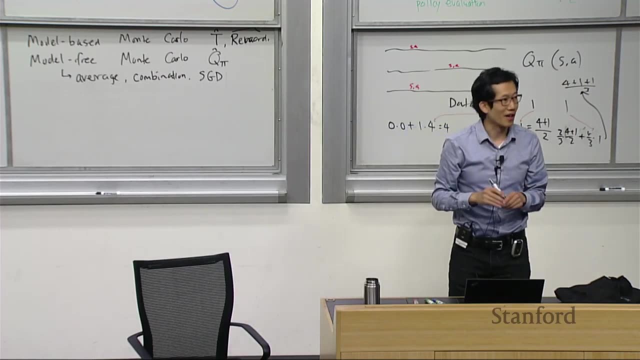 y, you know the, what the output is, And you this is the model that's trying to predict, And you want those to be close to each other. Okay, Okay, So so those are kind of three views on basically. 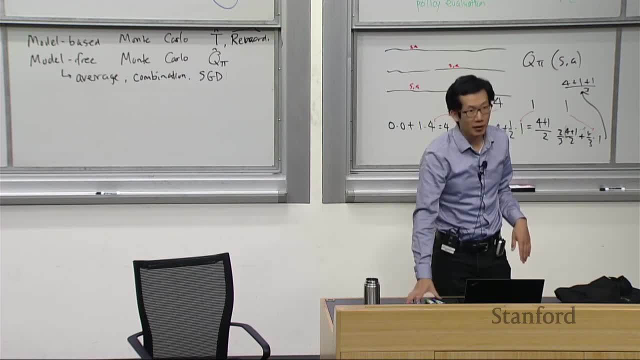 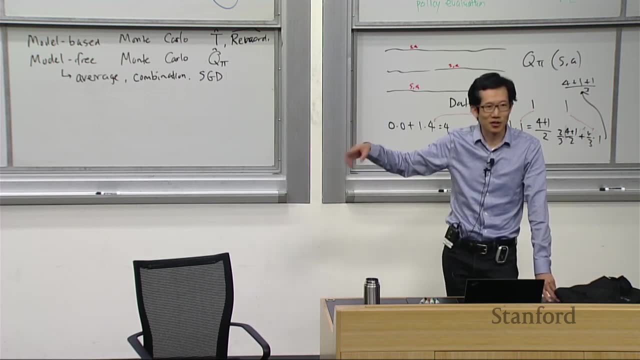 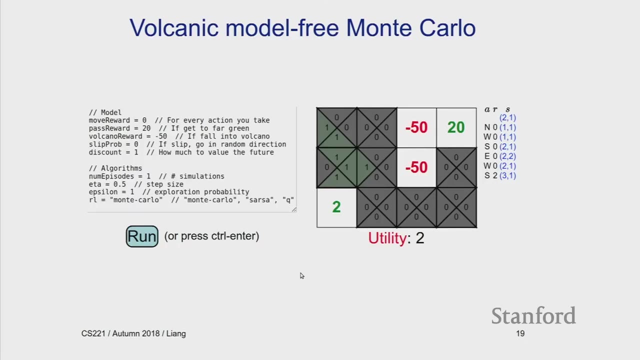 uh, this idea of averaging, or, um, incremental updates. Okay, So it'll become clear why. you know, I, I did this, This isn't just to you know. have fun, Um, okay, So now let's uh see an example of model. 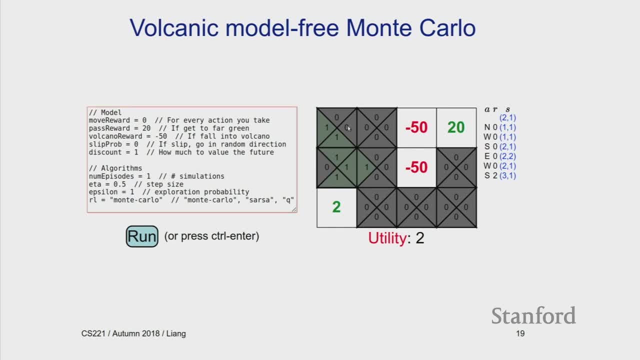 free Monte Carlo in action on this, um, the volcano game. So remember, here we have this, uh, you know, volcanic example And, um, I'm going to uh set the number of episodes to, let's say, 1,000.. Let's see what happens. 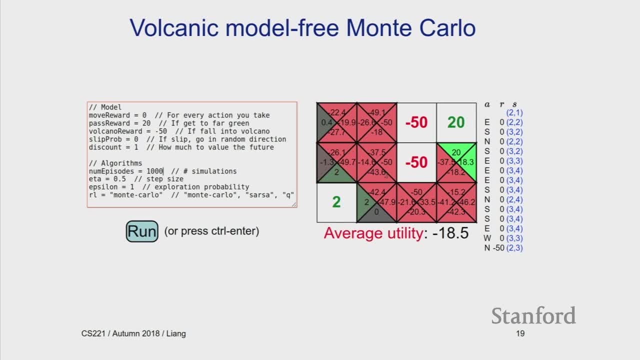 Um, so here, okay, So what is this kind of uh uh, grid-like structure, grid of triangles denote? So this, remember, is a state. This is two comma one, So what I'm doing here is dividing into: 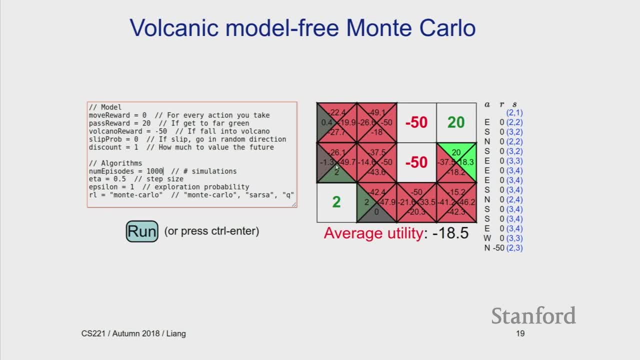 four pieces which correspond to the four different actions. So this triangle is two comma one north, this triangle is two comma one east, and so on. Okay, So, and the number here is the q-pi uh value that I'm estimating along the way. 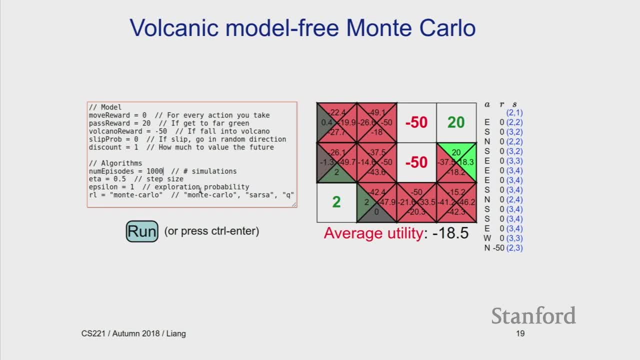 Okay, So the the policy I'm using um is complete random um just move randomly Um and I run this 1,000 times um and we see that the average um utility is um. you know. 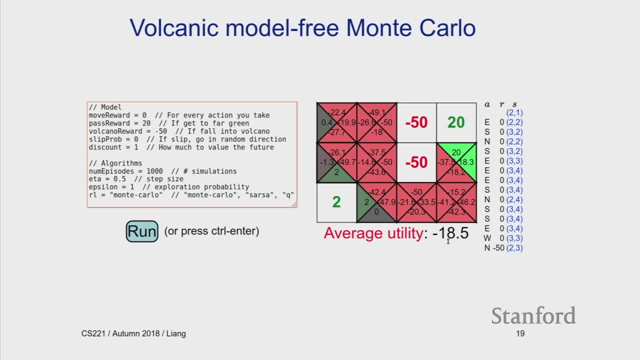 minus 18, which is, uh, obviously not great. Okay, Um, but this is an estimate of how well the random policy is doing. So, you know, as advertised, you know random policy, you would expect to fall into a volcano quite often. 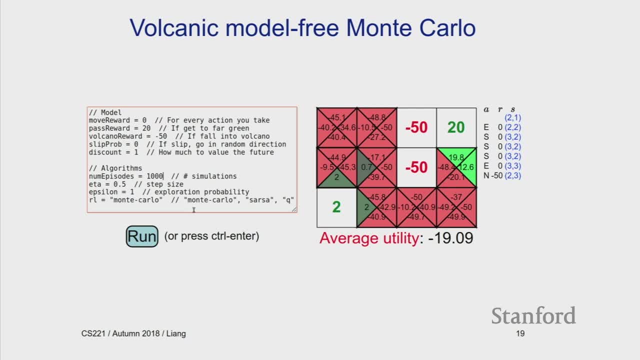 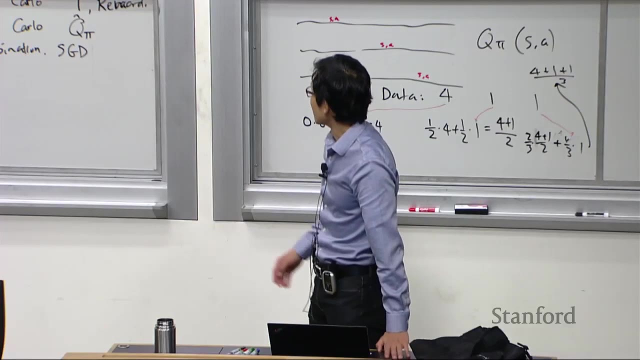 Um, okay, Um, and you can run this and sometimes you get slightly different results, but you know, it's pretty much stable around minus 19, minus 18.. Okay, Any questions about this before we move on to? 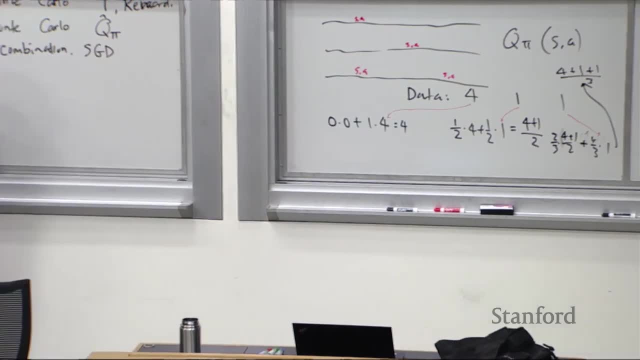 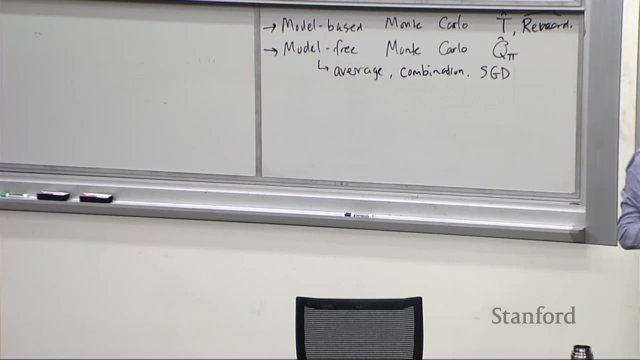 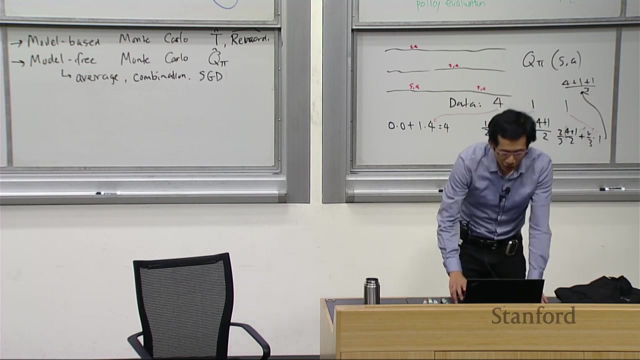 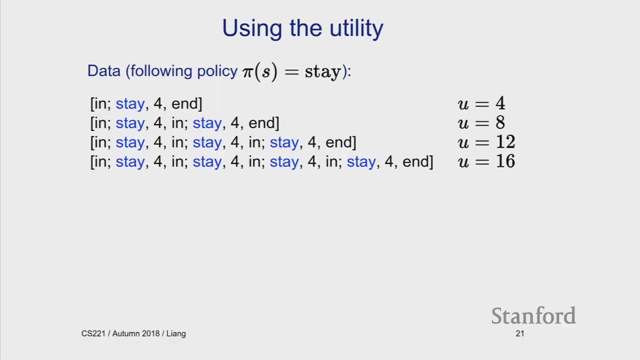 um different algorithms. Okay So, model-based Monte Carlo: we're estimating the MDP. model-free Monte Carlo: we're just estimating the q- values of a particular policy for now. Okay So so let's revisit what uh, Model-Free Monte Carlo is doing. 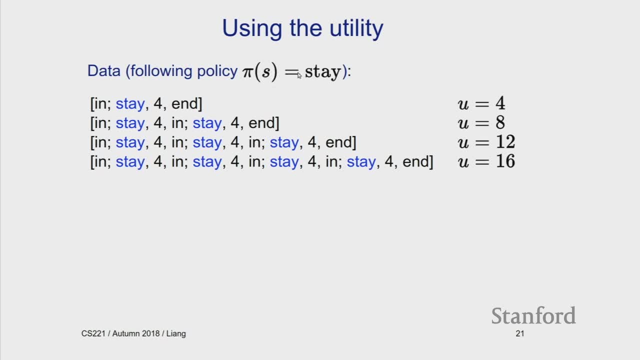 So if you use a policy pi equals state for the dice game, um, you know you might get a bunch of different um trajectories that come out. These are possible episodes and each episode you have a utility, you know, associated with that. 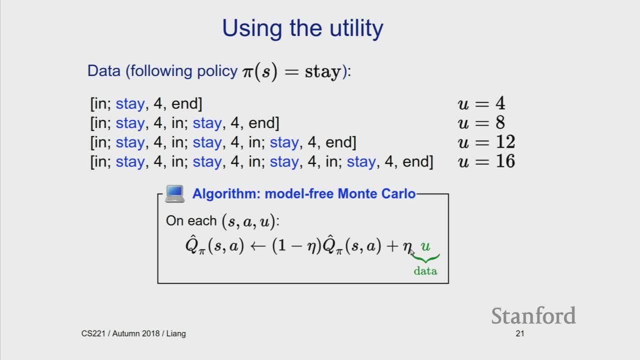 Um, and what Model-Free Monte Carlo is doing is it's using these utilities um to kind of update um towards uh, to update your q-pi, right. So in particular, like for example this: you're saying okay. 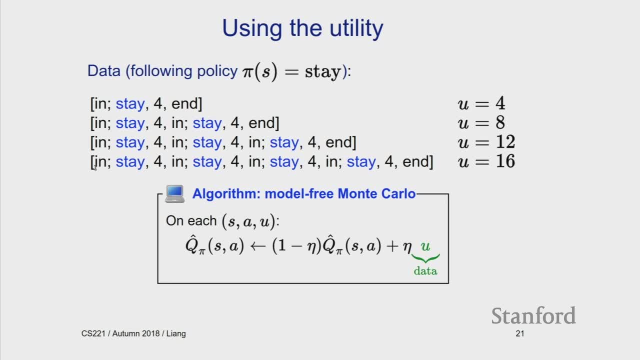 I'm in- I'm in. uh, the in-state and I, you know, take an action, stay when you know what will happen. Well, in this case, I got you know 16 and, uh, this case, I got 12.. 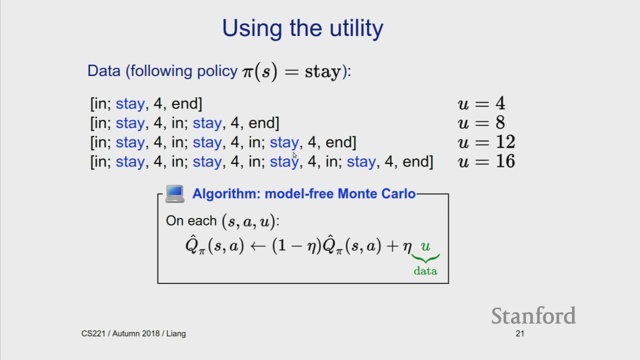 And notice that there's, you know, quite a bit of variance. So, on average, this actually does the right thing, right? So, um, just by definition, This is an unbiased, you know estimate If you do this a million times in average. 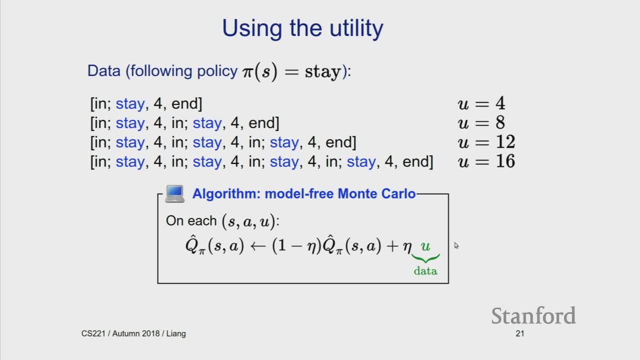 you're just gonna get the right value, which is uh 12 in this case, But the variance is huge. So if, for example, if you only do this a few times, you're not gonna get 12, you might get something you know slightly related. 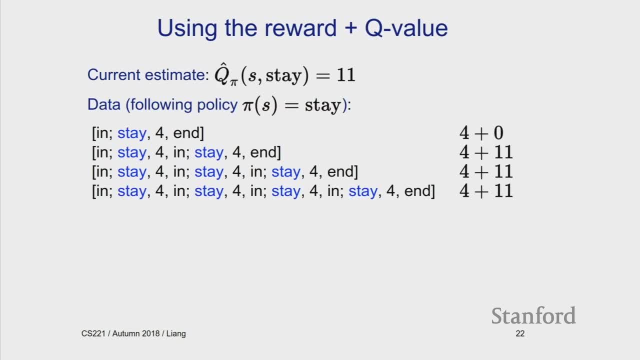 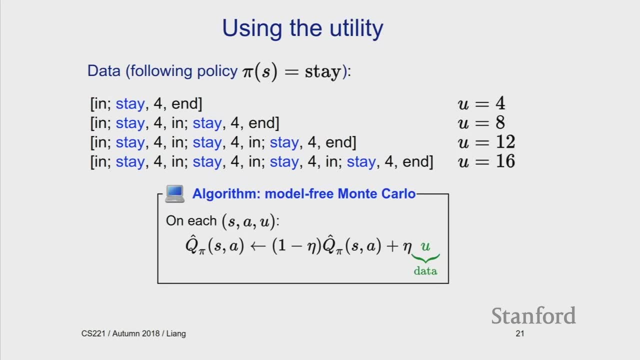 Um, so how can we kind of counteract uh this, uh this variance? So the key idea um behind what we're gonna call bootstrapping is is that, you know, we actually have, you know, some more information here. 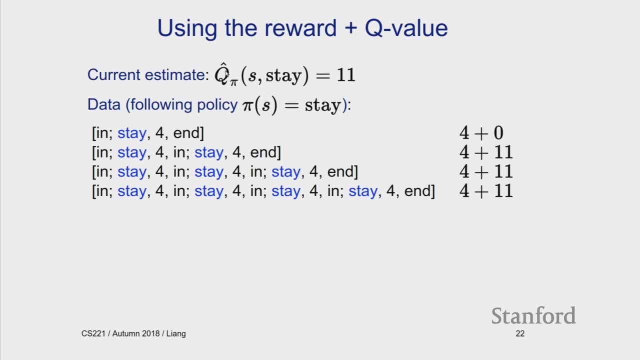 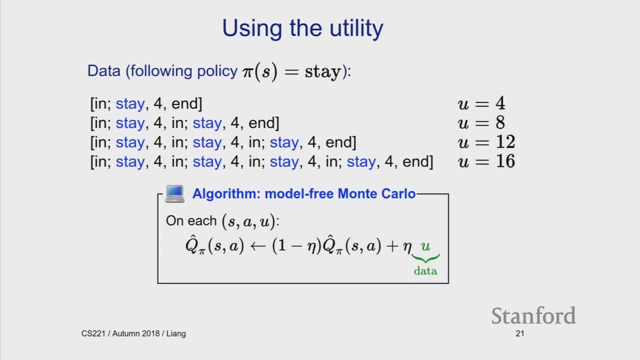 So we have this q-pi that we're estimating along the way, right? So so this view is saying, okay, we're trying to estimate q-pi, um, and then we're gonna try to basically regress it against you know, this data that we're seeing. 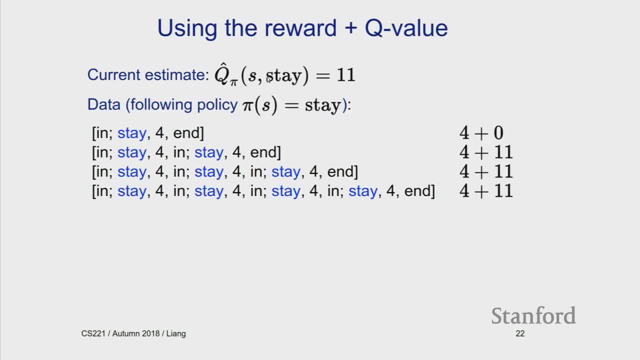 But you know, can we actually use q-pi itself to um help, you know, uh, reduce the variance? So so the idea here is: um, I'm going to look at all the places where I, you know, I start an in and I take stay. 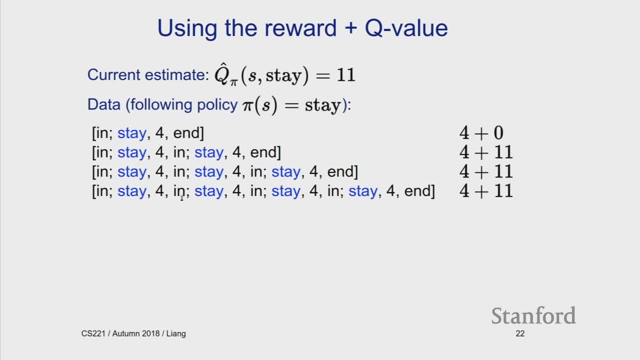 I get a 4, okay, So I'm gonna say I get a 4.. But then after that point I'm actually just going to substitute this 11 in okay. This is kind of weird, right, Because normally I would just see, okay, what would happen. 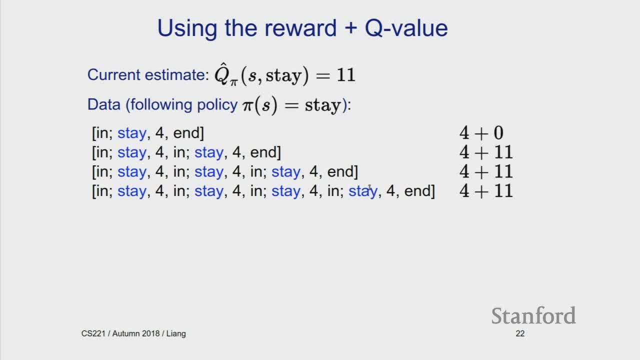 But what happens is kind of random. On average it's gonna be right, But you know, on any given case I might get, like you know, 24 or something And the. the hope here is that, by using my current estimate, 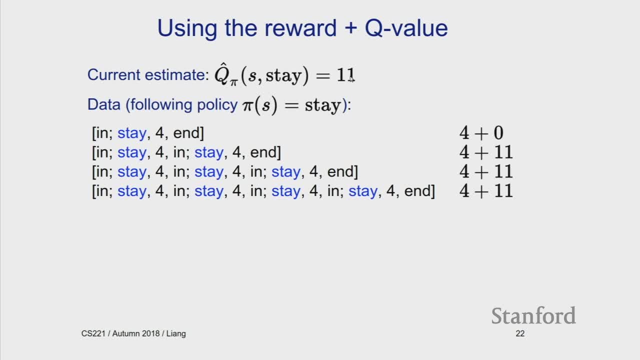 which isn't gonna be right, because if I were, if it were right, I would be done. But hopefully it's kind of somewhat right and that will you know be. you know better than using the, the kind of the raw, uh, rollout value. 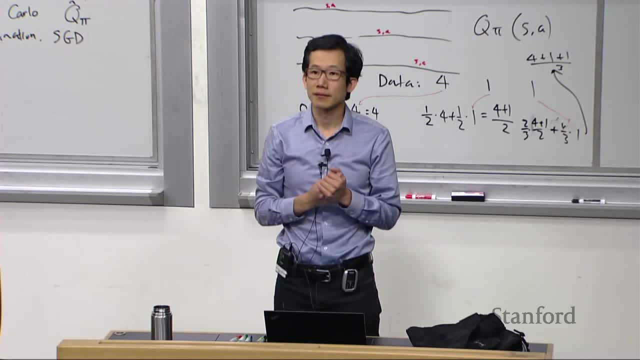 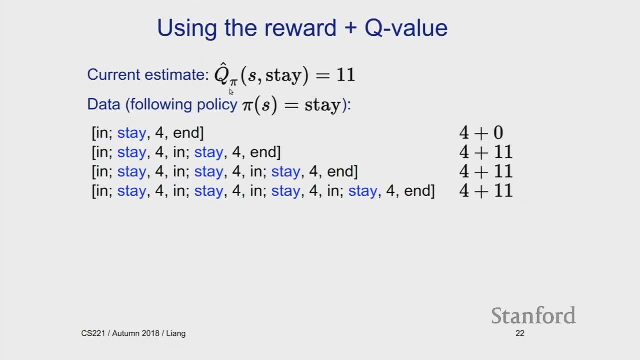 Yeah, question. So you, you would update your current estimate at the end of each each episode, correct? Uh, yeah, So the question is: would you update the current estimate after each episode? Yeah, So all of these algorithms? 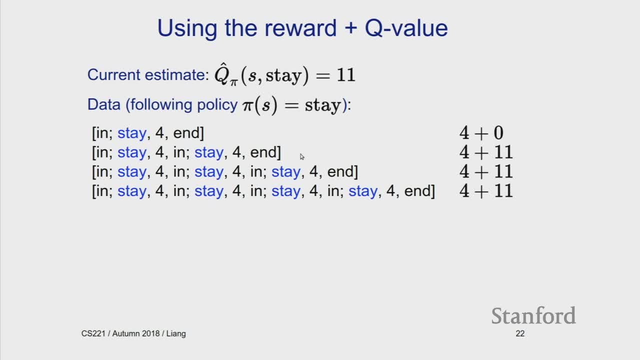 I haven't been explicit about it is that you see an episode, you update, um, after you see it and then you get a new episode, and so on. Yeah, Sometimes you would even update before you're done with the episode. Um, okay, 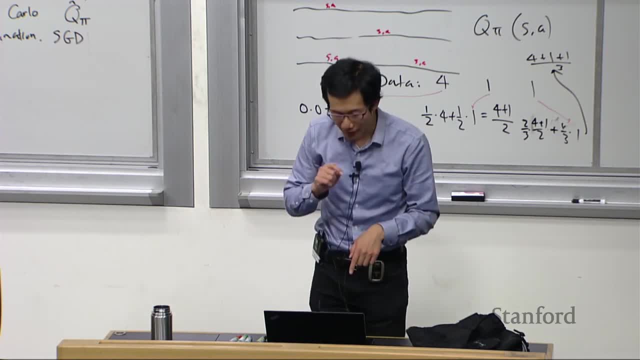 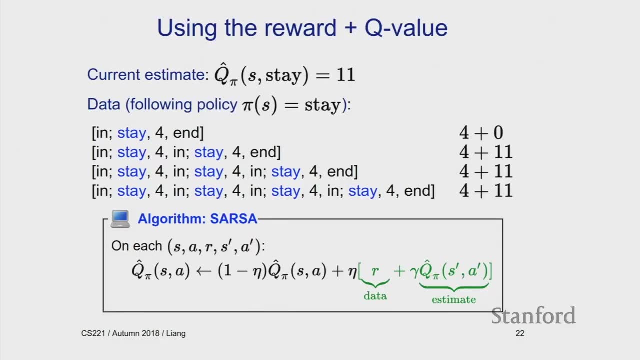 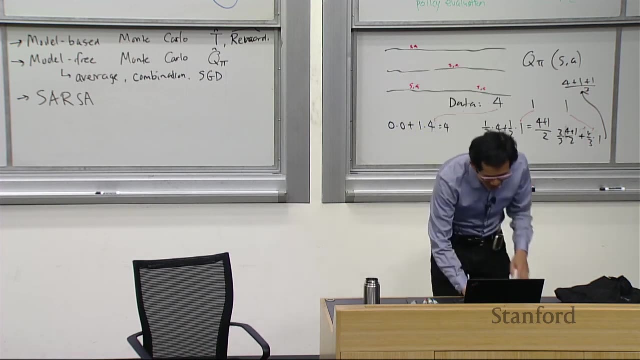 So, uh, let me show this. uh, what um this algorithm? So this is a new algorithm. It's called um SARSA. Does anyone know why it's called SARSA? Oh yeah, Right. So if you look at this, 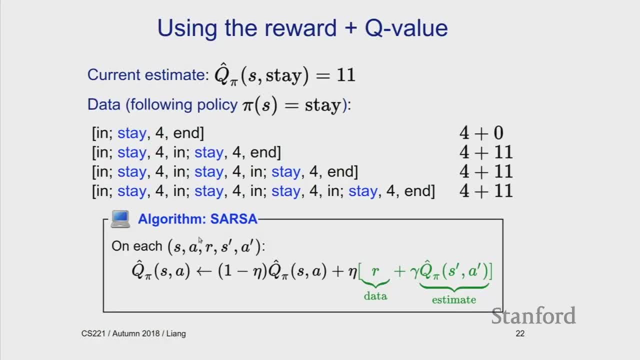 it spells SARSA, and that's literally the reason why it's called SARSA. Um, so what does this algorithm say? So you're in a state S, you took action A, you got a reward, and then you ended up in state S prime, and then you took another action, A prime. 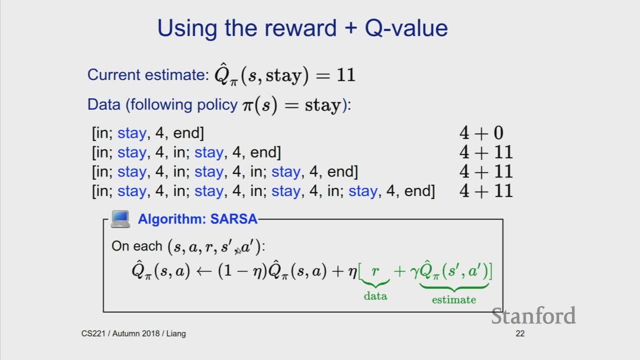 So, for every kind of quintuple that you see you're gonna perform this update. Okay, So what is this update doing? So this is the convex combination- uh, remember that we saw from before, um- where you take a part of the old value and then you 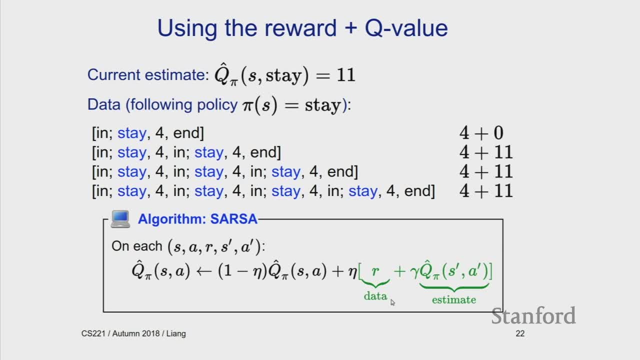 um, try to merge in with the new value. So what is the new value here? This is looking at just the immediate reward, not the full utility, just immediate reward, which is this? 4 here, And you're adding the discount. 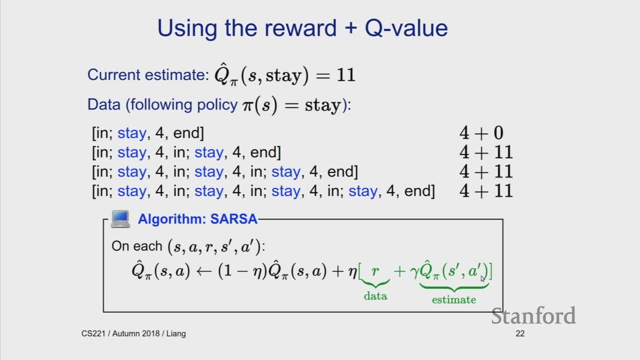 which is 1 for now, um of your S? um estimate. And remember what is the estimate trying to do? Estimate is trying to be the expectation of rewards that you will get in the future. So if this were actually Q? pi, 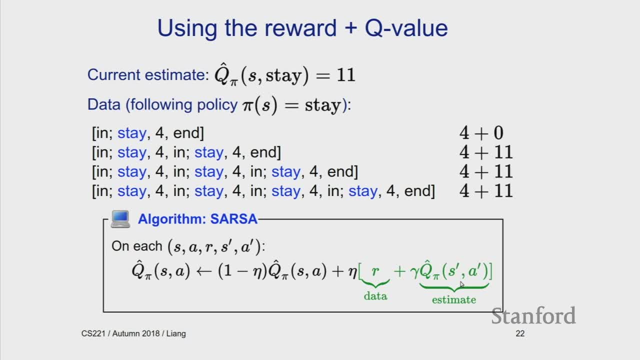 not Q pi hat, then this will actually just be strictly- you know better, because that would be um, just reducing the variance, Um. but you know, of course this is not exactly right. There is bias, so it's 11, not 12.. 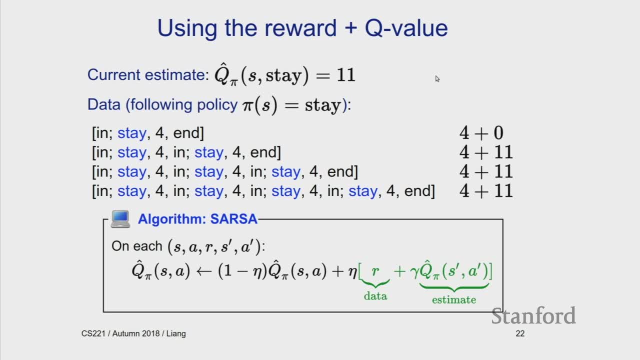 But the hope is that you know this is not, you know, biased by you know too much, Too much. Okay, So these would be the kind of the, the values that you will be updating, rather than, uh, these kind of raw values here. 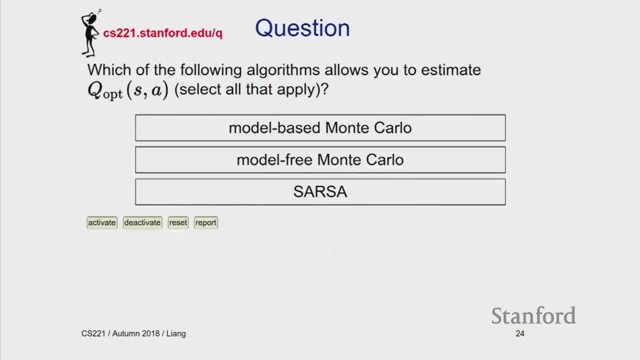 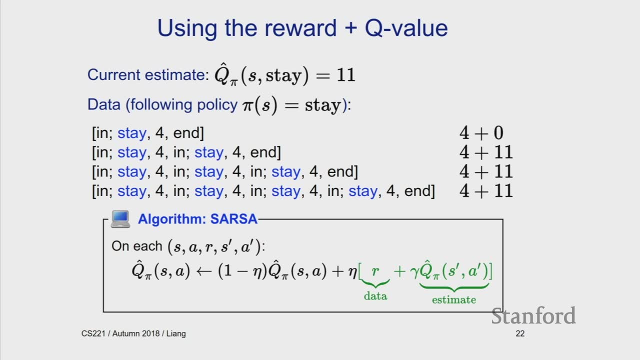 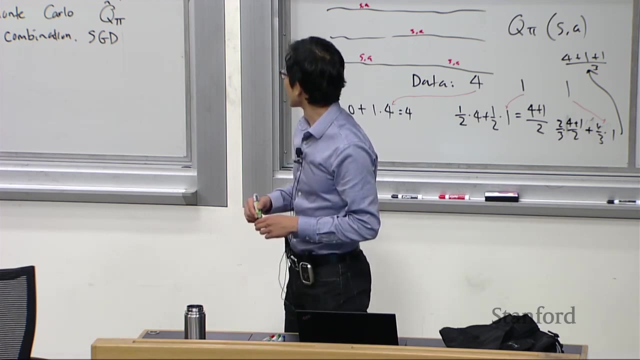 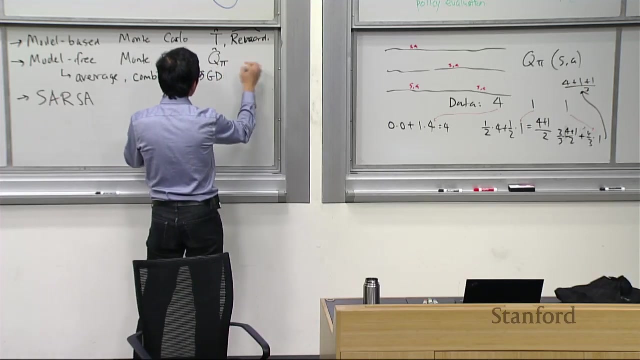 Okay, So just to kind of compare them. well, okay, Um, okay, Any questions about what SARSA is doing before I move on? Okay, So, maybe I'll write something. I mean to try to be helpful here. So Q pi- model-free Monte-Carlo estimates. Q pi based on U. 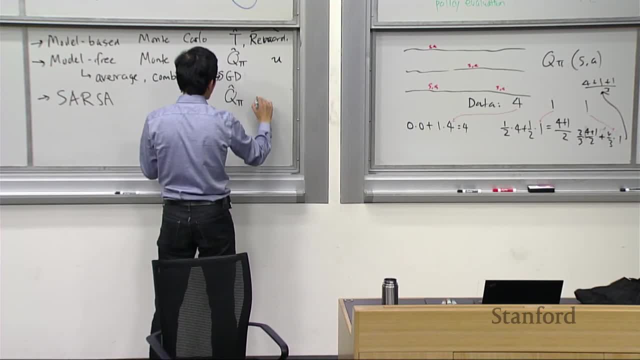 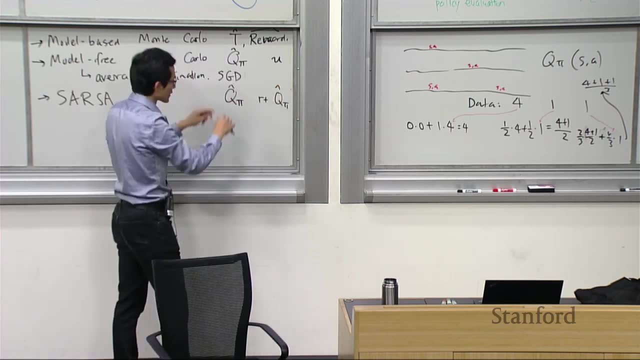 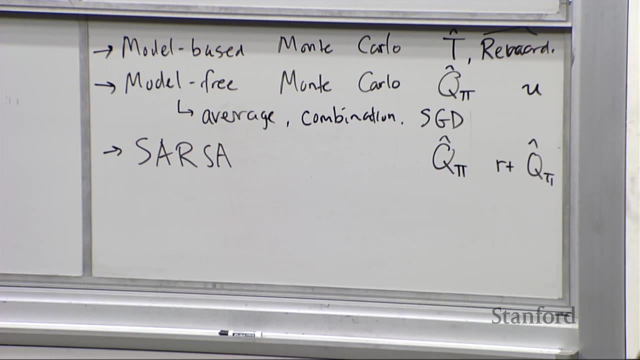 and SARSA is still Q pi hat, but it's based on reward plus uh, essentially Q pi hat. I mean, this is not like a valid expression, but hopefully it's some symbols that will evoke uh, the right memories, Um, okay. 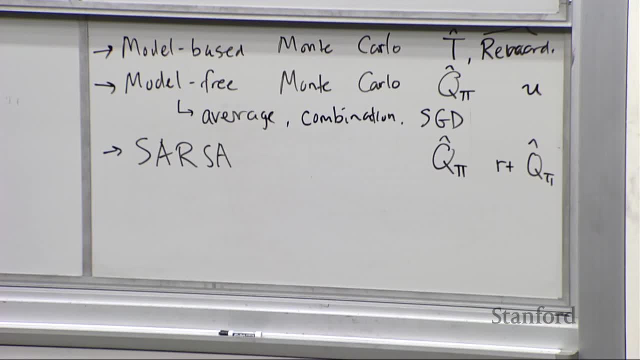 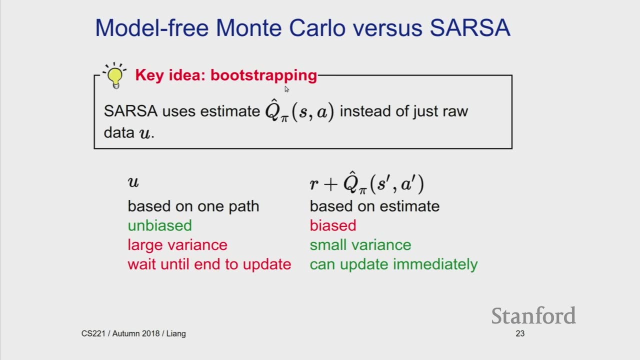 So let's discuss um the differences. So this, this: whenever people say kind of bootstrapping, um, in the context of reinforcement learning, this is kind of what they mean. is that, instead of using U as the prediction target? 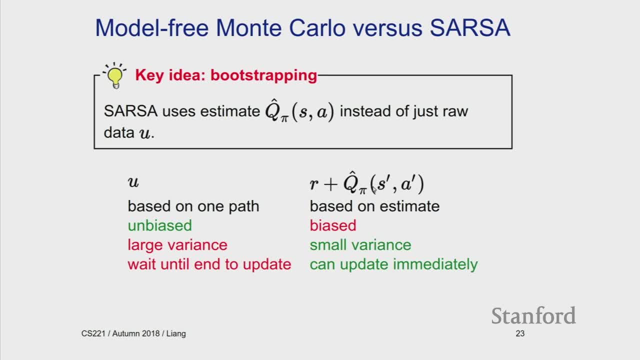 you're using R plus Q pi And this is kind of you're pulling up yourself from your bootstraps because you're trying to estimate Q pi but you don't know Q pi, but you're using Q pi to you know, estimate it. 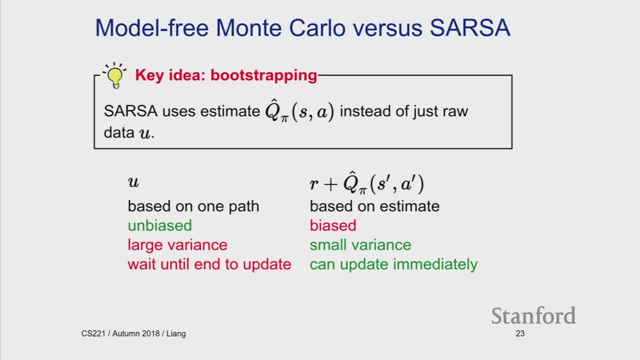 Okay, So U is based on one path, Um, in SARSA, your base on the estimate, which is based on all your previous kind of experiences, Which means that this is unbiased. uh, so, model-free, Monte-Carlo is biased, but SARSA is biased. 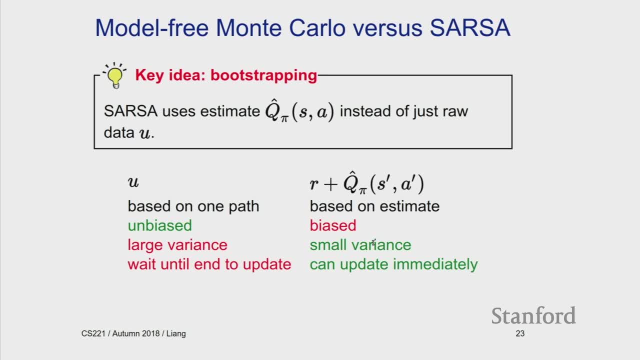 Monte-Carlo has large variance, SARSA has, you know, smaller variance, Um and one. I guess a consequence of the way the algorithm is set up is that model-free Monte-Carlo, you have to kind of roll out. 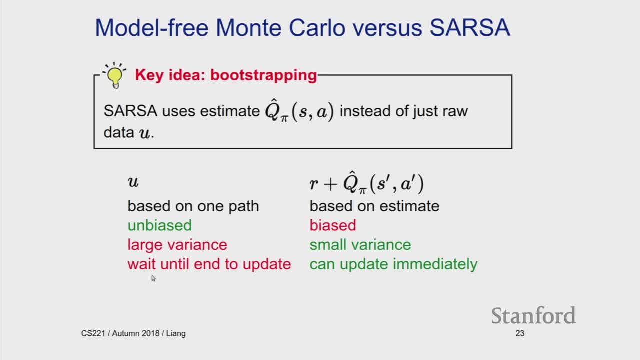 the entire game. Basically, play the game or the MDP until you you reach the terminal state and then you can- now you have your U to update, Whereas uh, SARSA when- or any sort of bootstrapping algorithm. 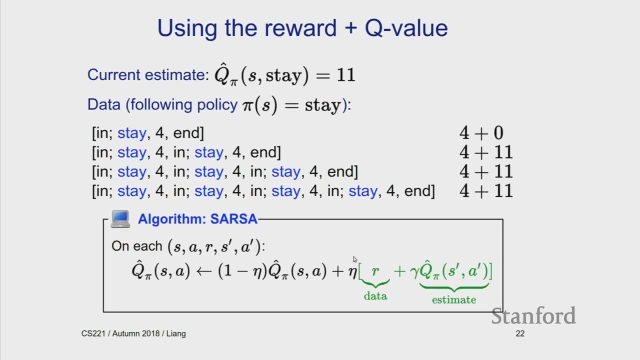 you can just immediately update, because all you need to do is you need to see, uh, this like a very local window of S-A-R-S-A, and then you can just update And that can happen, kind of you know anywhere. You don't have to wait until the very end to get the value. 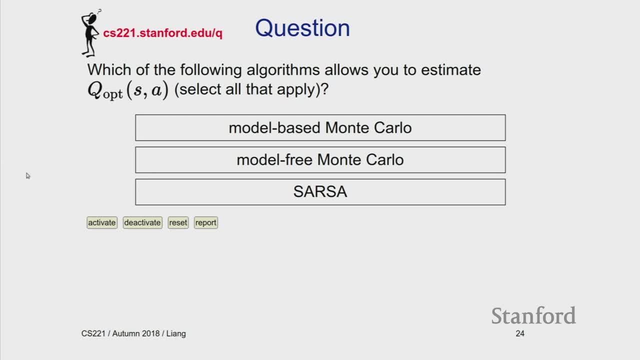 Okay. So, just as a quick sanity check, um, which of the following algorithms allows you to estimate? uh, QOpt, Okay. So. model-based Monte Carlo? uh, model-free Monte Carlo. or SARSA, Okay. So I'll give you maybe 10 seconds to ponder this. 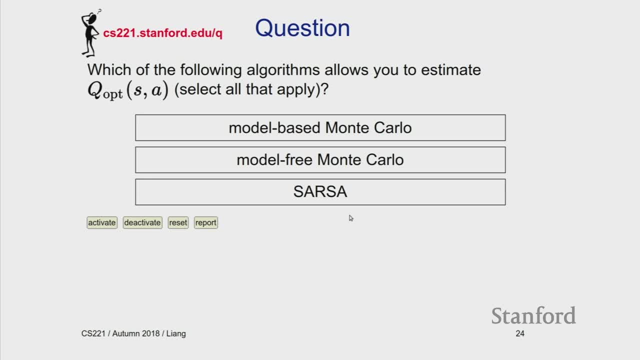 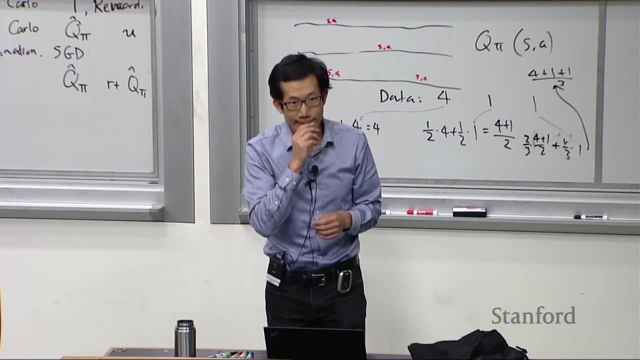 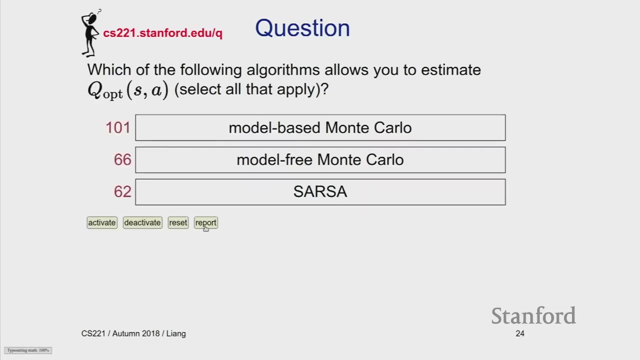 Okay, How many of you more need more time? Okay, Let's uh get a report. I think I didn't reset it from last year, So this is- includes- last year's uh participants. Um, so Model-based Monte Carlo. 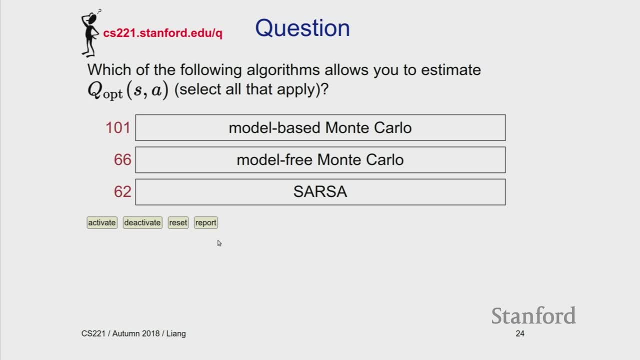 um allows you to get QoP right Because once you have the MDP right. But once you have the line, you'll find solo queue opt agreed Because once you have the MDP don't right, Because once you have the MDP right. 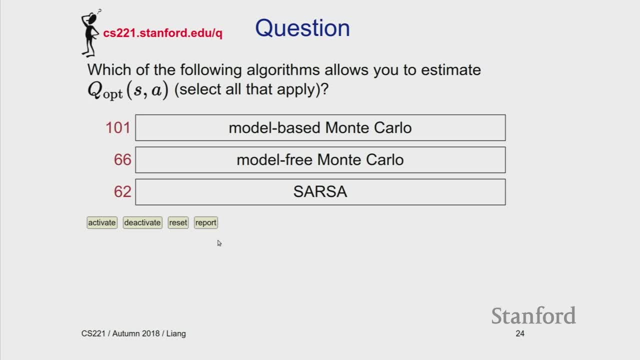 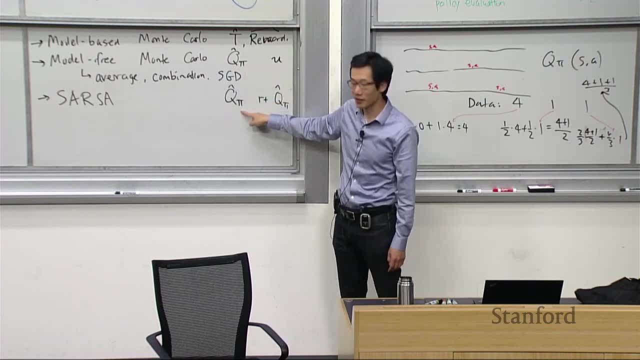 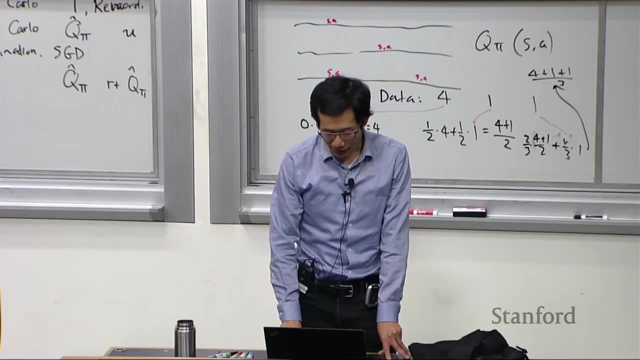 you can get whatever you want. you can get QOpt Model-free. Monte Carlo: um estimates QPy- it doesn't estimate QOpt. And um SARSA also estimates QPy, but doesn't estimate QOpt. Okay, All right. 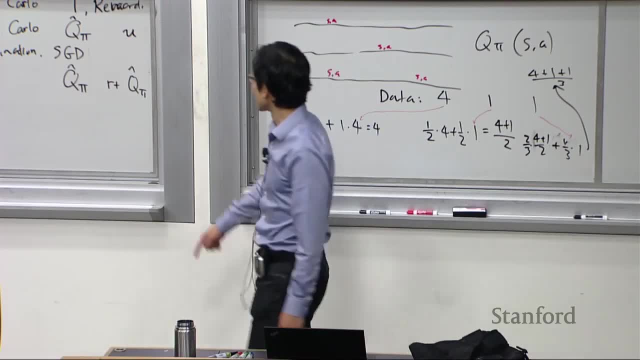 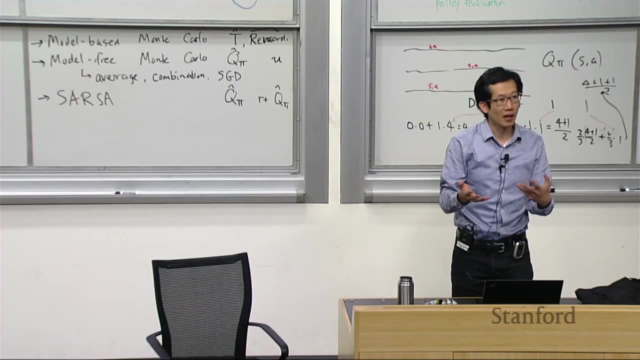 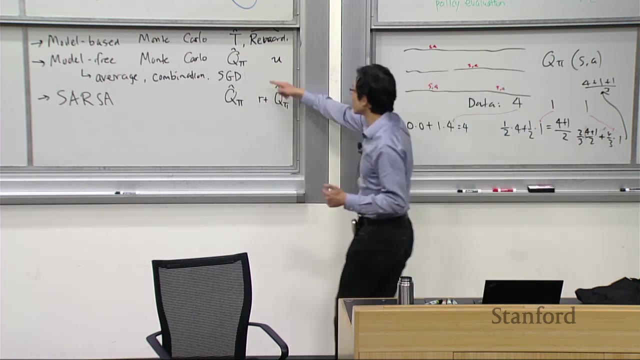 So so that's a kind of a problem, Like I mean, these algorithms are fine for, uh, estimating the value of a, a policy, Um, but you really want the optimal policy right? In fact, these can be used to improve the policy as well, because you 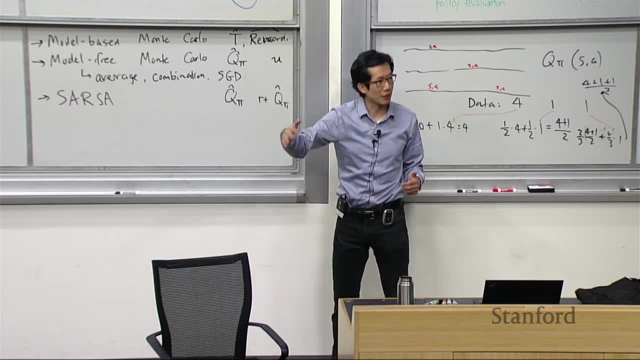 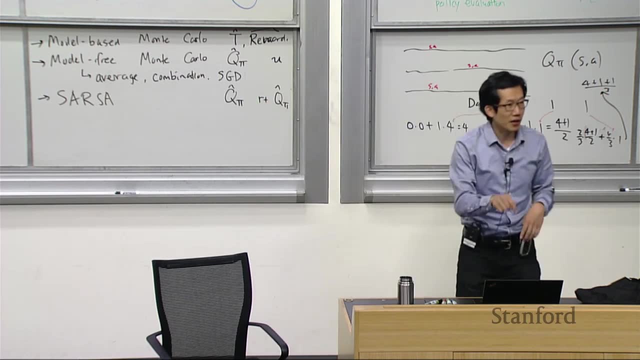 can um do something called policy improvement, which I didn't talk about. Once you have the Q values, you can define the new policy based on the Q values, Um, but there's actually a kind of a more direct way to do this. 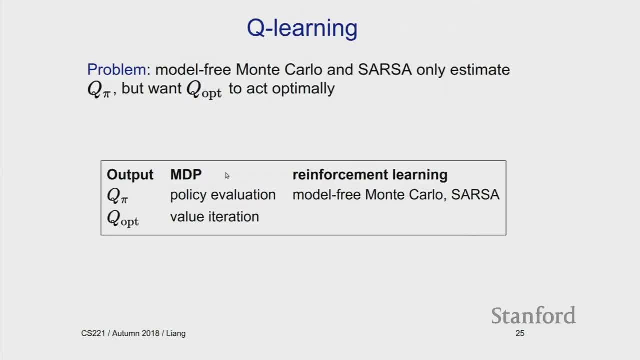 Okay So so here's the, the kind of the way mental framework you should have in your head. So there's two values: QPy and QOpt. So in MDPs we saw that policy evaluation allows you to get QPy. 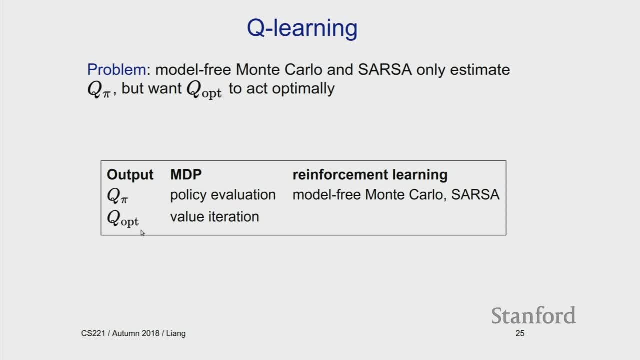 value iteration allows you to get QOpt, And now we're doing reinforcement learning And we saw model-free Monte Carlo and SARSA allow you to get QPy, And now we need- I'm going to show you- a new algorithm called Q-learning that allows you to get QOpt. 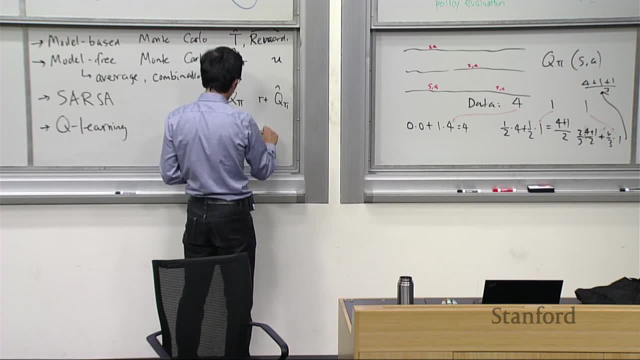 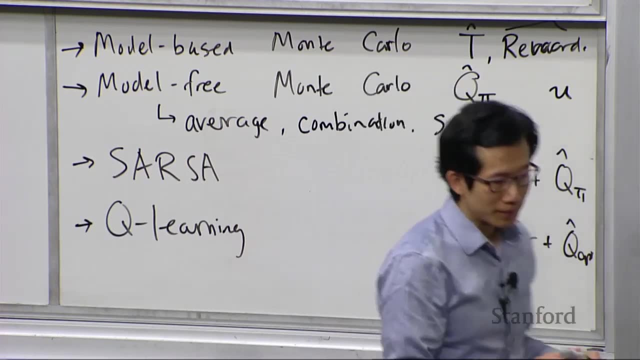 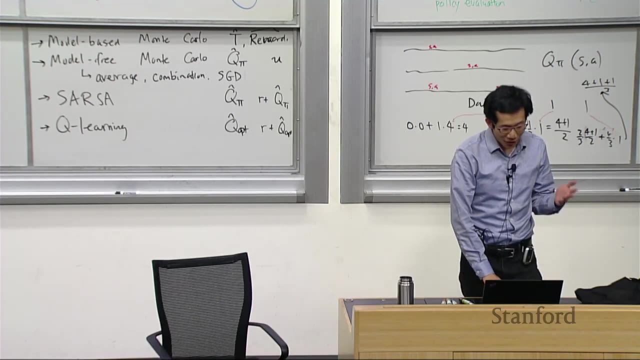 So this gives you QOpt And it's based on reward- uh plus uh, QOpt, kind of Okay. So this is going to be very similar to SARSA. Uh, it's only going to differ by essentially. 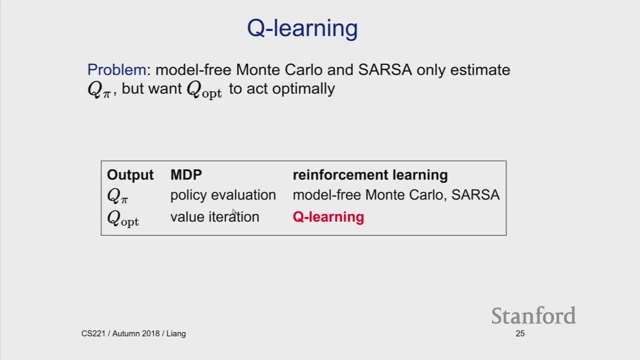 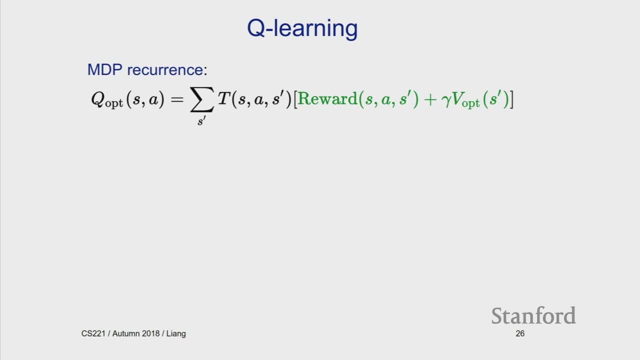 as you might guess, the same difference between policy evaluation and value iteration. Okay, So it's helpful to go back to kind of the MDP recurrences. So even though MDP recurrences can only apply when you know the MDP for deriving, 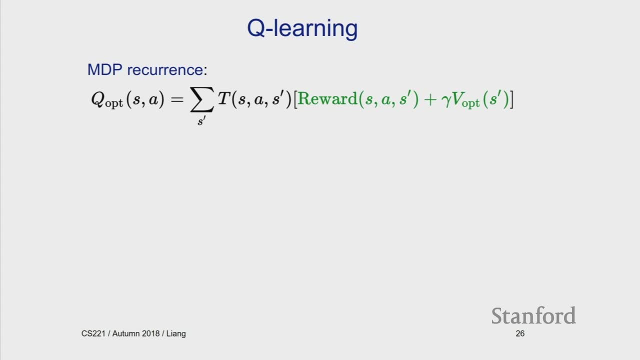 reinforcing learning algorithms- um it's- they can kind of give you inspiration for the, the actual algorithm. Okay, So remember QOpt. what is QOpt? QOpt is considering all possible successors, the probability immediate reward plus, uh, future um returns. 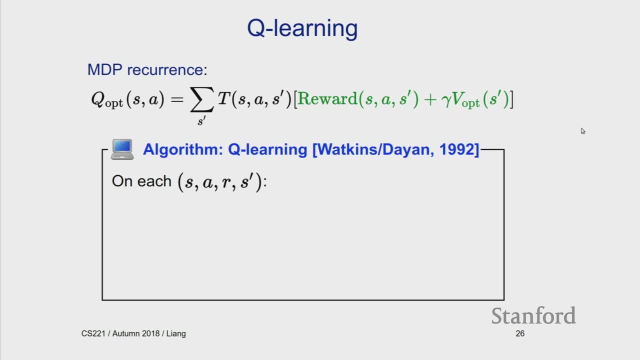 Okay, So the Q-learning. is this actually really kind of clever idea? Um and it's- it could also be called SARS, SARS, I guess, um, but maybe you don't want to call it that- Um, And what it does is as follows. 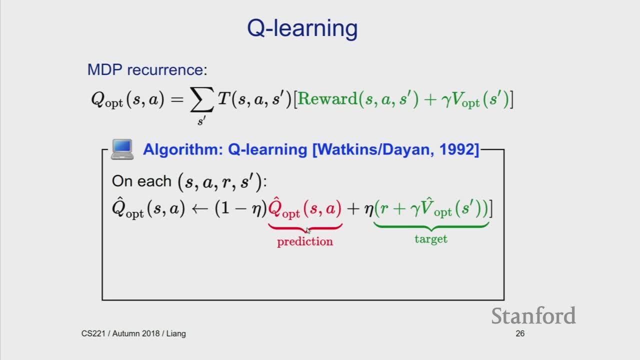 So this is- has the same form- the convex combination of the old uh value, um and the- the new value, right? So what is the new value? Um? so if you look at QOpt, QOpt is uh. 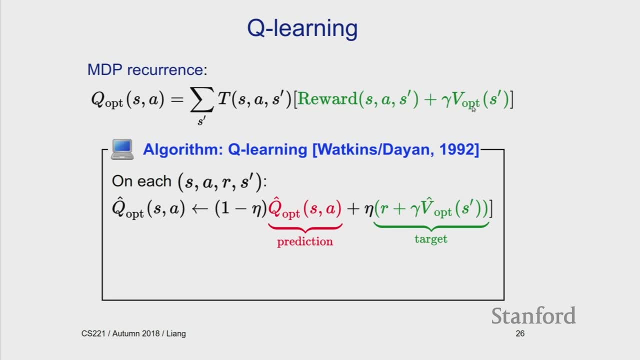 looking at different successors- reward plus V-Opt. What we're gonna do is: well, we don't have all- we're not gonna be able to sum of all successors because we're in our reinforcement learning setting and we only saw one particular successor. 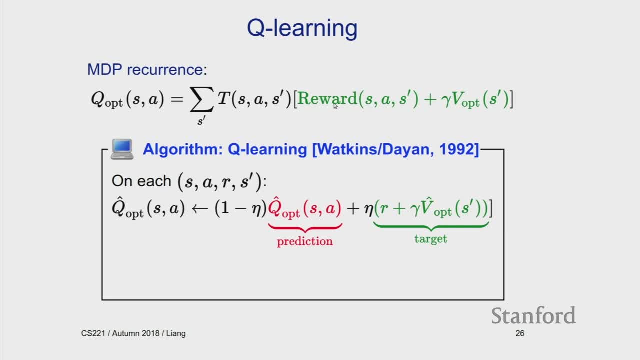 So let's just use that successor. So, on that successor, we're gonna get the reward. So R is a stand-in for the actual reward. uh, I mean, is the stand-in for the reward? that f- reward function, And then you have Gamma times. 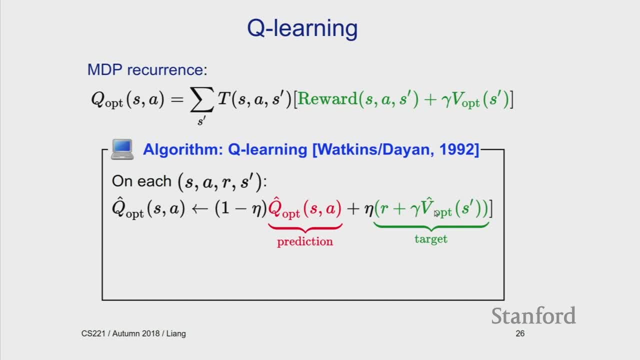 and then V-Opt. I am going to replace it with um, our estimate of of what V-Opt is And what should the estimate of V-Opt be. So what relates V-Opt to QOpt? Yeah, The A that maximizes QOpt, that should be V-Opt. 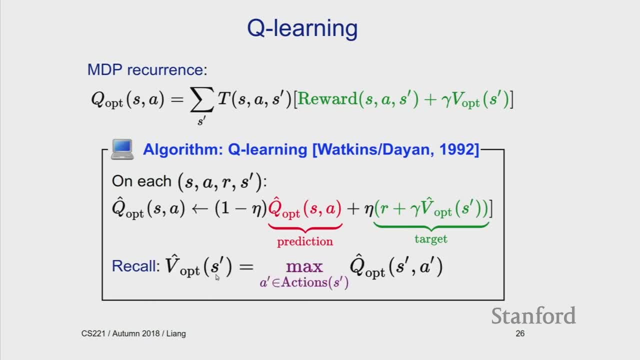 Yeah, exactly So you-. if you define V-Opt to be the max overall possible actions of QOpt of S in that particular action, then this is uh V-Opt, right. So Q is saying I'm at a chance node. 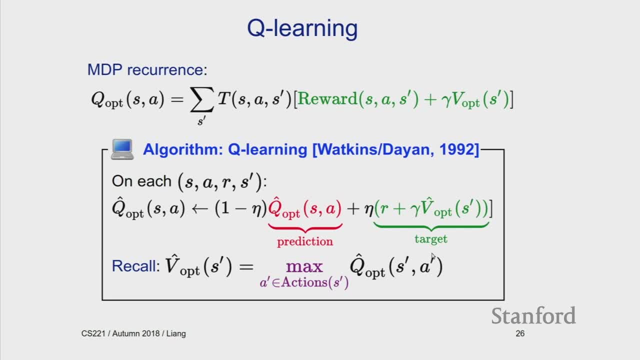 um, how much- what is the optimal utility I can get, provided I took an action. Clearly the best thing to do if you're at a state is just choose the action that gives you the maximum of uh Q value that you get into. 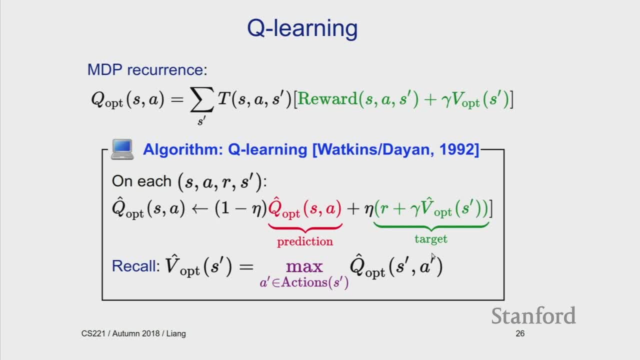 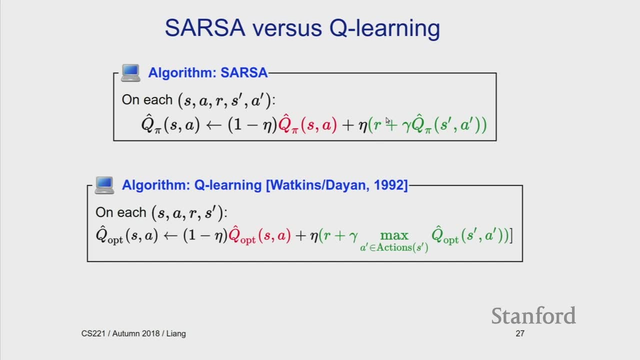 Okay, So that- that's just, you know, Q learning, So let's put it side-by-side with SARSA. Okay So, SARSA. um, these two are very similar, right? So SARSA, remember, updates against R plus QPi. 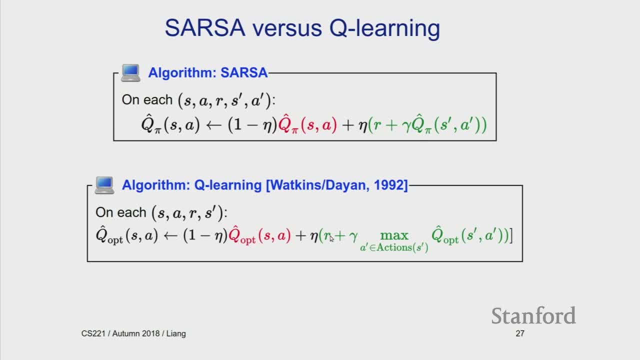 Okay. So SARSA, um, these two are very similar, right? So, SARSA, remember updates against R plus QPi, And now we're updating against R plus this max over QOpt. Okay, And you can see that SARSA requires knowing what action I'm gonna take next. 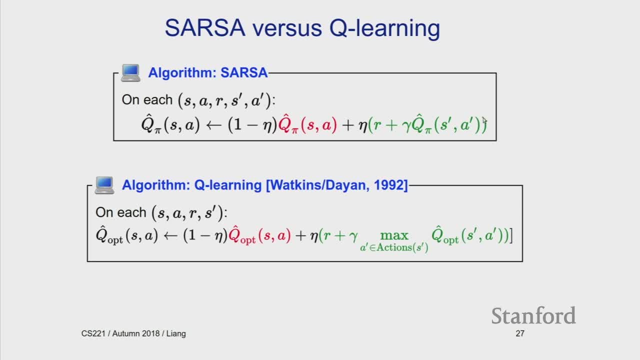 um, kind of a one-step look ahead: A prime and it plugs it into here, whereas Q learning, it doesn't matter what uh A you took, because I'm go- just gonna take the one that maximizes right. So you can see why SARSA dep- is. 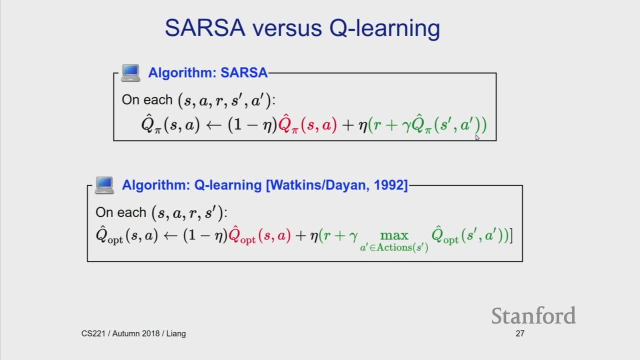 estimating the value of the policy, because you know what A prime uh shows up here is, you know a function of a policy And here, um, I'm kind of insulated from that because I'm just taking the maximum overall actions. 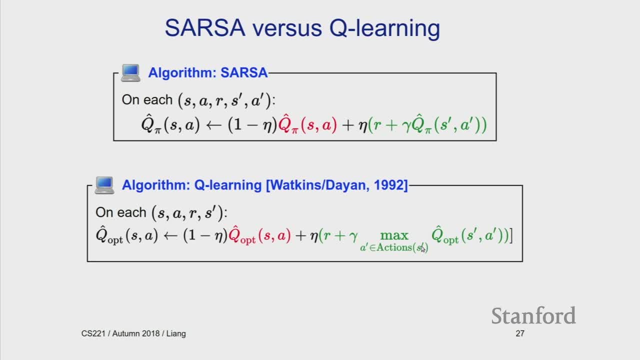 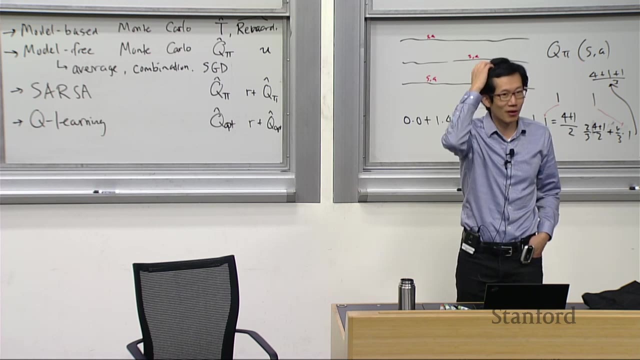 This is the same intuition as for value iteration versus policy evaluation. Okay, I'll pause here Any questions: Q learning versus SARSA. So is Q learning on policy? Is Q learning on policy or off policy? It's off policy because I'm following whatever policy I'm following. 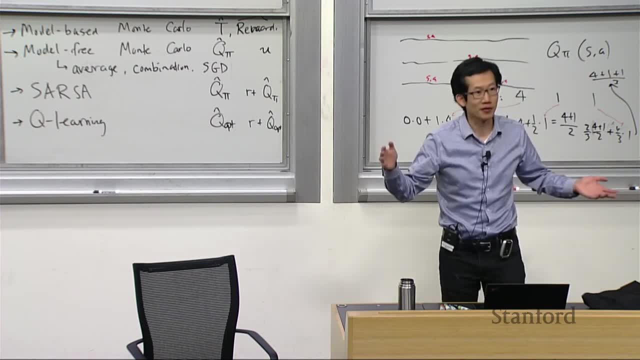 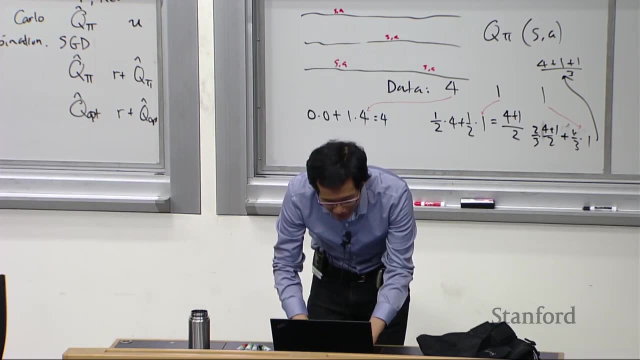 and I get to estimate the value of the optimal policy, which is probably not the one I'm following, at least in the beginning. Okay, So let's look at the example here. So here's SARSA, and run it for 1,000 iterations. 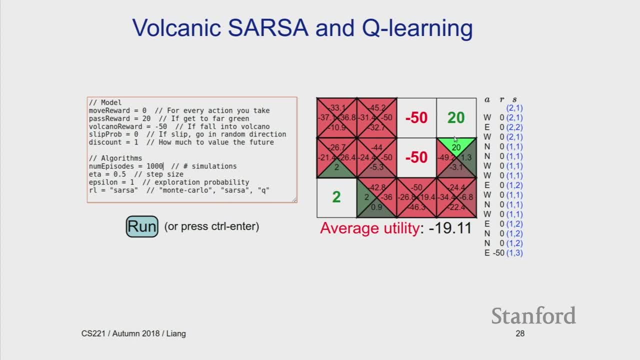 And like model-free Monte Carlo, um this, um, I'm uh estimating that the average- the average utility I'm getting is minus 20.. And, in particular, the values I'm getting are all very negative because this is Q pi. 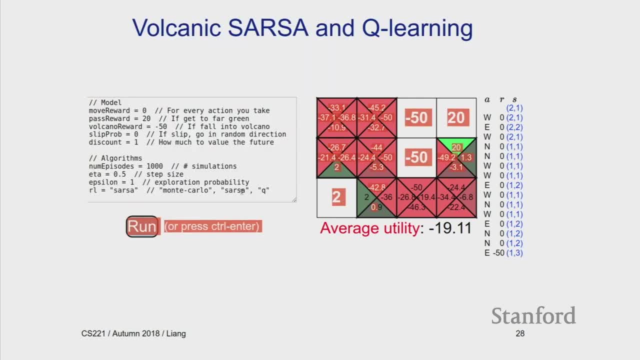 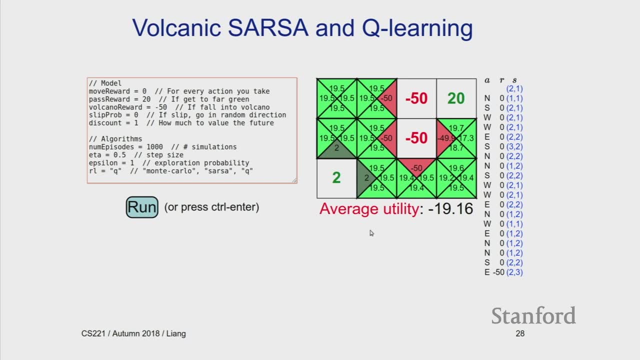 This is a policy I'm following, which is the random policy. Um, if I replace this with Q, what happens? So first notice that the average utility is still minus 19, because I actually haven't changed my exploration policy. I'm still doing random exploration. 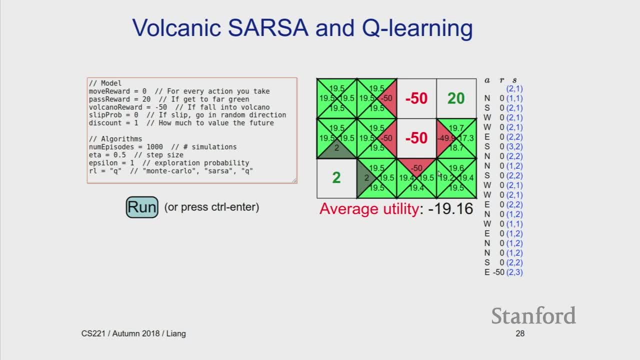 Um, well, yeah, Okay, I'm still doing random exploration, But notice that the value, the Q-opt values, are all around, you know, 20, right, And this is because the optimal policy, remember, is just to- and this is a slip- probability of zero. 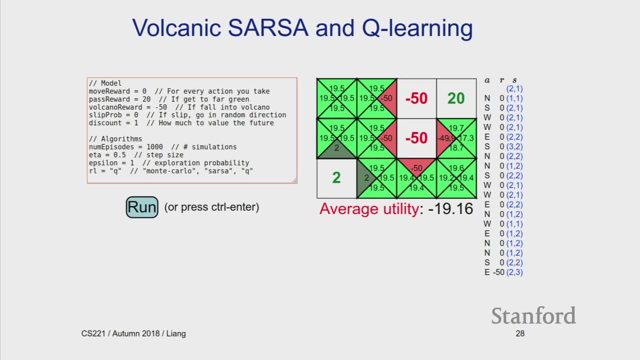 So optimal policy is just to go down here and get your 20, okay, And Q- and I guess it's kind of interesting that Q-learning. I'm just blindly following the policy running, you know, off- off the cliff into the volcano all the time. 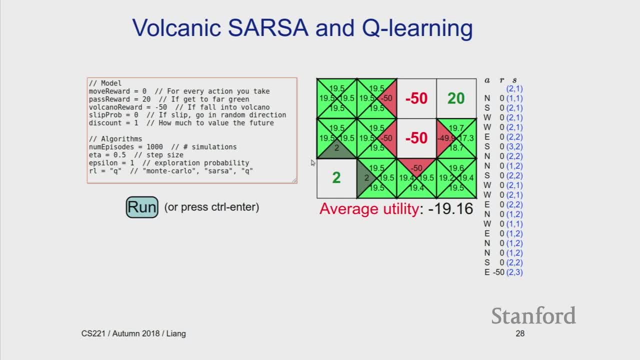 But you know, I'm learning something, um, and I'm learning how to uh behave optimally even though I'm not behaving optimally, And that's uh the kind of uh hallmark of off-policy learning. 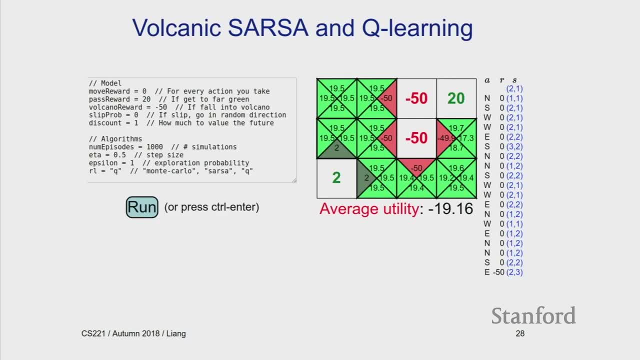 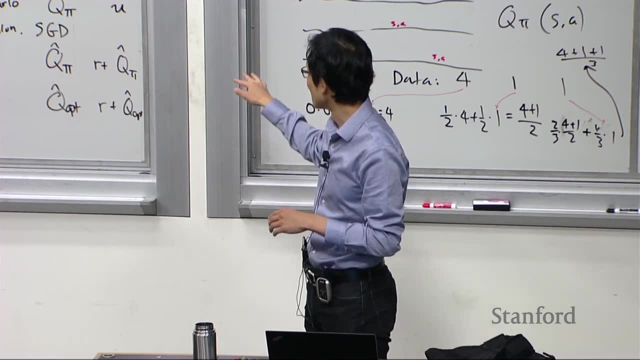 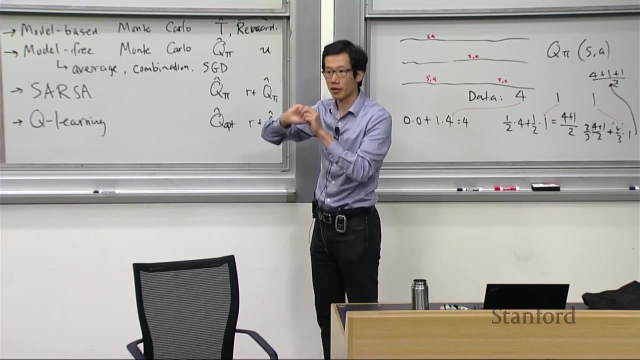 Okay, So any questions about these four algorithms? So, model-based Monte Carlo estimate- MDP. model-free Monte Carlo um estimate, uh, the Q value of MDP, this policy based on um, the actual returns that you get. 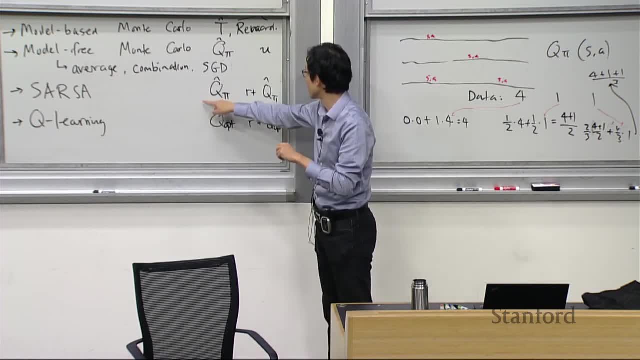 the actual sum of the uh rewards. SARSA is bootstrapping, estimating the same thing, but with kind of a one-step look ahead, And Q-learning is like SARSA, except for I'm estimating the optimal instead of um a fixed policy pipe. Yeah, 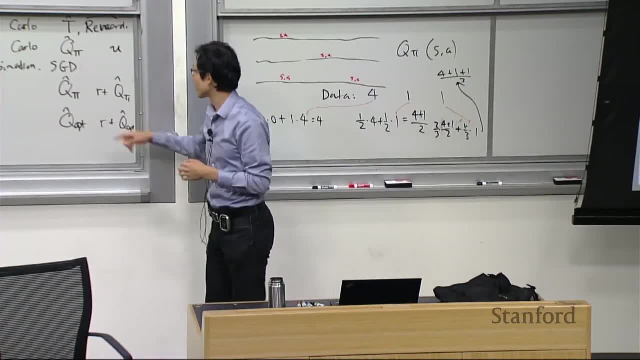 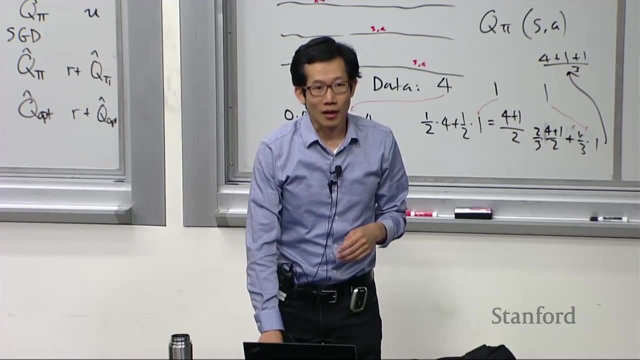 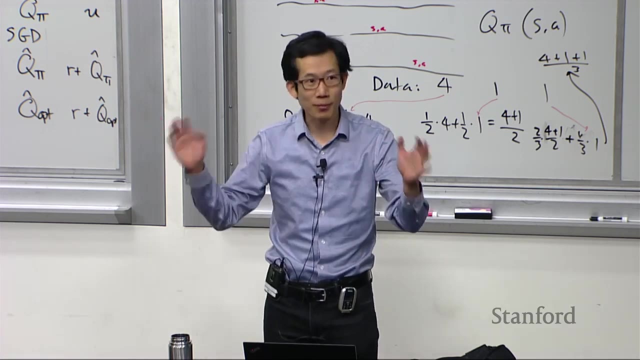 Is SARSA on policy or off policy? SARSA is on policy because I'm estimating Q-Pi. All right, Okay, So now let's talk about covering the unknown. So these are the algorithms. So at this point, if I just hand you some data, 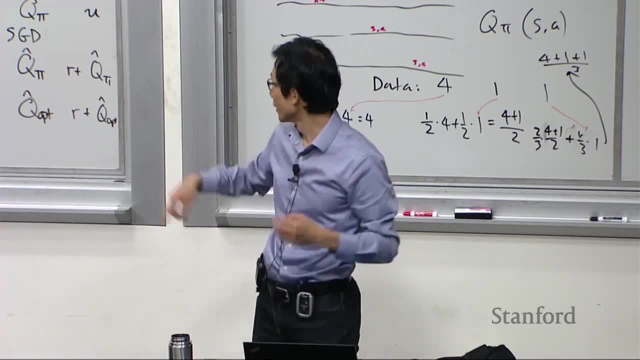 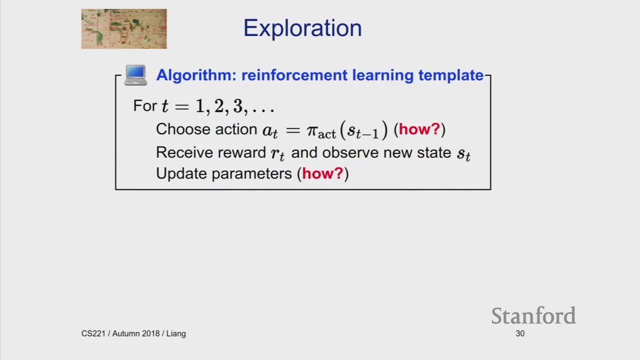 um, if I told you, here's a fixed policy, here's some data, you can actually estimate all these quantities. Um, but now there's a question of exploration, which we saw was really important, because if you don't even even see all the states, 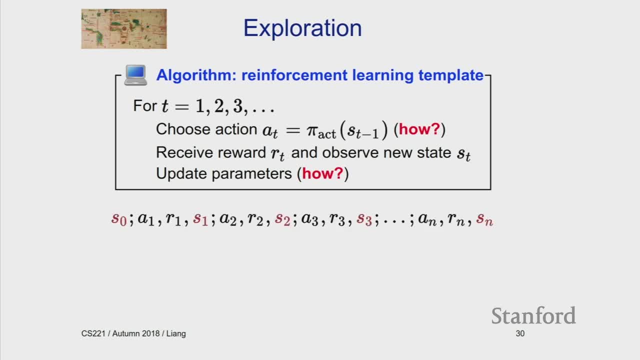 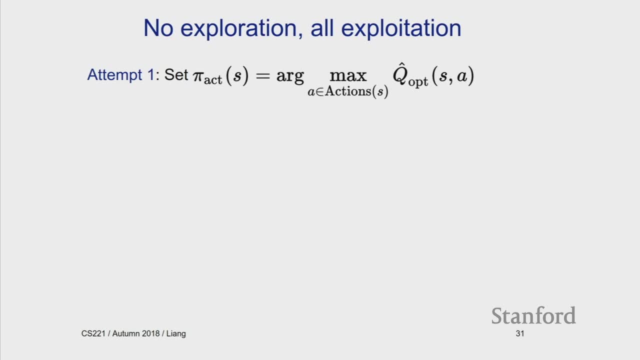 how can you possibly act optimally? So, um, so which exploration policy should you use? So here are kind of two extremes. So the first extreme is: um, let's just set the exploration policy So. so imagine we're doing Q-learning now. 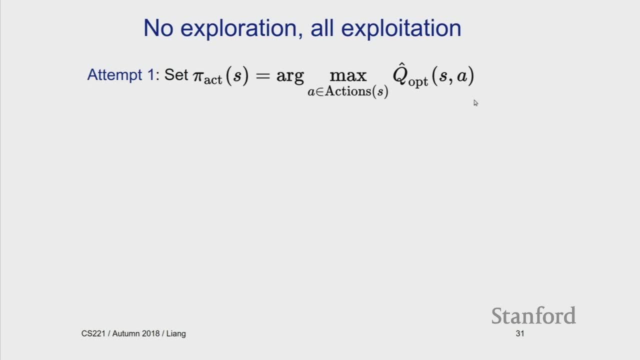 So you have this Q-opt estimate. So it's not the true Q-opt, but you have an estimate of Q-opt. Um, the naive thing to do is just take a use that Q-opt, figure out which action is best and just always do that action. 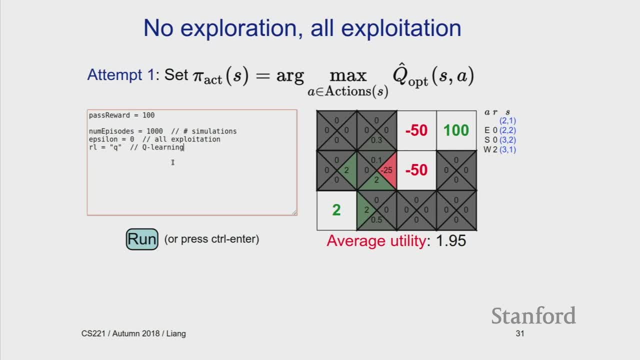 Okay. So what happens when you do this is: um, you uh, don't do very well. So why don't you do very well? Because, initially, well, you explore randomly and soon you, you find the 2.. And once you've found the 2, you say: 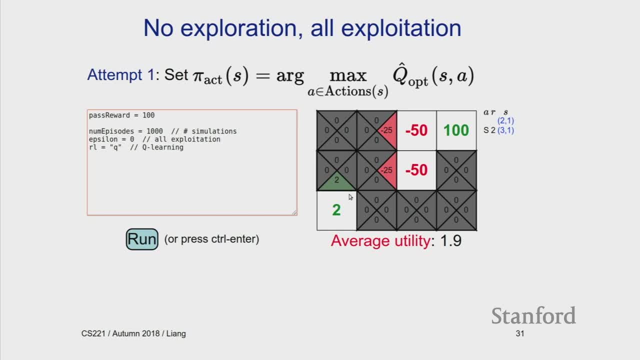 ah well, 2 is better than 0, 0, 0.. So I'm just gonna keep on going down to the 2, which is, you know, all exploitation, no exploration, Right? So you don't realize that there's all this other stuff over here. 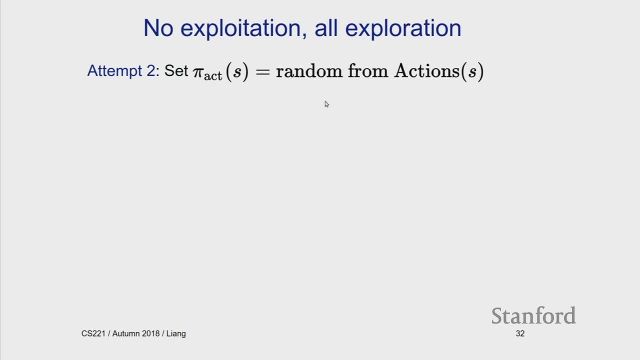 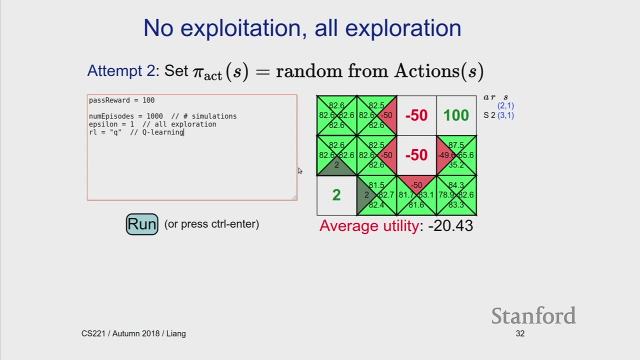 Um. so in the other direction, we have no exploitation, all exploration. Um, here, uh, you kind of have the opposite setup where I'm I'm running Q-learning right. So, as we saw before, I'm actually able to estimate the. 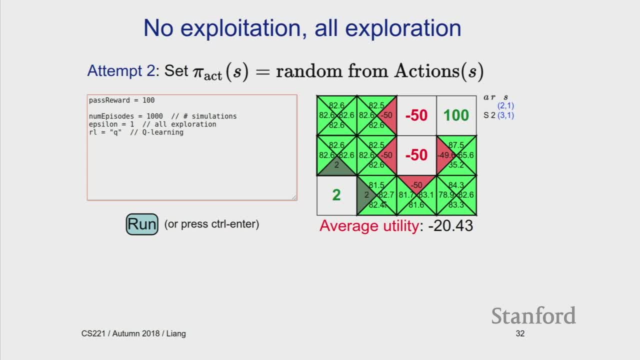 the, the Q-opt values. So I learn a lot, But the average utility, which is the actual utility I'm getting by playing this game, is pretty bad. In particular, it's the, the utility you get from, just you know, moving randomly. 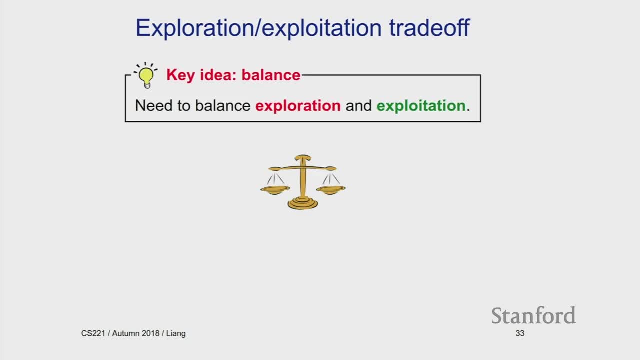 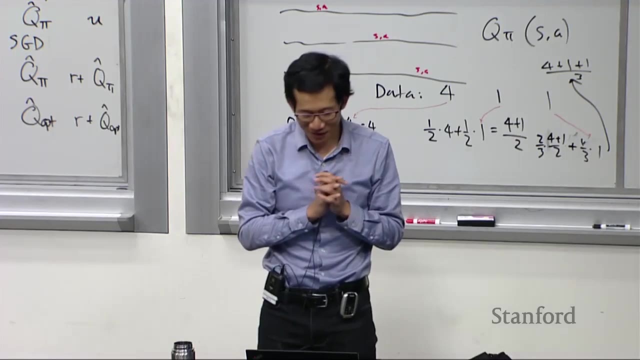 So kind of what you really want to do is uh, balance, you know, exploration, exploitation. So just kind of a kind of a side or a commentary is that I really feel reinforcement learning kind of captures uh life pretty well. 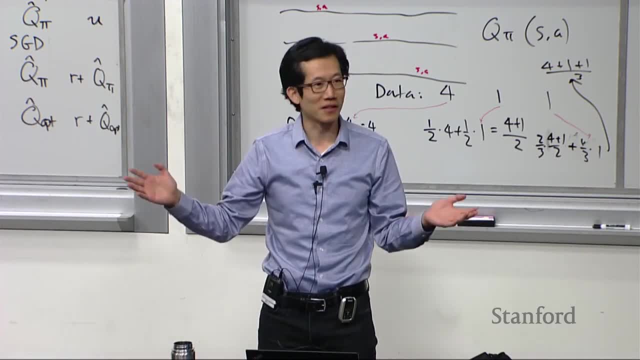 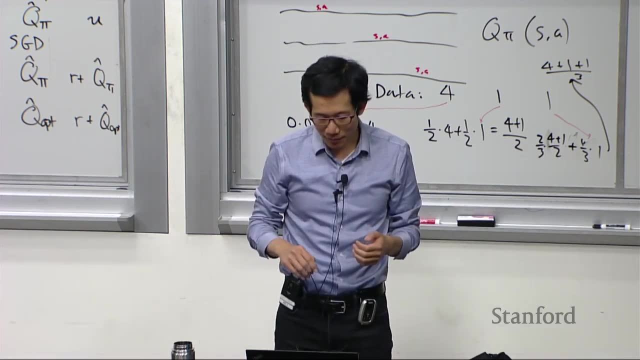 Um, because in life there's- you know, you don't know what's going on- Um, you want to get rewards. you know you want to do well Um and um, but at the same time time you have to um. 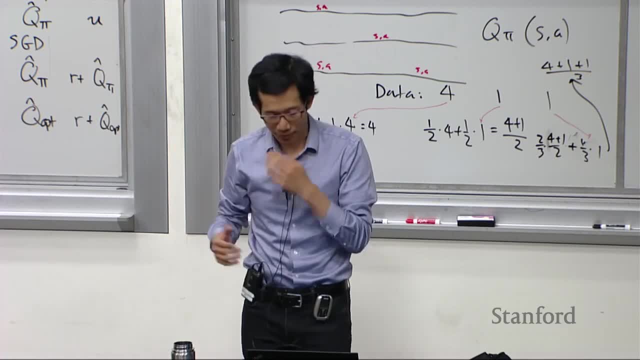 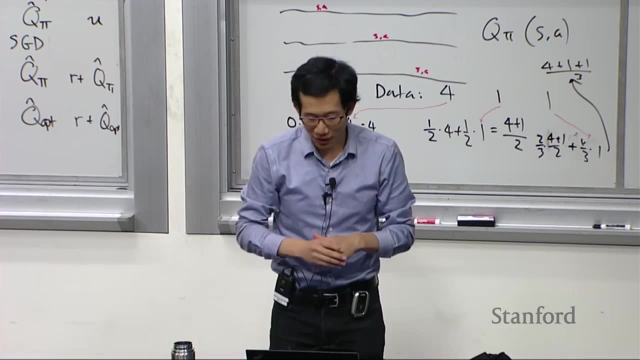 kind of learn about how the world works so that you can kind of improve your, your policy. So if you think about going to the restaurants or finding it the shortest path, better way to get to um, to school or to work or in research, even when you're. 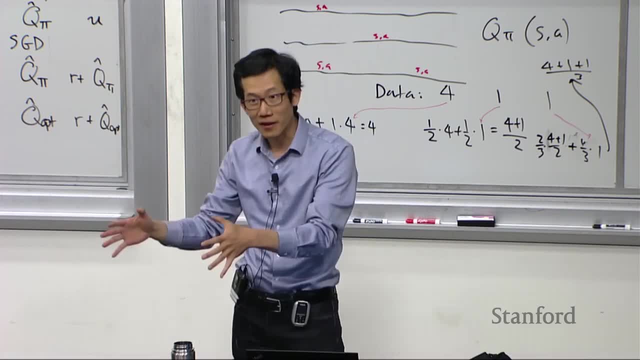 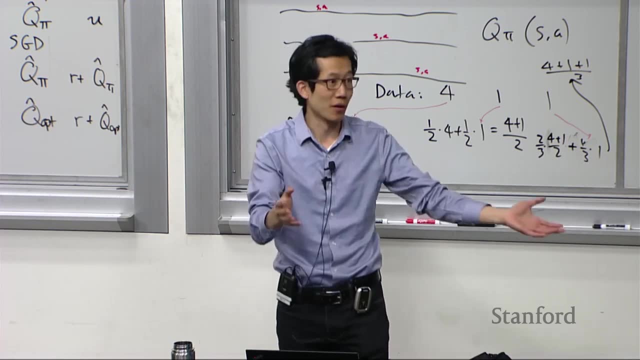 you're trying to figure out um a problem. You can work on the thing that you know how to do and will definitely work. Or, you know, do you try to do something new in hopes of you learning something, but maybe it won't get you as high reward. 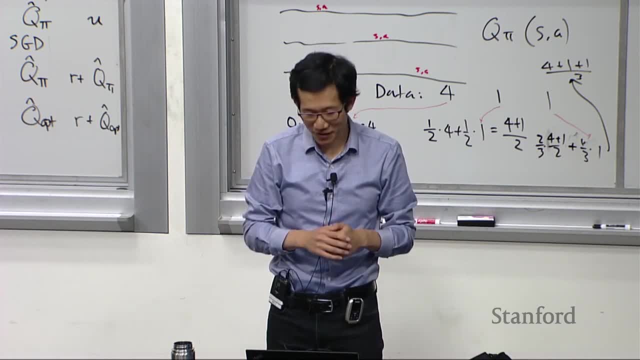 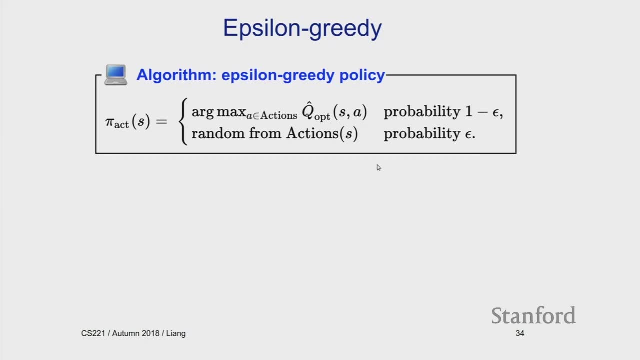 So, um, hopefully, reinforcement learning is, um, I know it's kind of a metaphor for life in many ways. Um okay, So uh, back to concrete stuff. Um, so here is one way you can balance um exploration and exploitation right. 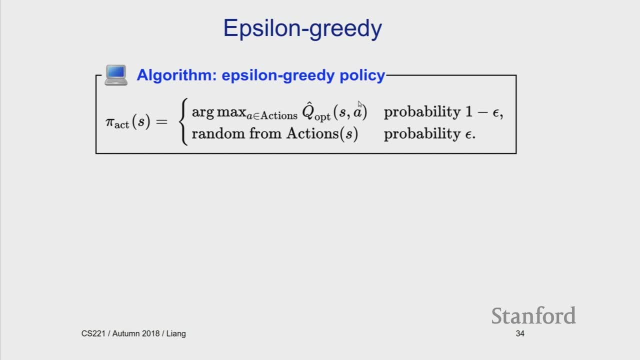 So it's called the epsilon greedy policy, And this assumes that you're doing something like Q-learning. So you have these Q-op values And the idea is that you know, with probability of 1 minus epsilon, where epsilon is. you know. 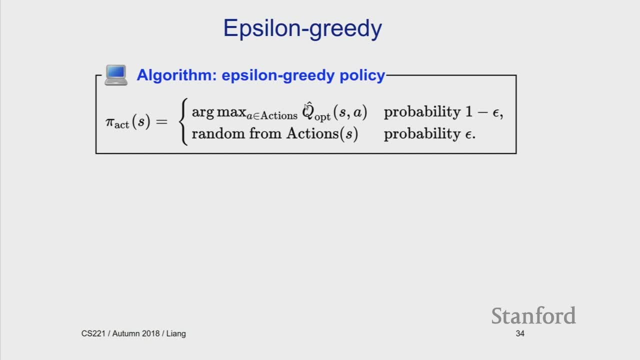 let's say like 0.1, you're just gonna give uh exploit. You're just gonna do- give you- give it all you- you have Um and then um. once in a while you're just gonna do something random, okay. 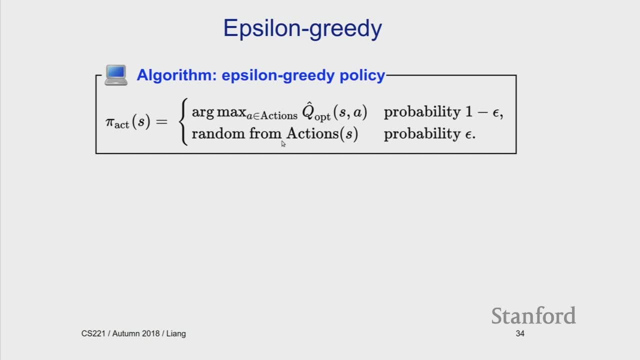 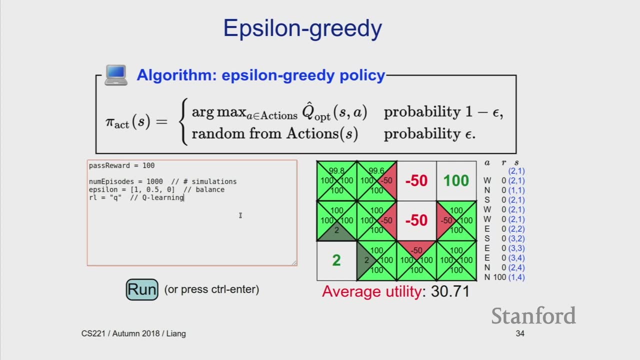 So this is actually not a bad policy to act in life. So once in a while, maybe you should just do something random and kind of see what happens. Um, so if you do this, um what- what do you get? Okay, So what I've done here is: 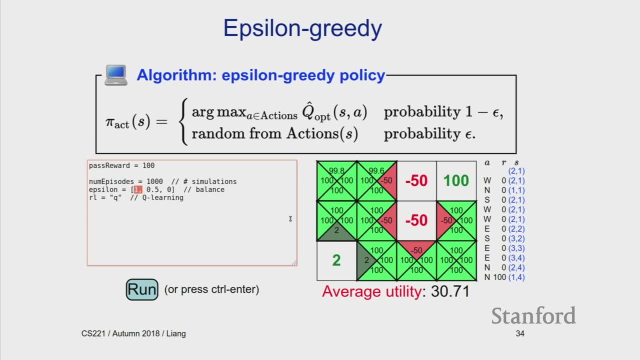 um, I've set epsilon to be starting with 1.. So 1 is, uh, all exploration. And then I'm going to change the value um a third of that Of the way into 0.5.. And then I'm gonna a two-thirds of the way. 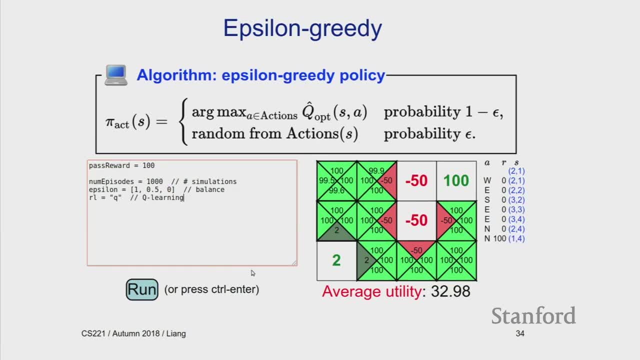 I'm gonna change it to 0,, okay. So if I do this, then I actually estimate the values, uh, really really well, um, and also I get utility, which is, you know, pretty good. you know, 32, um, okay. 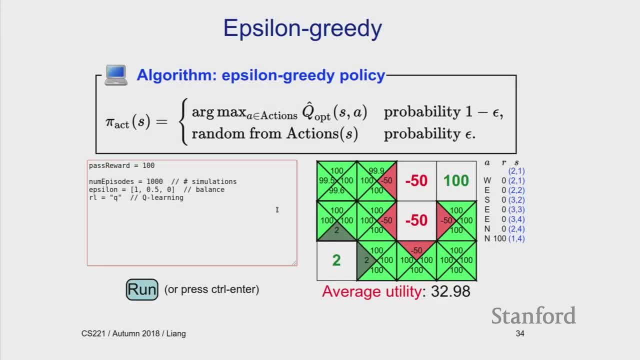 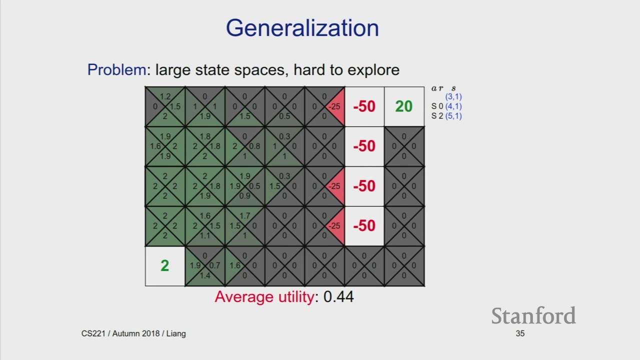 And this is also kind of something that happens. uh, um, as you get older, you tend to um, explore less and exploit more. um, it just happens. Um, okay, All right, So that was exploration. So let's put some stuff on the board here. 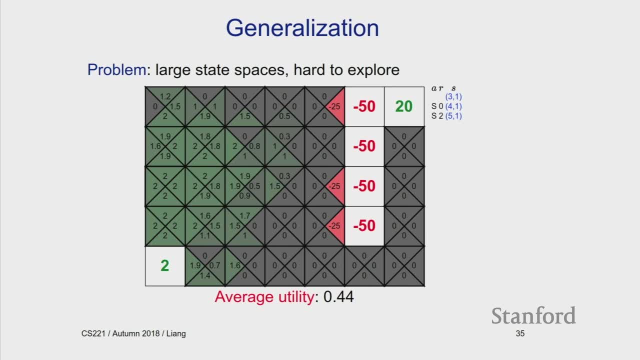 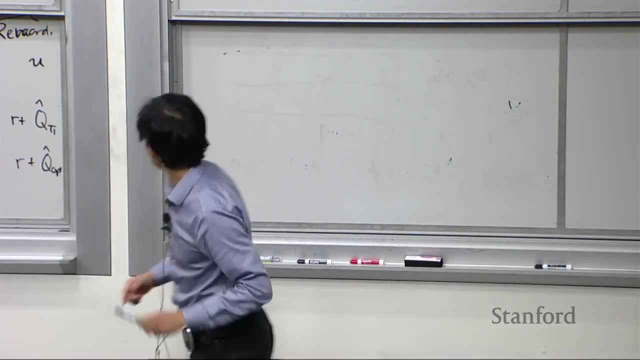 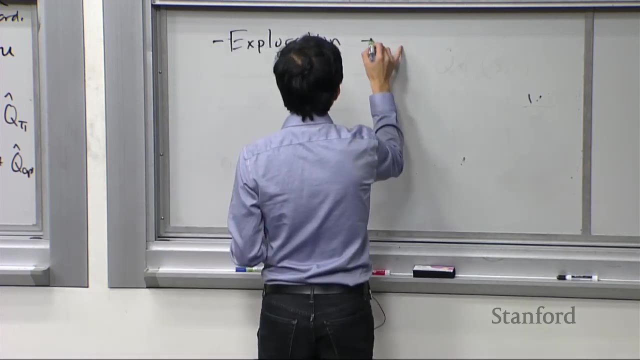 Um, do I need this anymore? Maybe I don't need this, Okay, Um, okay, So covering the unknown. So we talked about, you know, exploration, um, you know epsilon, greedy, Um, and there's other ways to do this. 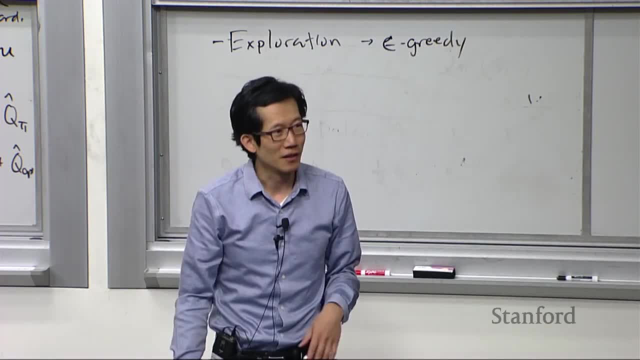 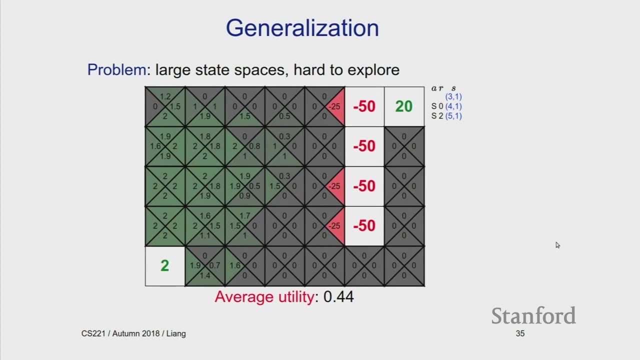 Um, epsilon greedy is just kind of the simplest thing that actually, you know, works remarkably, you know well, um, even in the state of our systems. Um, so the other problem now I'm gonna talk about is, you know, generalization. 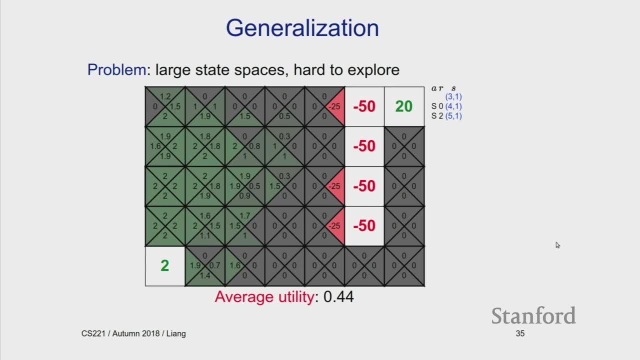 Um, so remember when we said exploration, well, if you don't see a particular state, then you don't know what to do with this. I mean, you think about for a moment that's kind of unreasonable, because you know in life, 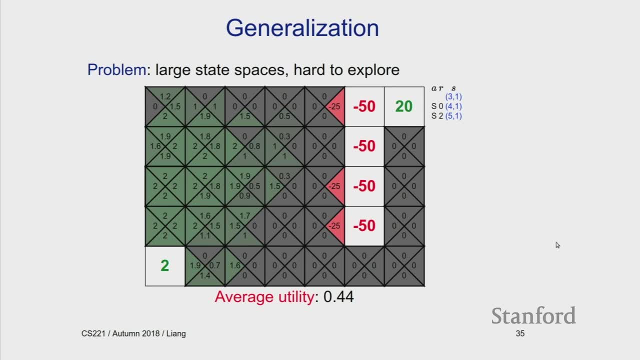 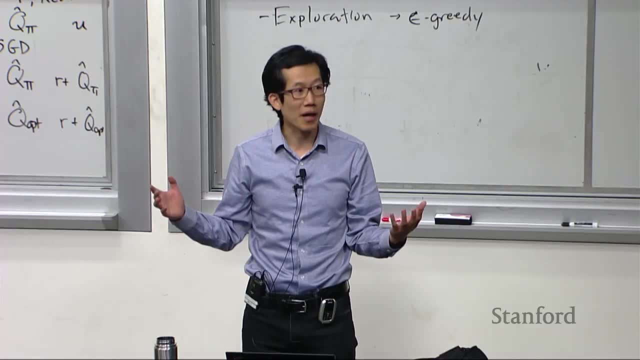 you're never gonna be in the exact same, you know situation, and yet we are- we need to be able to act properly, right? So general problem is that the state space that you you might deal with in a kind of a real world situation is enormous. 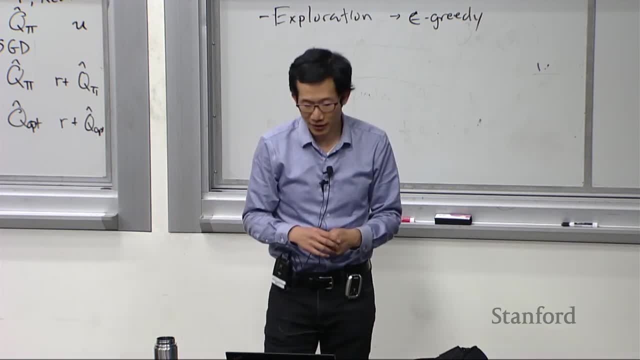 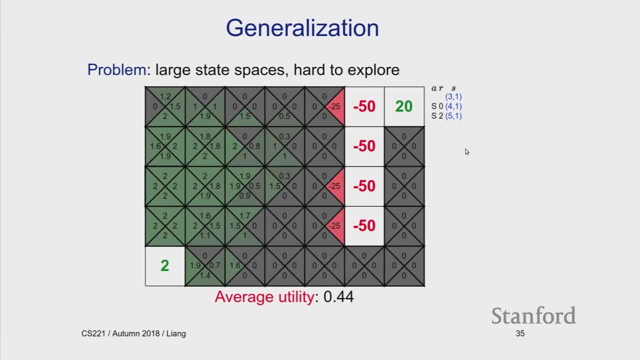 And there's no way you're going to go track down every possible state. Okay, So this state space is actually not that enormous, Um, but this is the biggest state space. I could draw on this- on the screen, Um, and you can see that. this you know. 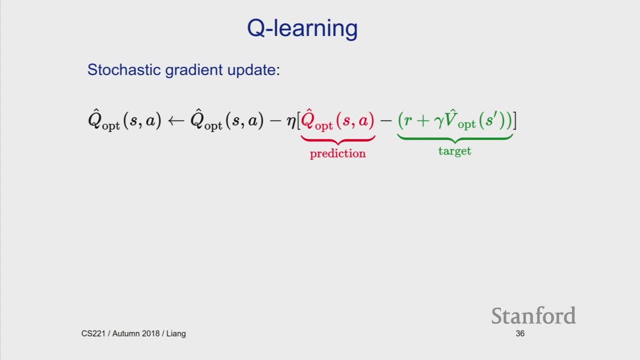 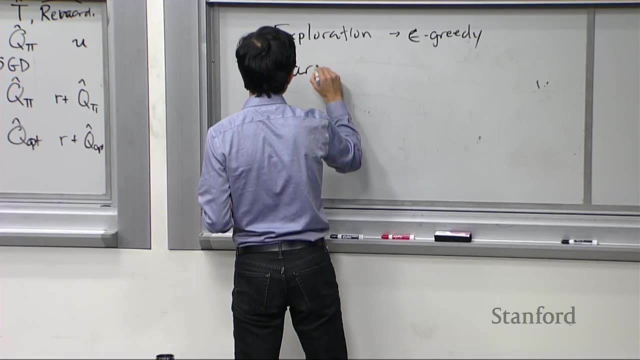 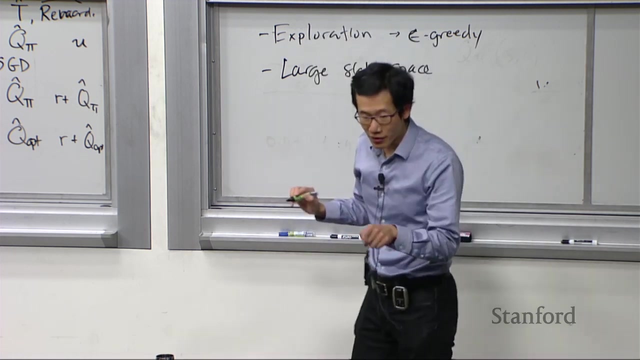 the average utility is, you know, pretty bad here. Okay, So what can we do about this? So, um, I guess let's talk about large state space. So this is the problem. So now, this is where the second-, the third interpretation of model-free Monte Carlo will come in handy. 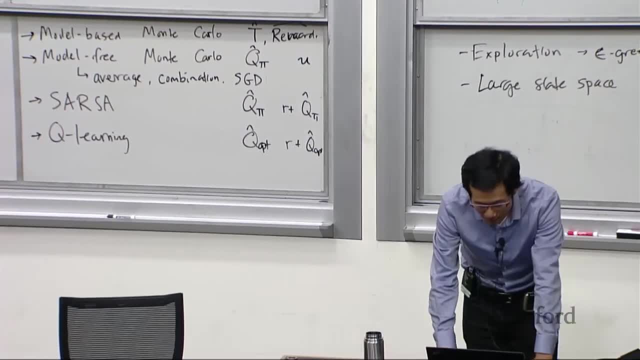 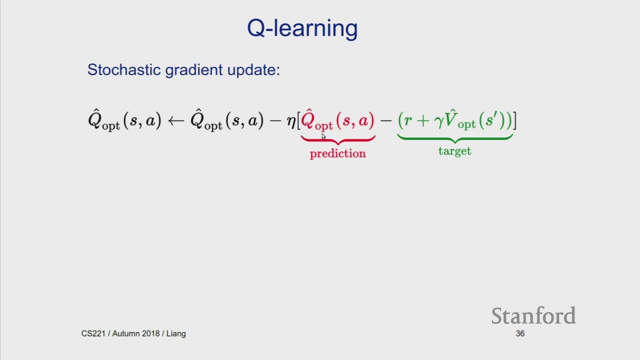 So let's take a look at Q-learning. Okay, So in the context of uh SGD, it looks like this, right? So it's a kind of a gradient step where you take the old value and you minus eta and something that kind of looks like uh. 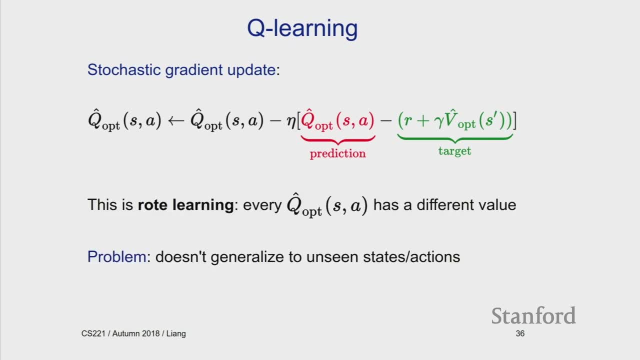 it could be a gradient, which is the residual here. Um, so one thing to note is that, under the the kind of formulations of a Q-learning that I've talked about so far, this is what we call kind of row learning, right? 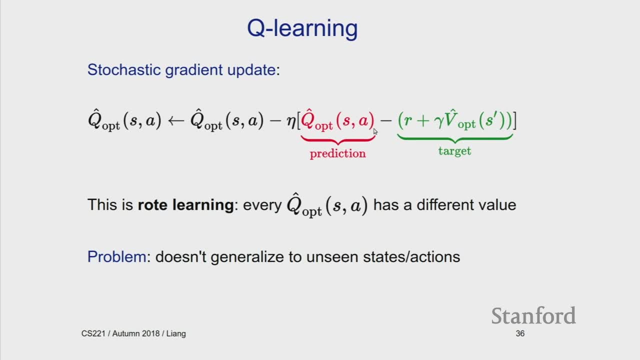 Um, which, if we were, you know Okay. So if we were, you know Okay. So if we were, you know Okay, So if we were, you know two weeks ago, we would have said: this is you know. 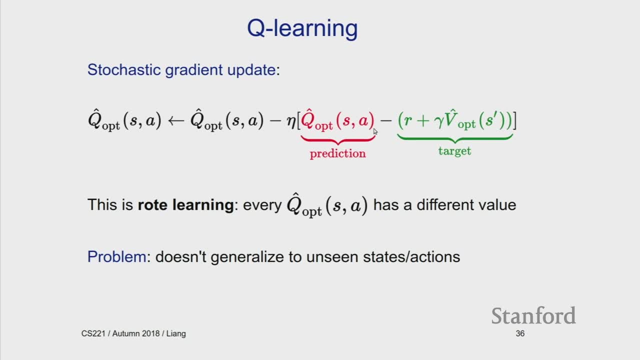 kind of ridiculous, because it's not really learning or generalizing at all. Um, right now it's basically for every single state in action, I have a value. If I have a different state in action, completely different value, I don't, I don't. 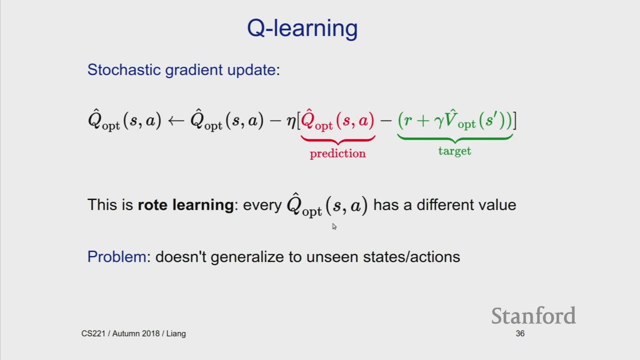 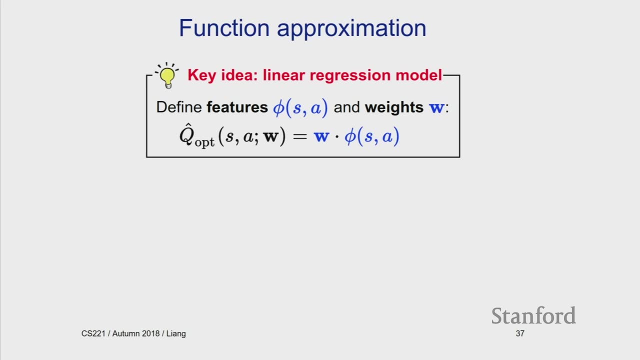 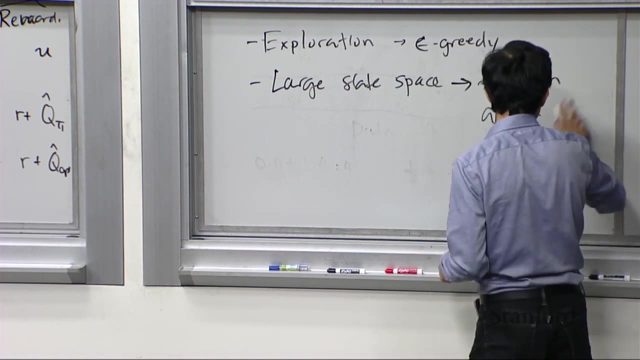 there's no kind of sharing of information And naturally, if I do that, I can't generalize between states and actions. Um, okay, So here's the key idea that will allow us to- um, actually overcome this. So it's called function approximation in the context of reinforcement learning. 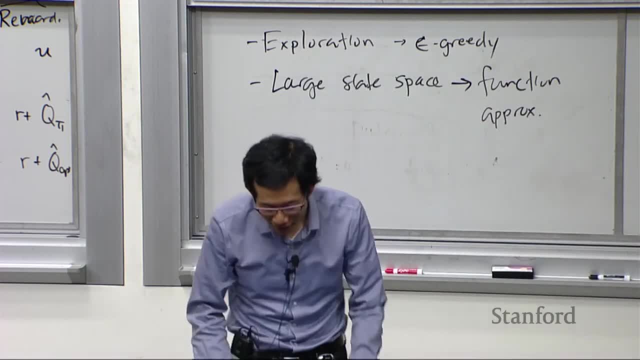 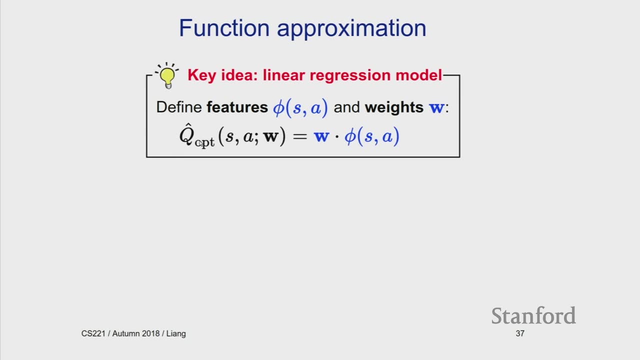 Um in normal machine learning. it's just called normal machine learning, Um. so the way it works is this. Uh, so we're going to define this Qopt SA. It's not going to be a lookup table. It's going to depend on some parameters here. W. 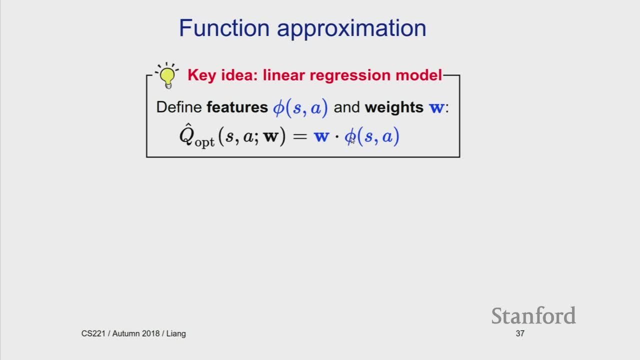 And I'm going to define this function to be W, dot, phi, SA. okay, So I'm going to define this feature vector very similar to how we did it in kind of machine- in the machine learning section, like, except for: instead of SA, we had X. 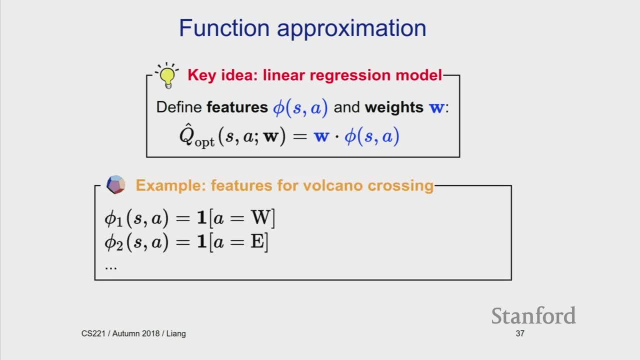 And now the weights are going to be kind of this: you know same. Okay, So what kind of features might you have? Uh, you might have, for example, uh, features on you know actions. So these are indicator features that say: 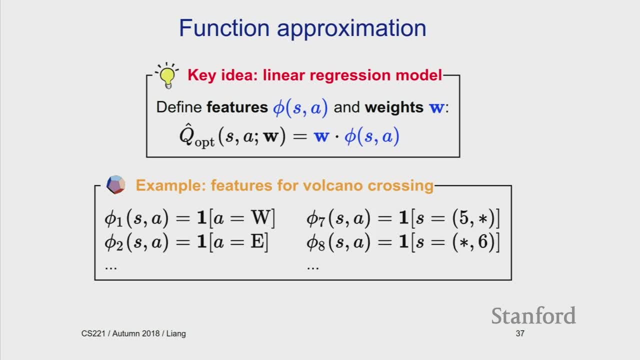 hey, maybe it's better to go east than to go west, or maybe it's better to be in the fifth uh row, or it's it's going to be in the sixth column and you know things like that. So, um, you have a smaller set of features and you try to use that to kind of. 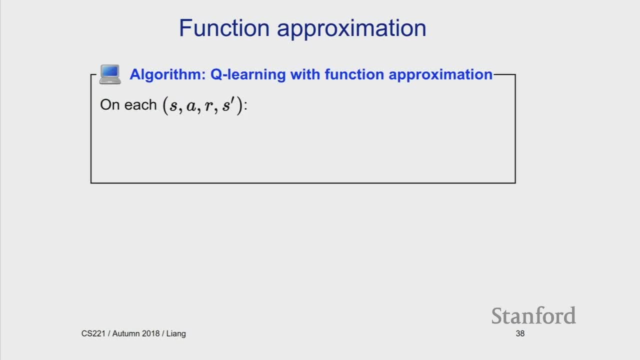 generalize across. you know all the different states that you might see. So what this looks like is now with the features is actually the same as before, except for um. now we have something that really looks like- uh, you know the machine learning lectures. 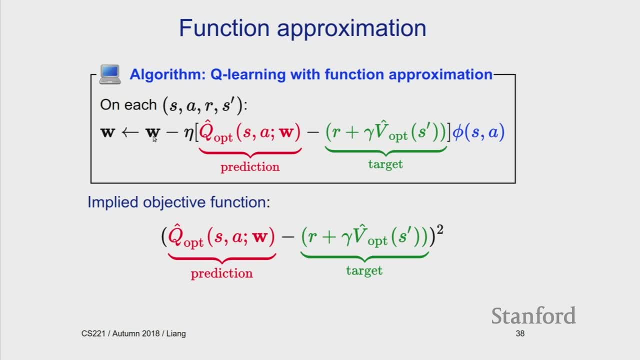 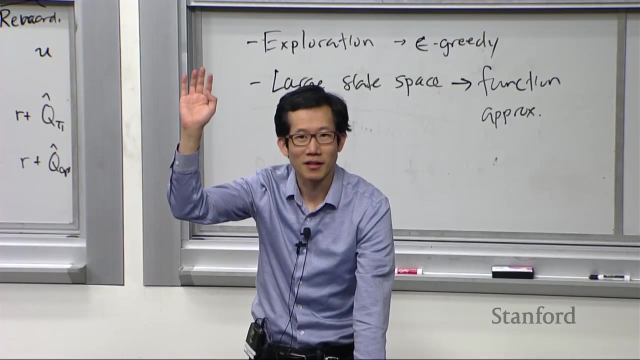 is that you take your weight vector and you do um an update of the residual times, the feature vector. Okay, So how many of you? this looks familiar from linear regression. Okay, All right. So so just to contrast. 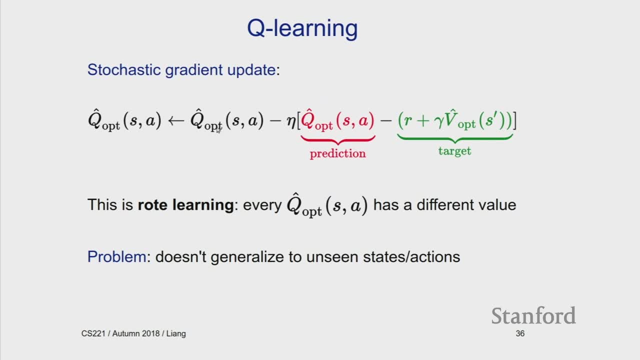 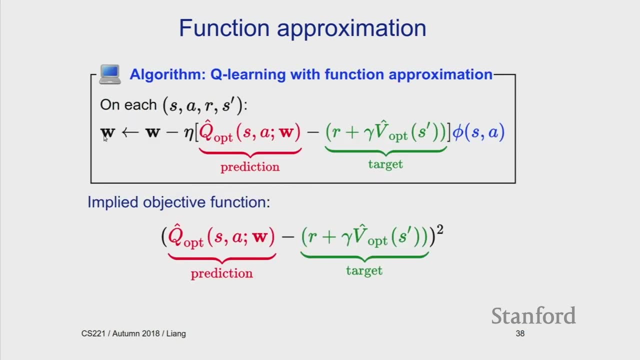 so. so before, we were just updating the Q-opt values, um, but the residual is exactly the same and there's nothing over here. And now what we're doing is we're updating not the Q-vector, um, but the residual is exactly the same and there's nothing over here. And now what we're doing is we're updating, not the Q-vector. 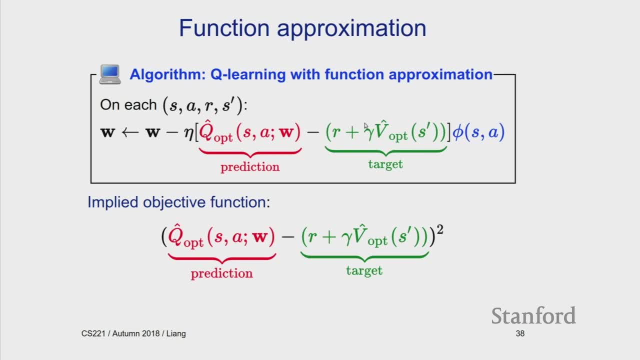 but the residual is exactly the same and there's nothing over here. And now what we're doing is we're updating, not the Q-vector, we're updating the weights. the residual is the same and the thing that connects the, the Q-values, with the 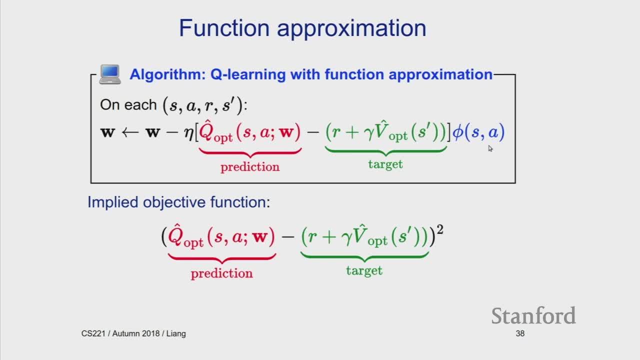 the residual with the weights is the, the kind of the feature vector. Okay, As a sanity check, this has the same dimension. This is a vector. this is a scalar. this is a vector which has the same dimensionality as uh. 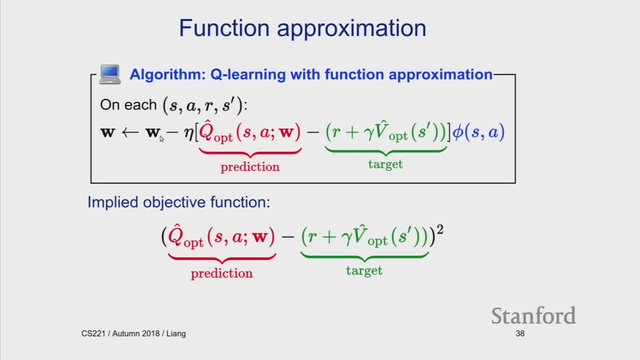 W. Okay, And if you want to derive this um, you can actually think about the implied objective function as, uh, just simply. you know, linear regression. You have a model that's trying to predict a value, um, from an input, um, S-A. 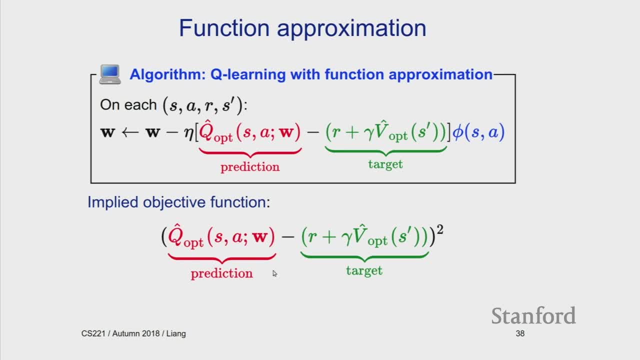 So S-A is like X and Q-opt is like kind of Y, And then you're regre- uh sorry, This target is like, uh, the Y that you're trying to predict, and you're just trying to make this prediction close to the target. 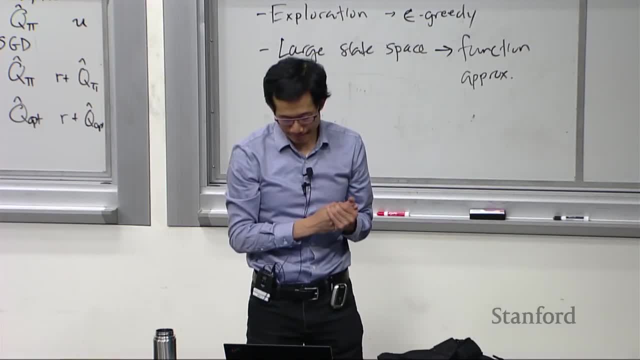 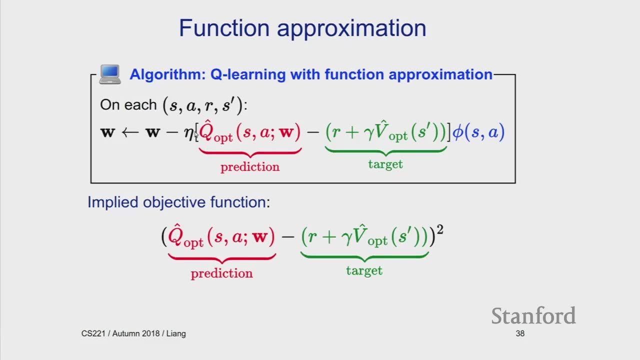 Yeah, Question: Um is the A is the same as A that we had before or now, when we set it like for learning Yeah, So a good question. So what is this A now? Um, is it the same as before or is it new? 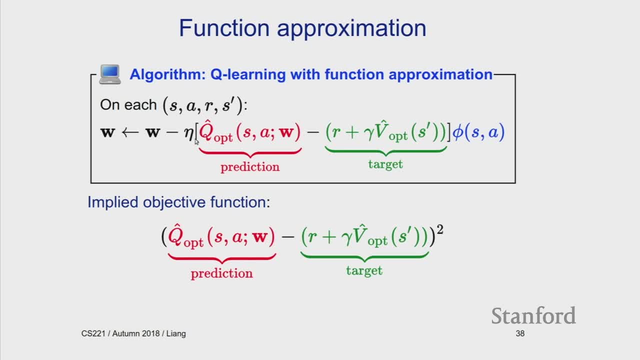 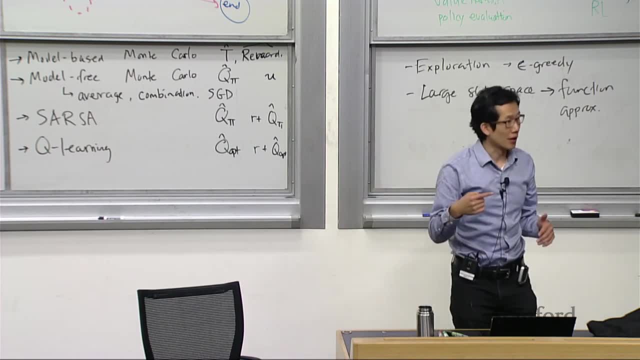 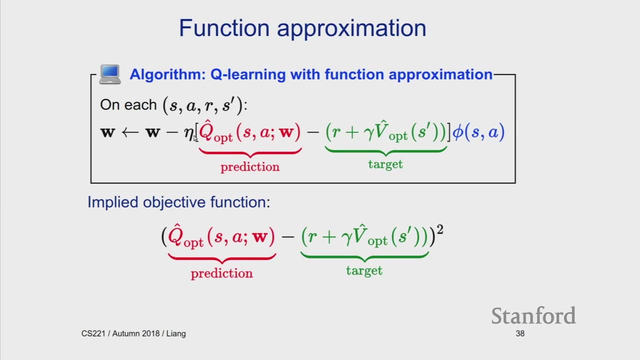 So when we first started talking about these algorithms, right A was supposed to be one over the number of updates and so on. Um, but once you get into the SGD form like this, then now this just behaves as a step size and you can tune it to your heart's content. 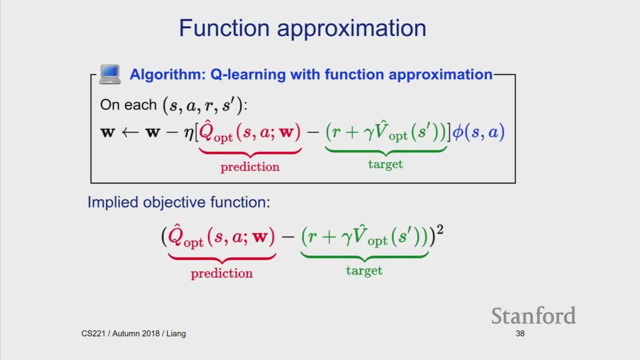 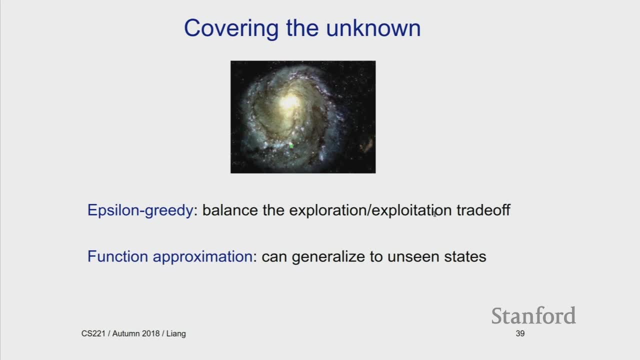 All right. So that's all I'll say about these two challenges. Um, one is: how do you do exploration? Um, you can use Epsilon-Greedy, which allows you to kind of balance exploration with exploitation. Um, and then the second thing is that for large state spaces, 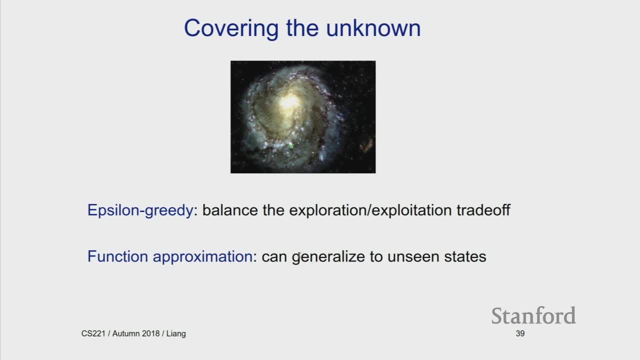 Epsilon-Greedy isn't gonna cut it because you you're not gonna see all the states, even if you try really hard, And you need something like function approximation And to tell you about new states that you fundamentally haven't seen before. 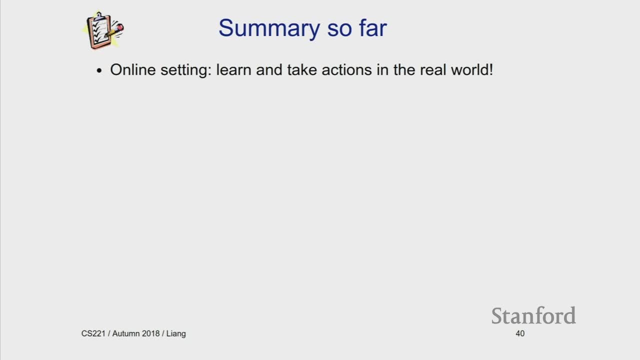 Okay, So summary so far, online learning. we're in the online setting. This is the game of reinforcement learning. You have to learn and take actions in real world. One of the key challenges is this exploration-exploitation trade-off. We saw um four algorithms. 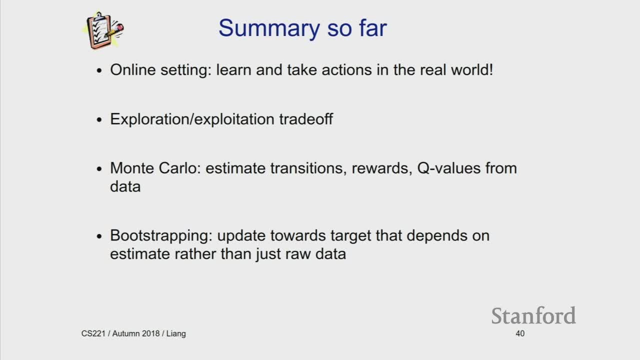 There's kind of two key ideas here. One is Monte Carlo, which is that from data alone, you can basically use averages to estimate quantities that you care about, For example transitions, rewards and Q values. And the second key idea is this bootstrapping, which shows up in SARSA and Q-learning. 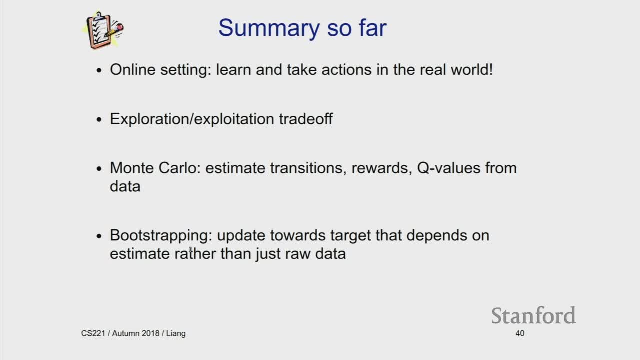 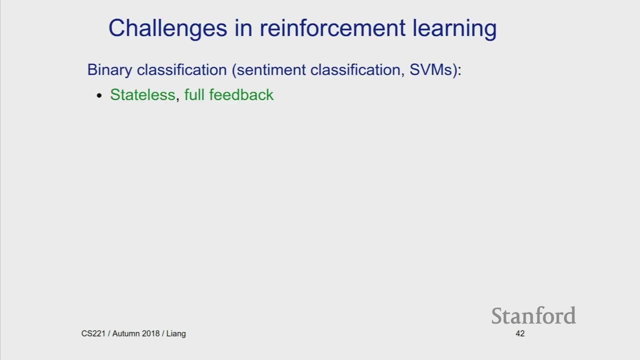 which is that you're updating towards a target that depends on your estimate of what you're trying to predict, Um, not just the, the kind of raw data that you see. Okay, So now I'm gonna maybe step back a little bit and 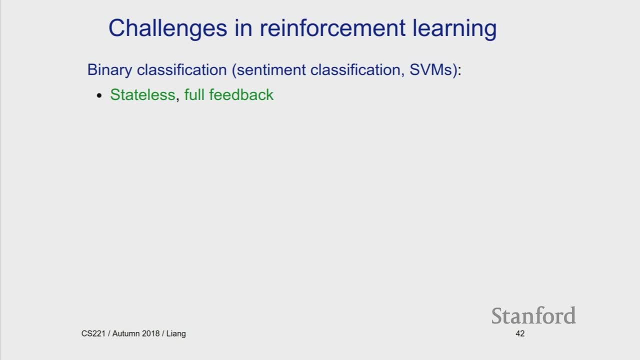 talk about, um, reinforcement learning in the context of some kind of other things. So there's kind of two things that happened when we went from binary classification, which was, you know, two weeks ago, to reinforcement learning now, And it's worth kind of decoupling these two things. 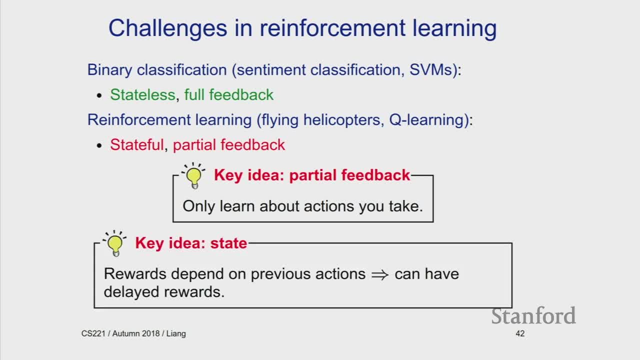 One is state and one is feedback. So, um, the idea about partial feedback is that you can only learn about actions you take, right? I mean, this is kind of obvious in reinforcement learning: If you didn't, don't, don't quit in this game. 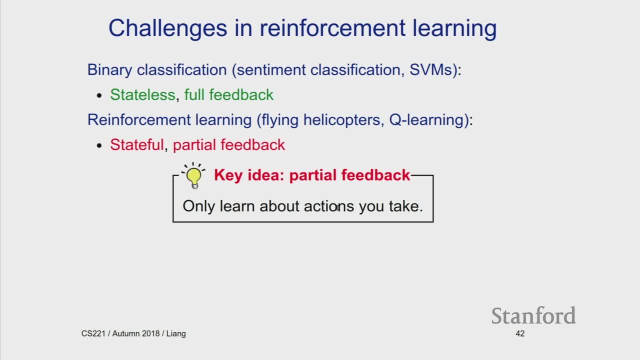 you'll never know how much money you'll you'll you'll get Um. and the other idea is the notion of state, which is that, um, you rewards depend on you know previous actions. So if you're going through a volcano, you have to um. 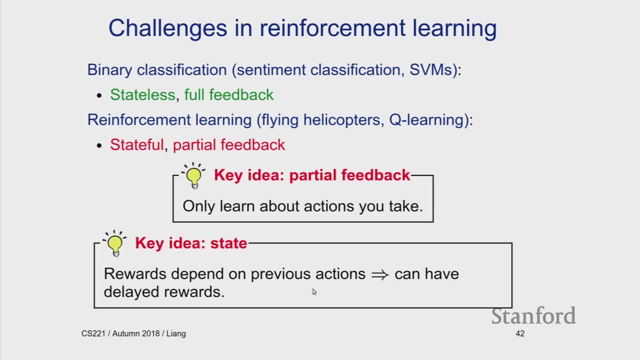 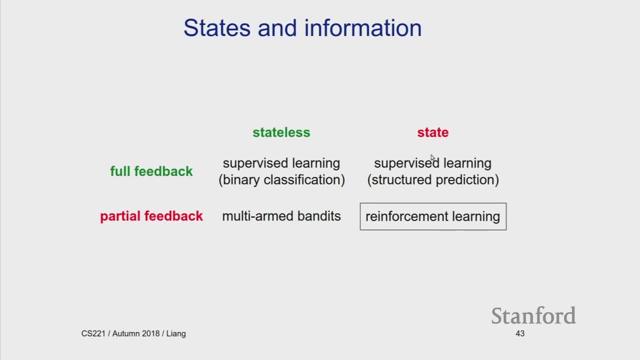 there's a kind of a different situation depending on where you are in in the map, Um, and there's actually kind of so. so this is kind of a you can draw a two-by-two grid where you go from supervised learning. 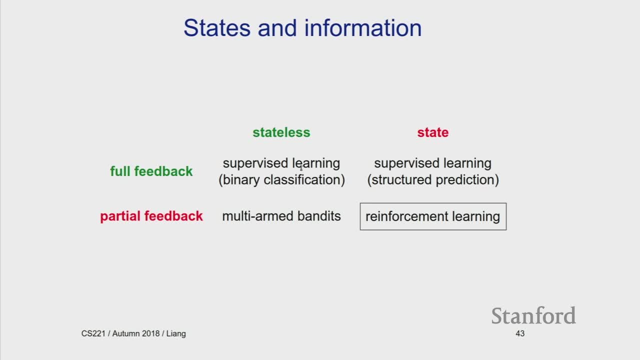 which is stateless and full feedback, right. So there's no state. Every iteration you just get a new example, um, and that doesn't have. you know, there's no dependency in the, in terms of prediction, on the previous examples. 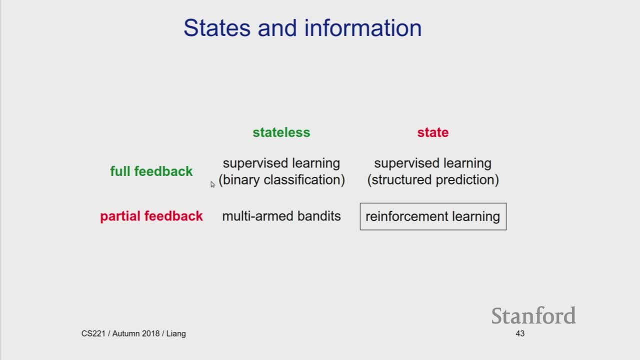 Um and uh, full feedback in, because in supervised learning you're told which is the correct way the label, even though there's, even if there might be, you know, a thousand labels, for example in an image classification, you're just told which one's the correct label. 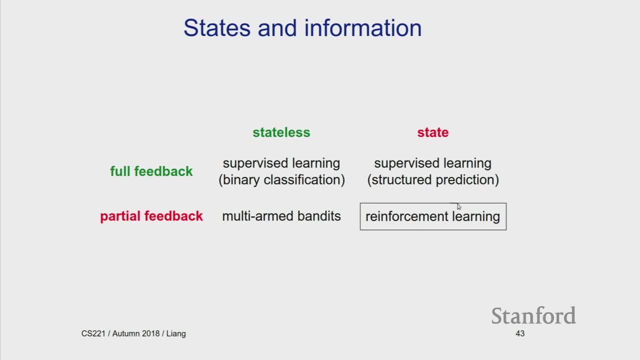 Um, and now in reinforcement learning, both of those are made harder. There's um two other interesting points. So what is called multi-armed bandits is kind of a you can think about as a warm-up to reinforcement learning. 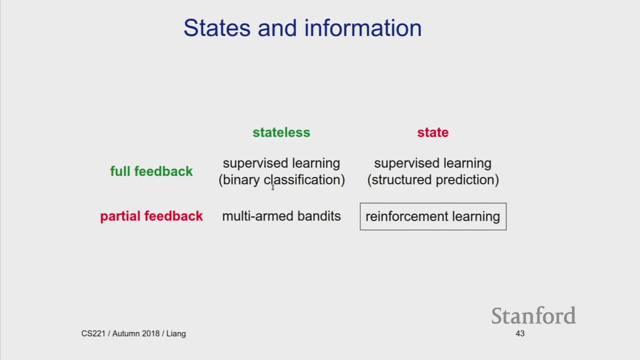 where there's partial feedback but there's no state, which makes it easier. And uh, there's also you can get full feedback, but there's state. So in structure prediction, for example, in machine translation, you're told what the translation output should be. 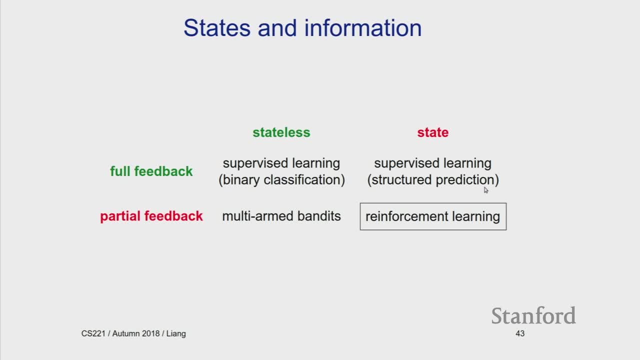 but clearly do uh actions depend on previous actions because, um, you know, you can't just uh translate words in isolation. essentially, Um, okay, So one of the things I'll just mention very briefly is, you know this: uh, deep reinforcement learning has. 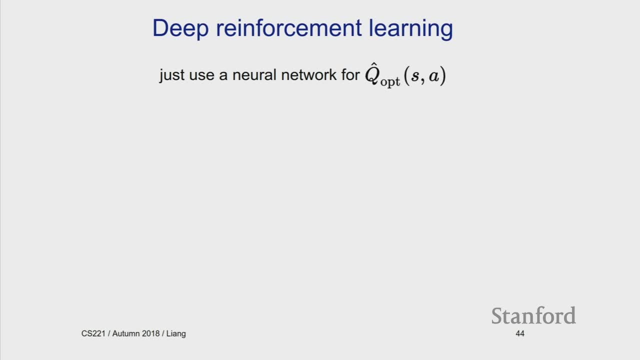 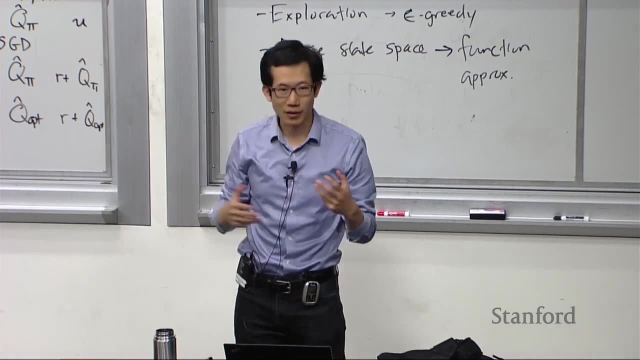 uh been, you know, very popular in recent years. So reinforcement learning: there was kind of a a lot of interest in the, the kind of 90s where a lot of the algorithms were kind of uh, in theory it was kind of developed. 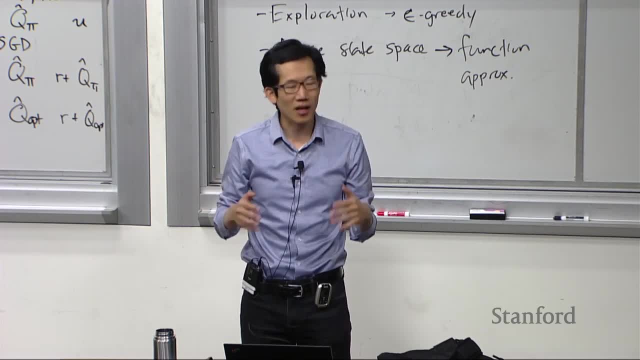 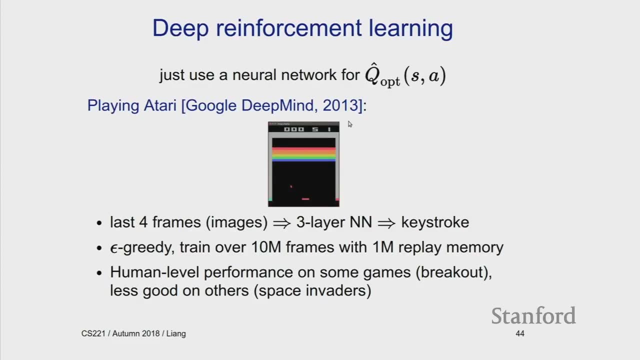 Uh, and then there was a period where kind of not that much, not as much happened. And since um, I guess 2013,- there's been a revival of reinforcement research. A lot of it's due to um, I guess, at the. 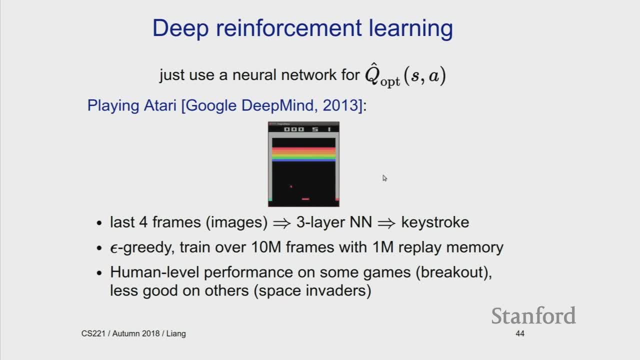 uh, DeepMind, um, where they published a, a paper showing how they can do uh, use raw reinforcement learning to play Atari. So this will be talked about more in the section uh this Friday. Um, but the basic idea of deep reinforcement learning, 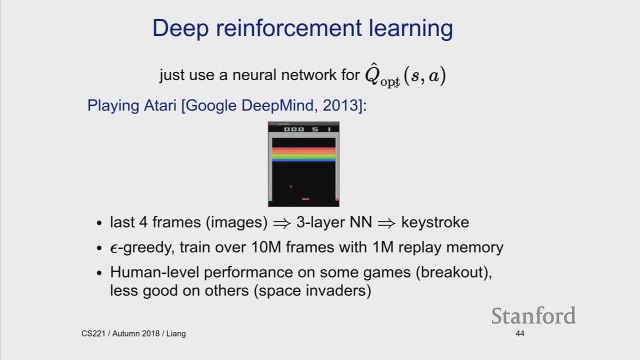 just to kind of demystify things, is that you're using a neural network for QOpt. Essentially, that's um what it is, And there's also a lot of uh tricks um to make this kind of work. 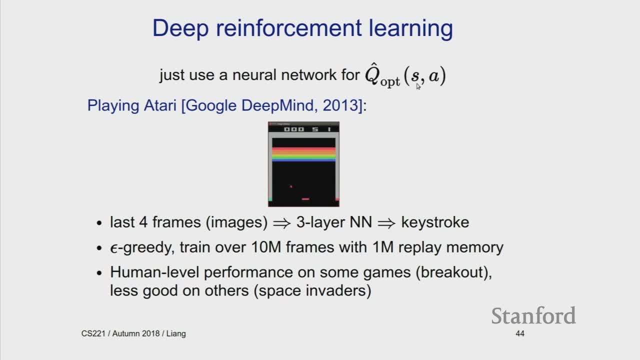 which um are necessary when you're dealing with enormous state spaces. So one of the things that that's different about deep reinforcement learning is that people are much more ambitious about handling problems where the state spaces are kind of enormous. So for this, the state is just the. 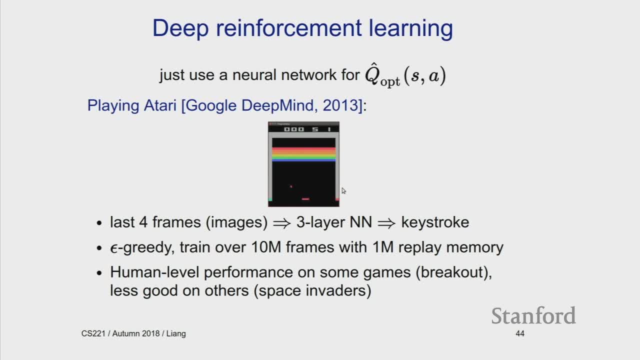 you know the pixels right. So there's, you know, a huge number of pixels, Um and uh, whereas before people were kind of in what is known as a tabular case, which there's, uh, the number of states you can kind of enumerate. 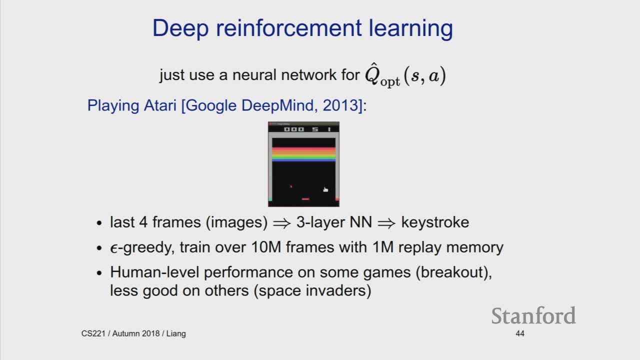 Um, so there's a lot of kind of uh details here. uh, to get right. One general comment is that reinforcement learning is uh tech. is it's really hard right, Because of the uh statefulness and also the delayed feedback. 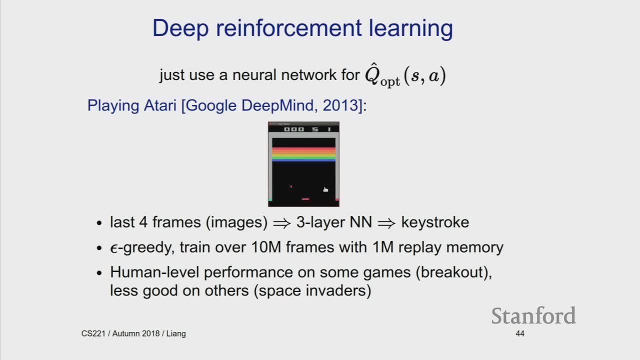 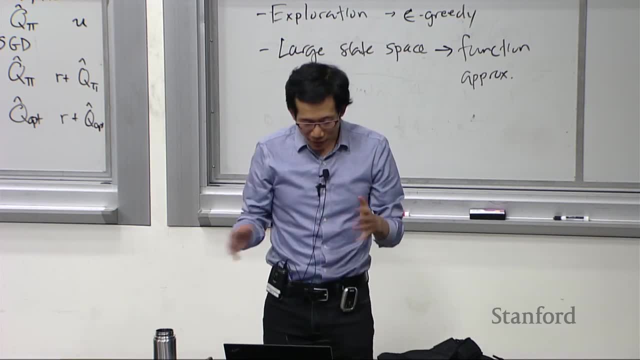 So, just uh, when you're maybe thinking about final projects, I mean, it's a really cool area but you know, don't underestimate how much uh work in compute you need to do. Um, some other things I won't have the time to talk about is. 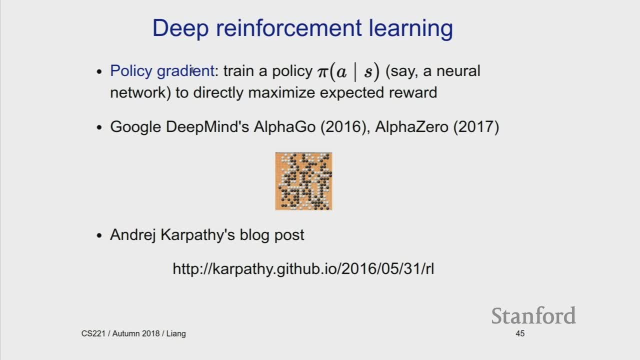 so far we've talked about methods that try to estimate the, the Q function. There's also a way to even do without the Q function and just try to estimate the policy directly. that's called, you know, uh um methods like policy gradient. 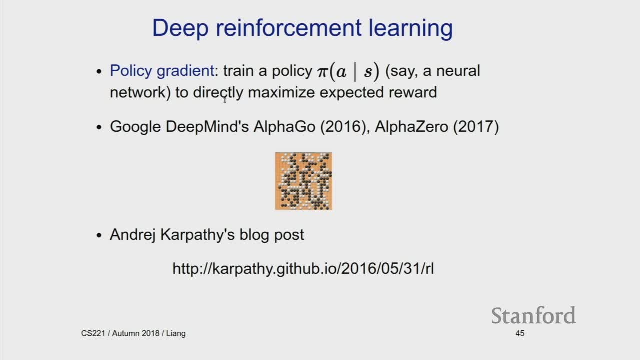 There's also methods like actor critic, that try to combine of these value-based methods and policy-based methods. Uh, these are used in um, uh, DeepMind's, um you know, AlphaGo and AlphaZero, um programs, for you know. 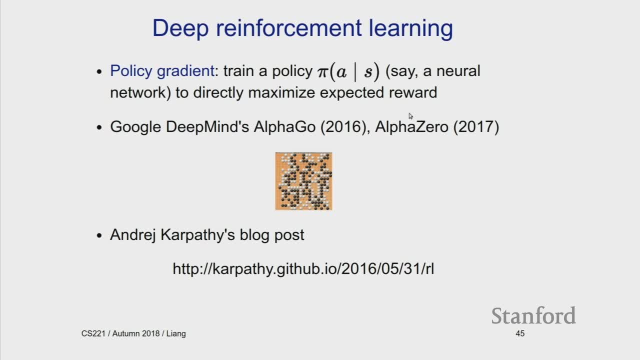 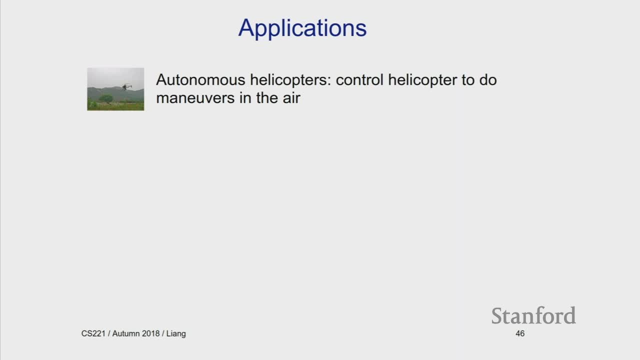 crushing humans like Go. Um, this actually will be deferred to next week's section. uh, because this is, uh in the context of games. Um, there's a bunch of other applications. uh, you know, you can fly helicopters, play backgammon. 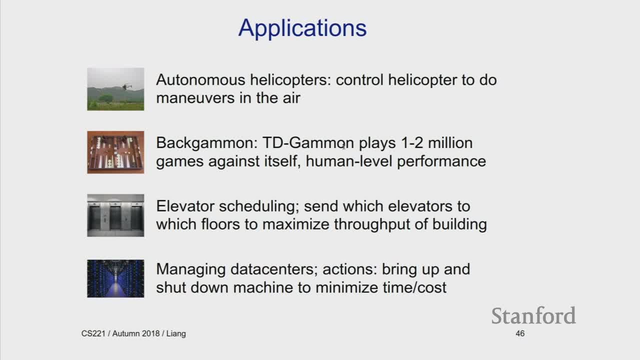 This is actually one of the early examples- TD Gamma was one of the early examples in the early 90s of on, kind of one of the success stories of using reinforcement learning and particular, you know, uh, self-play, Um for non-games, you know.